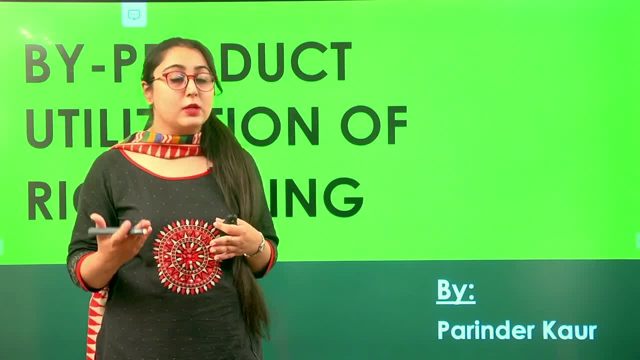 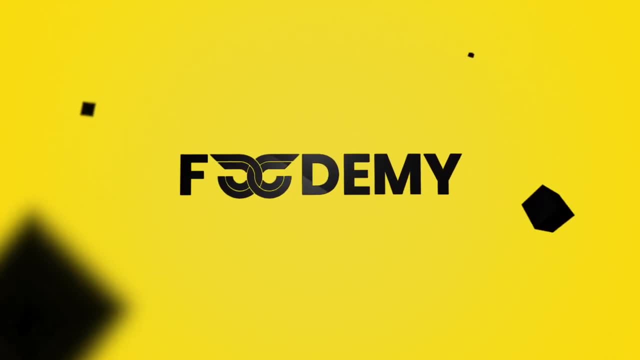 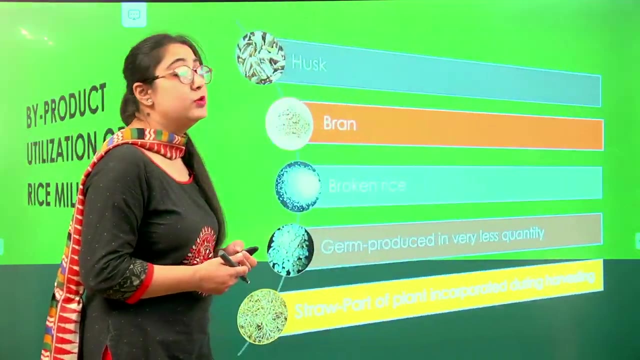 So in today's lecture we will be looking at all the utilizations of the by-products which can be done. So, first of all, if we look at what all products are produced during the rice milling, So there are these main, these five products which are being produced. 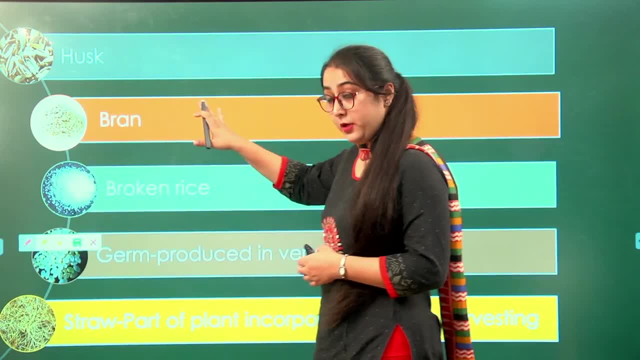 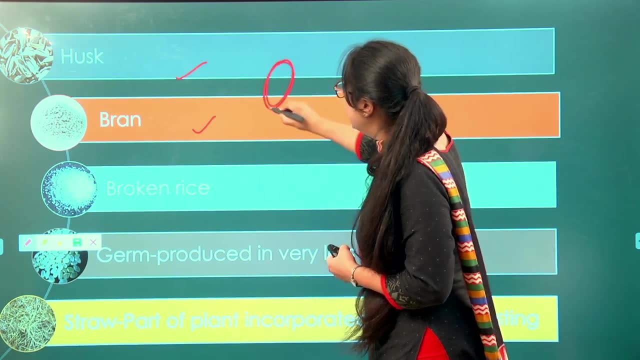 So first one we have is the husk is being produced and then we have the bran. So just to give you a revision, the structure of the rice, the outermost layer, bran, which is removed from brown rice to produce white rice, is being removed. 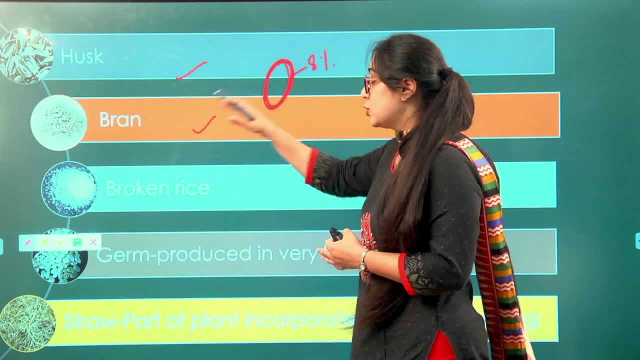 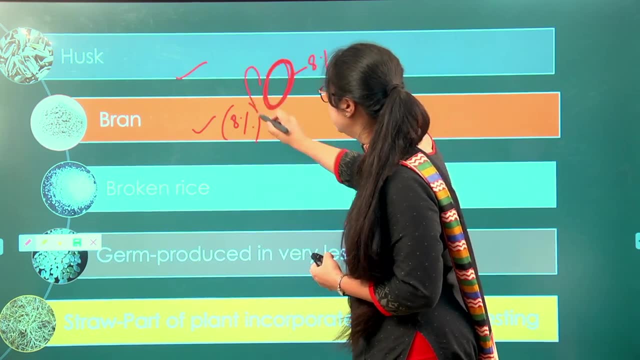 which is around eight percent of the total rice weight. So bran will be present in very high quantity, It will be produced in very high quantity, And then we have the outer covering husk, which is also being removed. That is around 20 percent of the total rice. 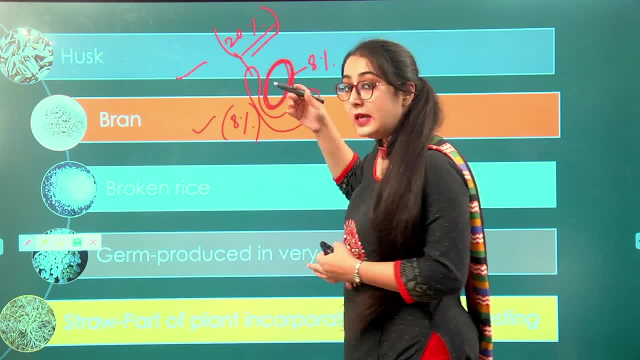 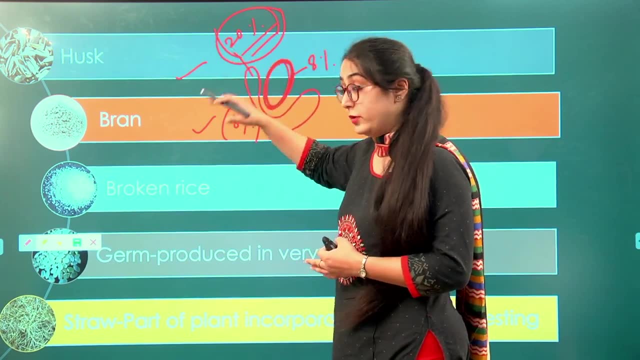 So that is also being removed in order to obtain rice, brown rice or white rice. So again that is 20 percent of the total weight And again it will go waste, which is a large quantity. So this can also be utilized. 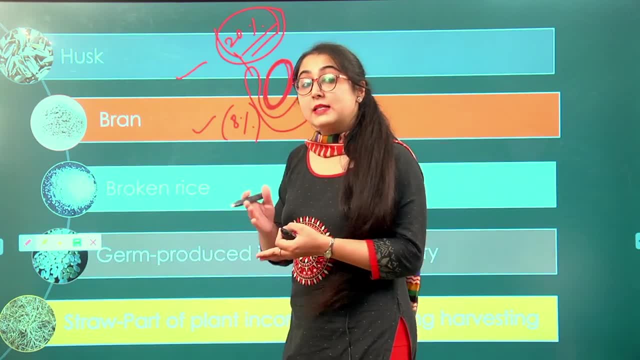 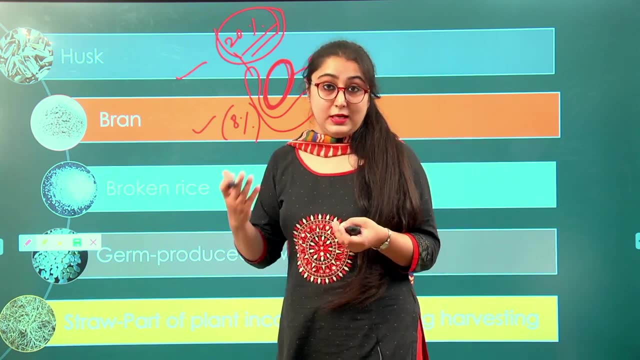 And then we have the broken rice. So already discussed in the milling that during the milling what will happen is that some rice, because of the abrasive and certain frictional forces utilized during milling the rice, can be broken into smaller fragments and many broken rice can be produced. 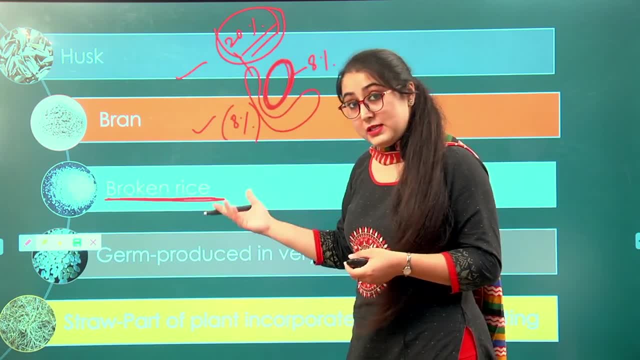 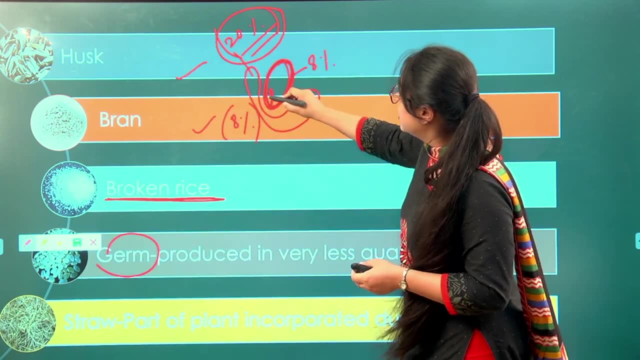 So again, these broken rice need not go waste, They can also be utilized. And then we have germ. So, as we know, in the rice structure around two percent is the germ portion, which consists of the mainly the lipids and the rich in vitamin E. 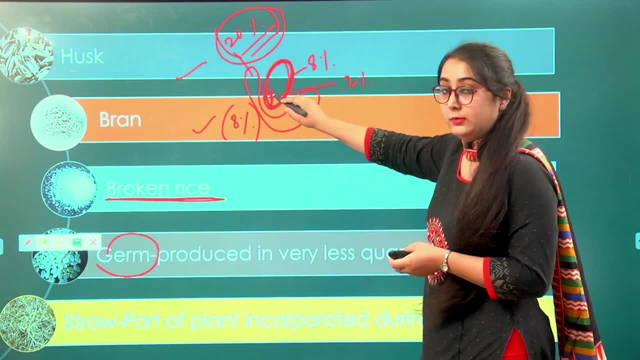 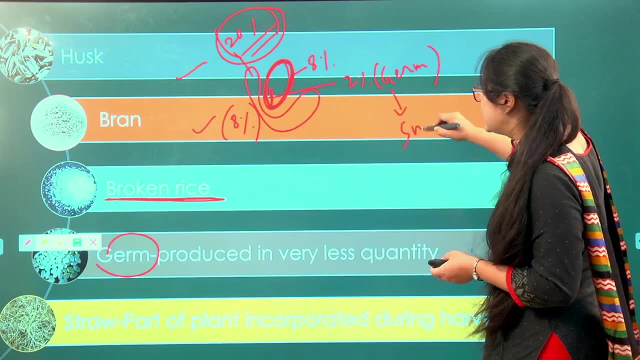 The motive during the rice milling is not to remove the germ, But sometimes what can happen is the germ can also be removed, But however, it will be present in very, very small quantities. So it is not present in such a huge quantity that it can be utilized as a byproduct. 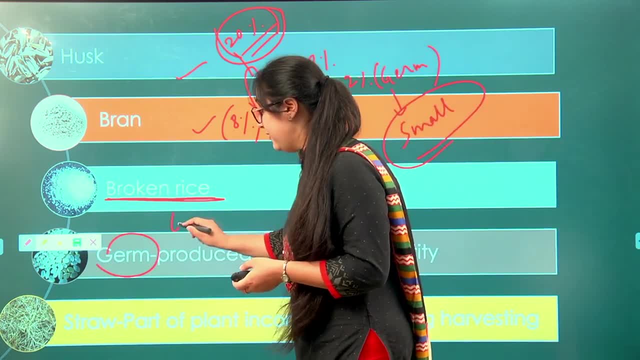 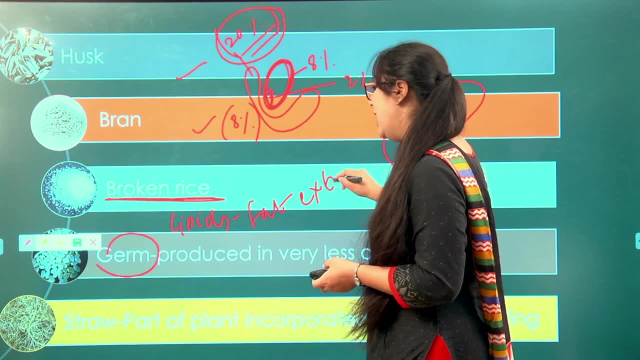 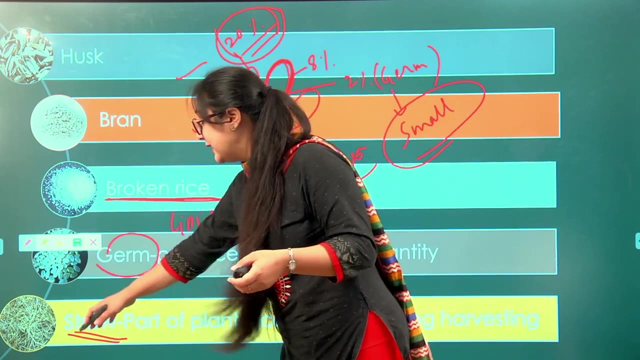 But again, since germ is very, very rich in lipids and fats, germ can sometimes be utilized for fat extraction. If required, or if we have germ in considerable quantity, we can utilize it for the fat extraction. Then we have straw. Straw is basically the part of the plant which is incorporated during the harvesting itself. 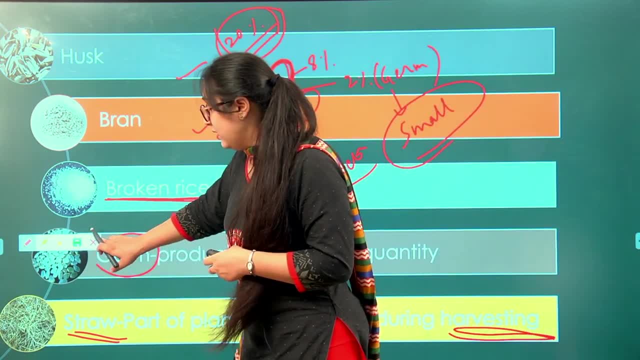 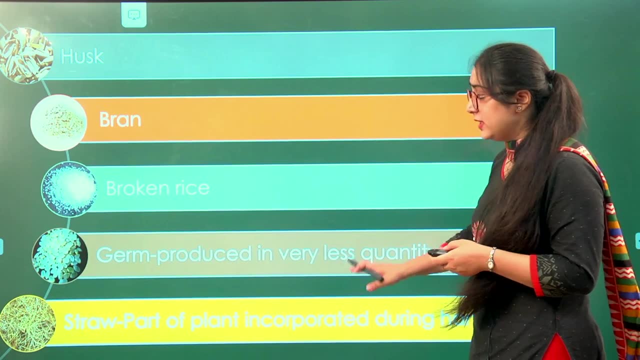 So it can be utilized as a cushioning in the cushions to give it a fluffy kind of a structure. Or sometimes it can be given to animals along with the feed. So these kind of uses straw can be brought to. In today's lecture we are not going to focus on the germ and the straw. 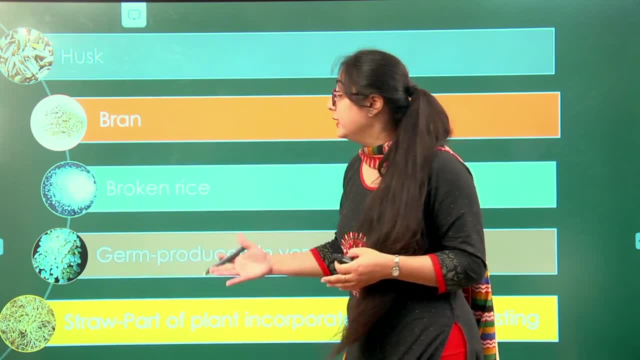 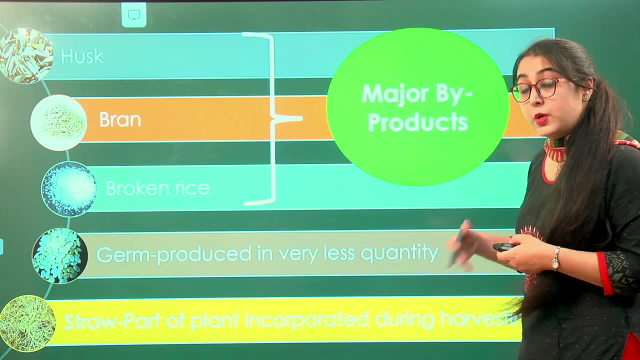 Reason being is they are being produced in very, very tiny quantities. The major byproducts that we are going to focus are the hormones, Husk bran and the broken, since they are the major byproducts which are produced in very, very large quantities. 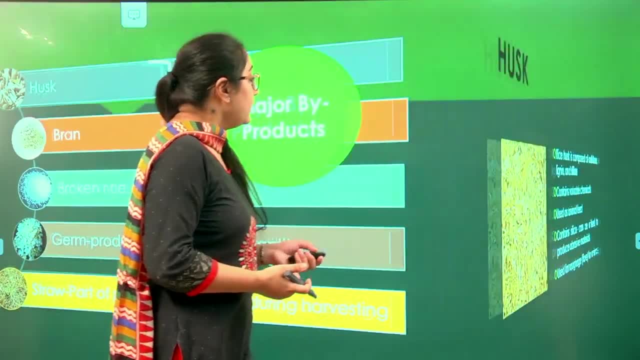 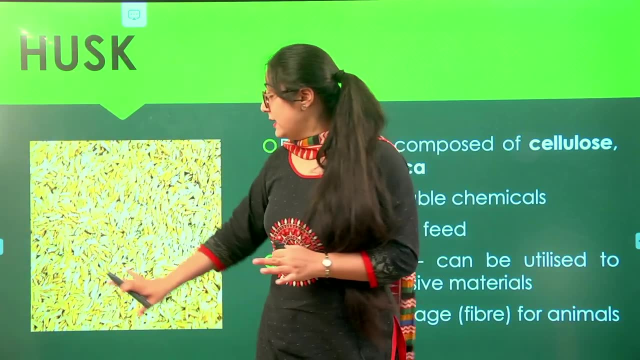 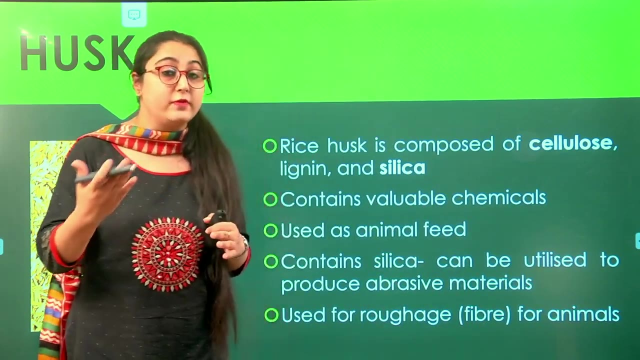 And such high quantities should not be wasted. So now, coming on to the first byproduct, we will be discussing the husk. So, as you know, that husk is the outer covering of the rice, So this husk can be brought to a number of uses, and it is around 20% of the weight. 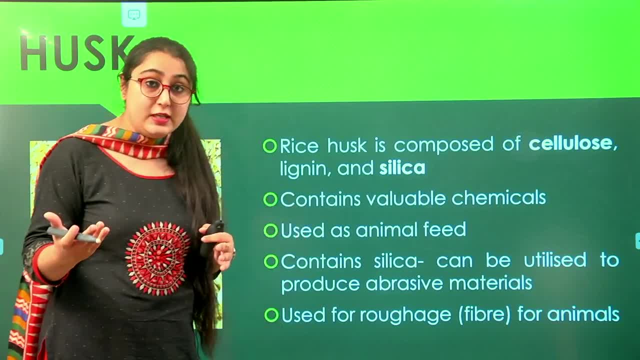 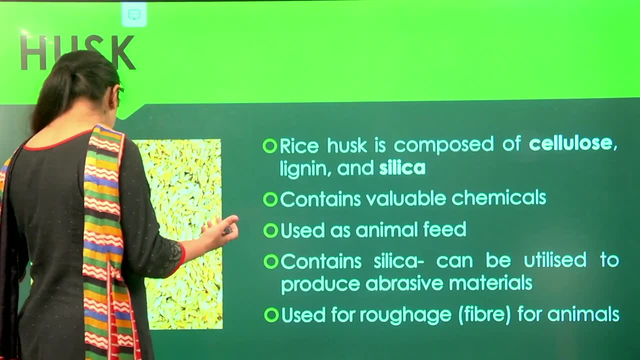 So if you are, if we are processing around 100 kg of rice, we are getting around 20 kg of husk itself. So such a large quantity should not be wasted. It should be brought to some uses, and we have a number of uses in which husk can be put into. 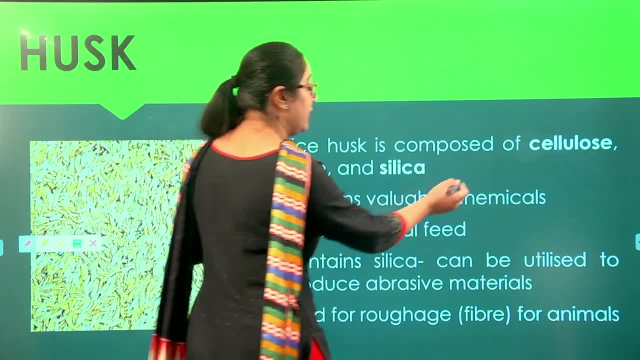 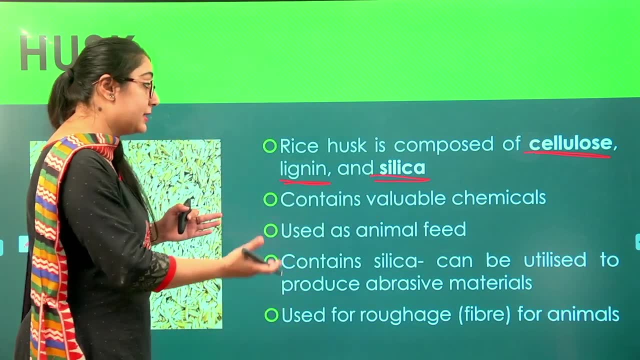 So if you look at the composition of husk, husk is generally made of, it consists of cellulose, lignin and silica. So now, when we say cellulose, lignin and silica, all the uses of husk will be revolving around its composition. 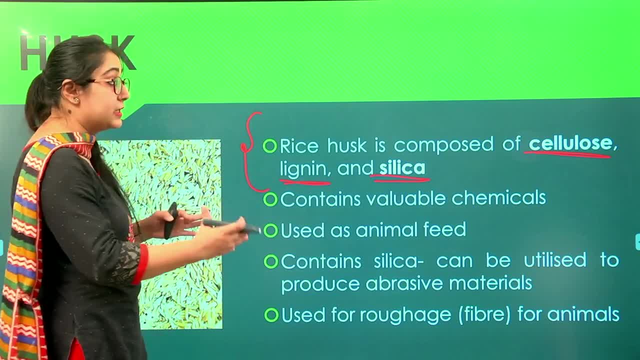 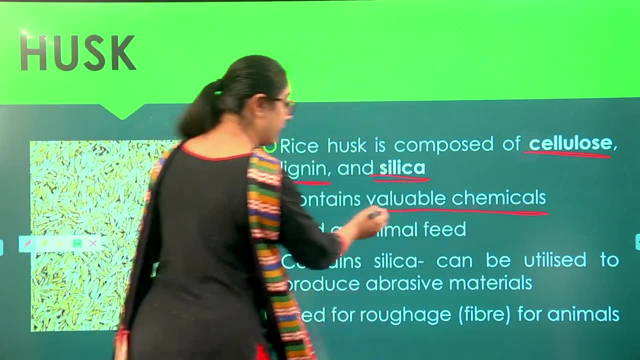 That, because it contains silica, it can be utilized for this purpose. Because it contains cellulose, it can be brought to this use. So we will be looking at all of those. Also, it contains certain valuable chemicals and it can be used as an animal feed. 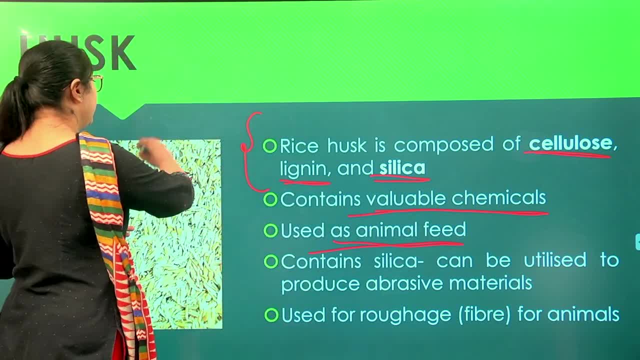 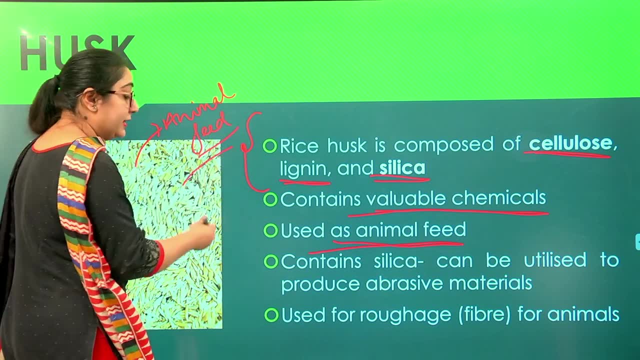 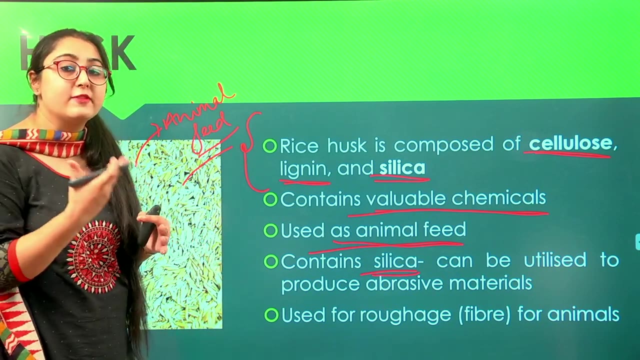 So if we look at the husk, it has very, very good use as an animal feed. It is given to a lot of animals to as a feed or fodder. It can be utilized. Then we have: it contains silica. So since it contains silica, it will be very good to be used as an abrasive material. 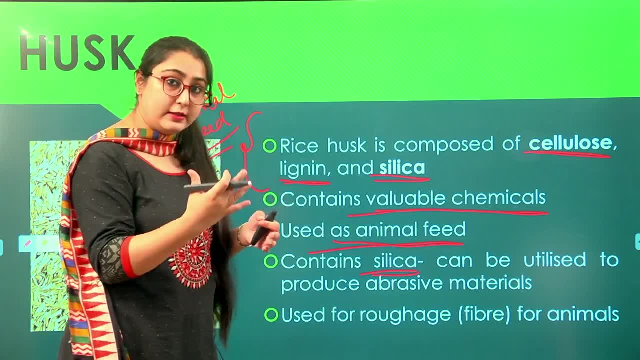 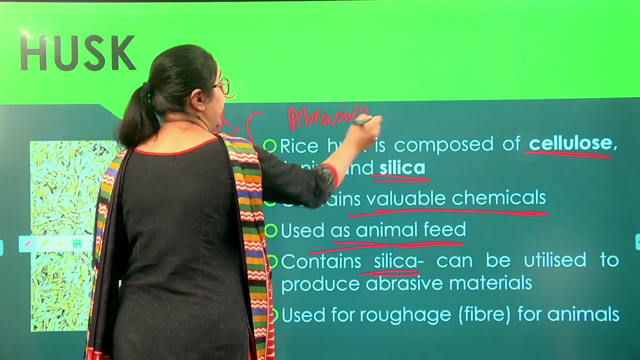 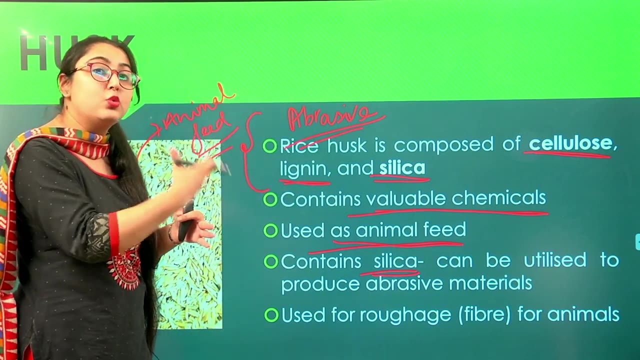 It will give that desired friction or that desired hardness. So it can be brought to a number of uses as an abrasive material. So we can use it, for example, even in the juice extraction. it can be brought to use Because of its abrasive nature. it can be used as an aid to press juice out of the fruits. 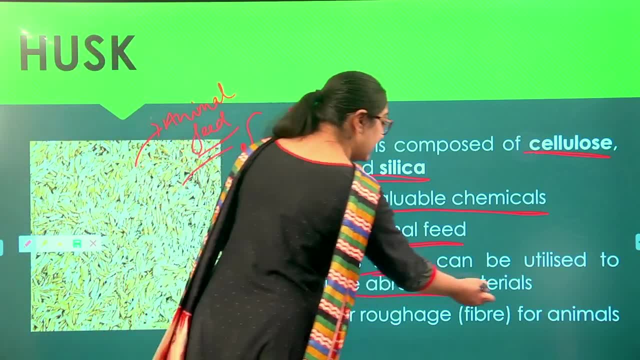 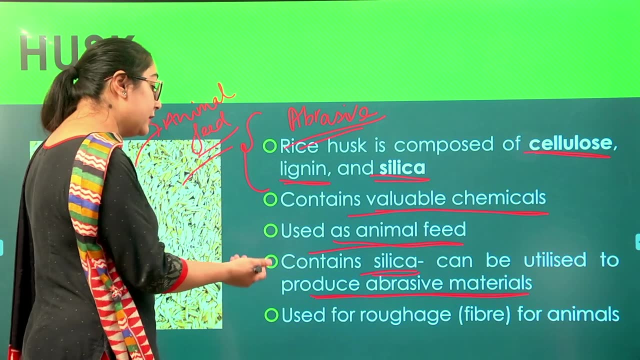 And then it can also be utilized to produce certain other abrasive materials Because of its very, very rough and hard nature due to the presence of silica. Next it contains it can be used for roughage. So the reason it can be used for roughage is that 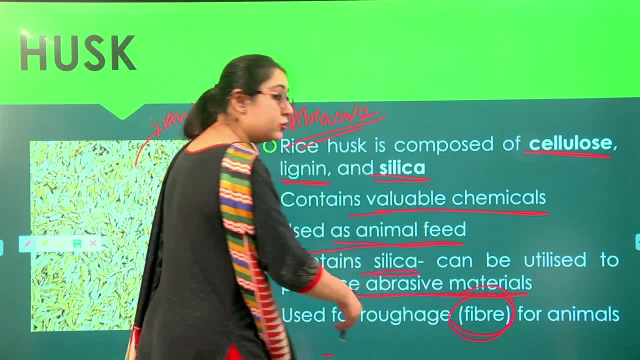 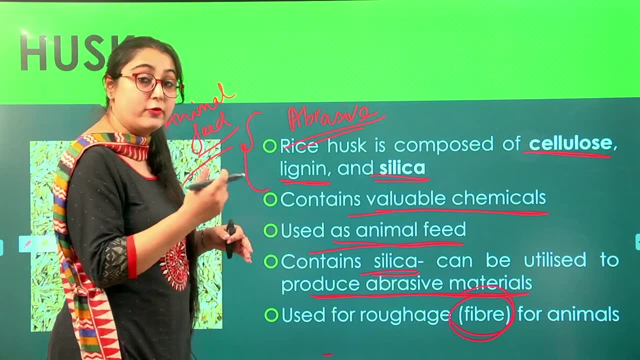 it contains very large amount of fibers. So when we say fibers, we know that fibers aid in feeling of fullness And are very, very good for health as a source of roughage. So for utilizing it as an animal feed, it becomes even more valuable now. 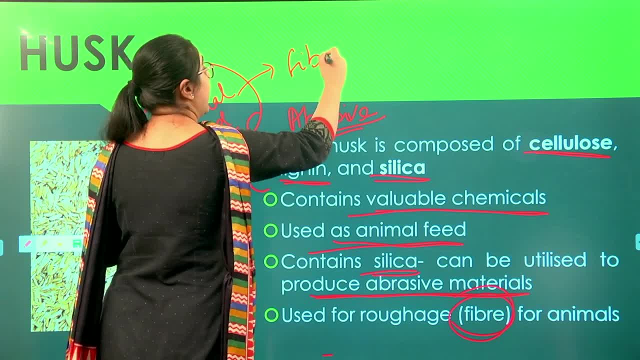 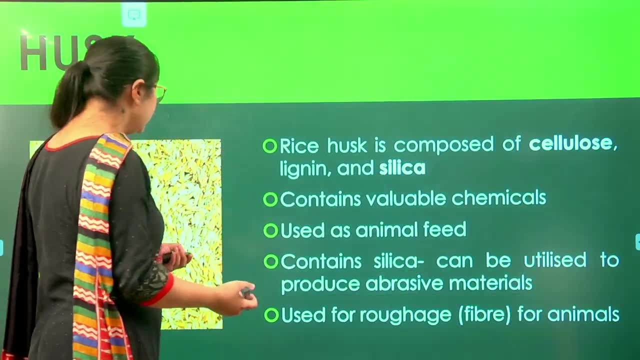 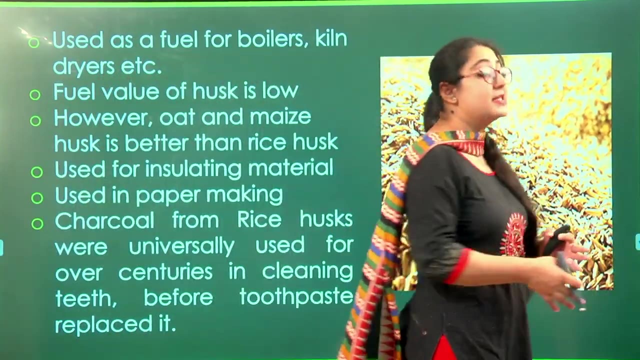 Because it is very, very good source of fiber And it can help add a filling kind of a feeling if added to the animal foods. So then, looking at some more uses of husk That we have over here, Is that even husk finds a use in fuel for boilers, kiln dryers and all of these. 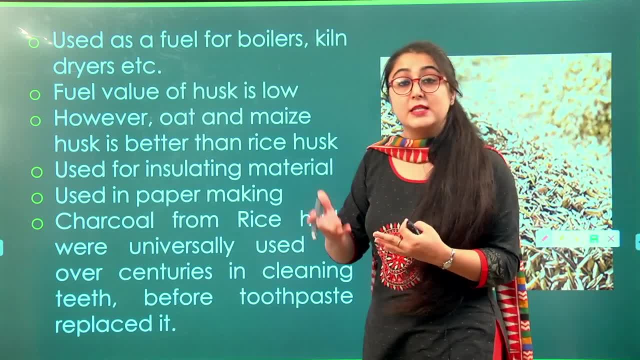 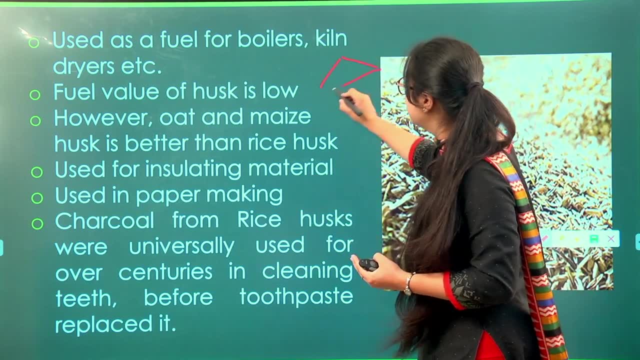 So it is generally born to produce energy. Fuel utilization is done from husk And kiln dryers. it has been basically used. So kiln dryers- if we basically look at what kiln dryers are, They are the most primitive kind of dryers which look something like this: 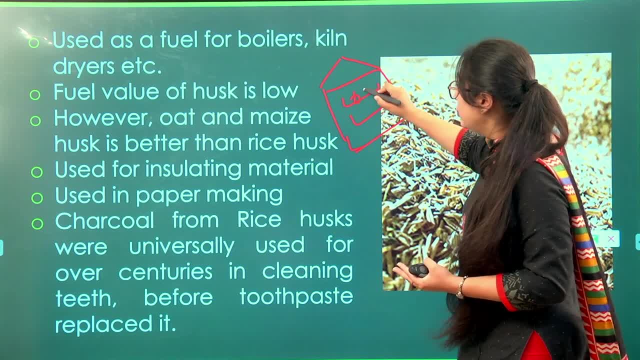 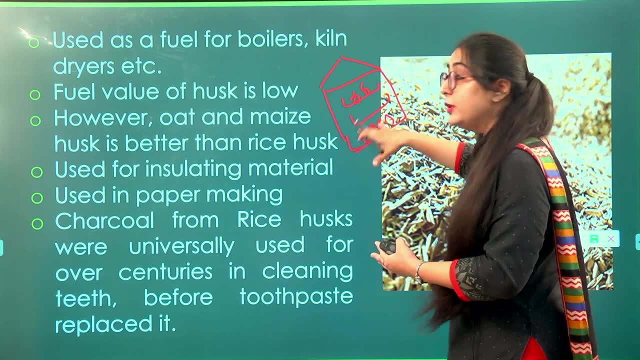 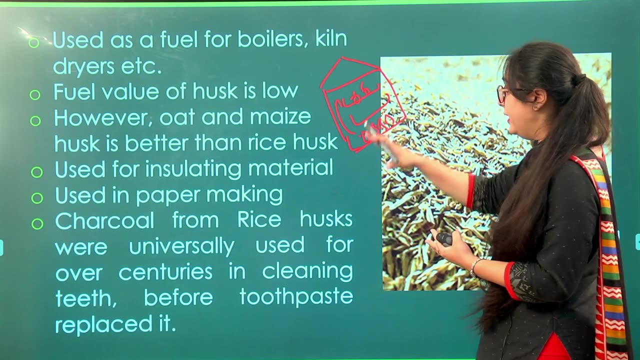 So we have trays on which the food is kept here to dry. The food is kept And from here we are burning some kind of fuel. So here we are burning and producing energy to dry this kind of fruits and vegetables Or certain other food products in this kind of a dryer and kiln type of a dryer. 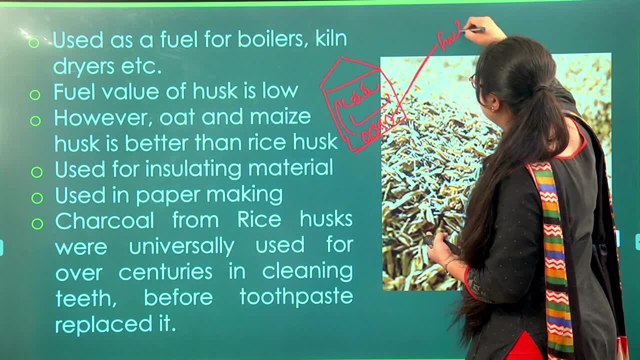 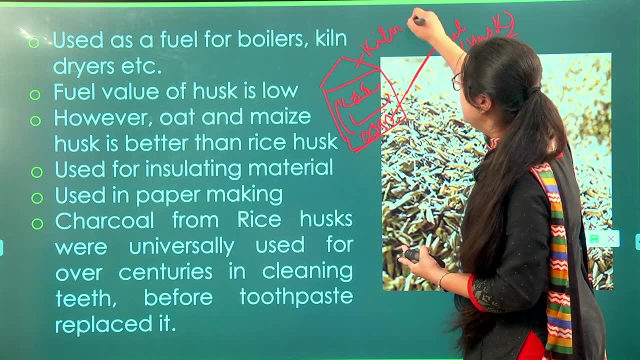 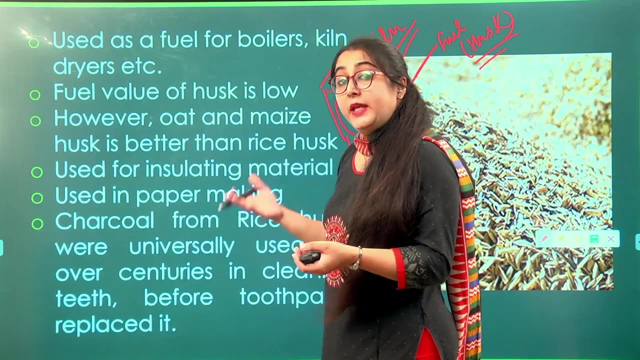 And a source of this fuel can be. this fuel can also be husk, So it has been used in a large quantity in these kiln dryers, As well as in certain other boilers, to produce energy, heat energy for various purposes And, however, even though it is used as a- you know, as a fuel very much. 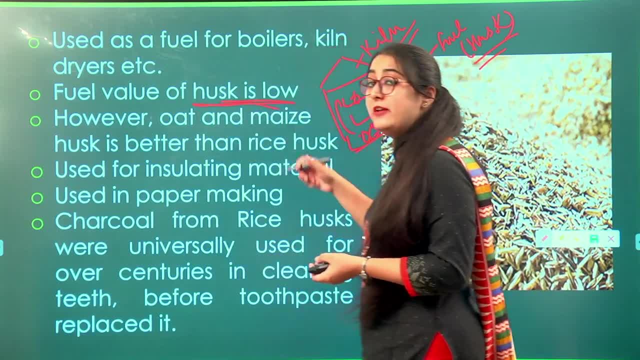 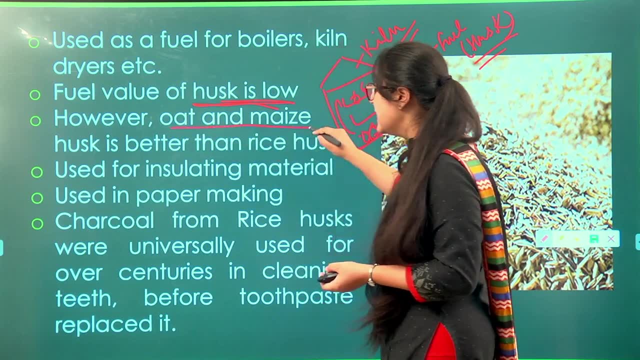 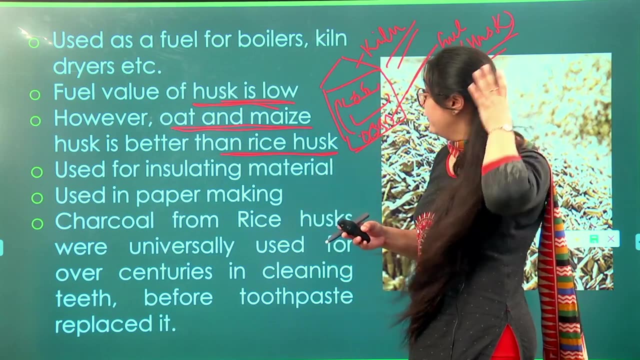 But the fuel value of this husk is low, Especially if we compare to husk being obtained from certain other food products, For example oat and maize. They have husk which give better fuel value than the rice husk. Still, rice husk has a finds a lot of uses. 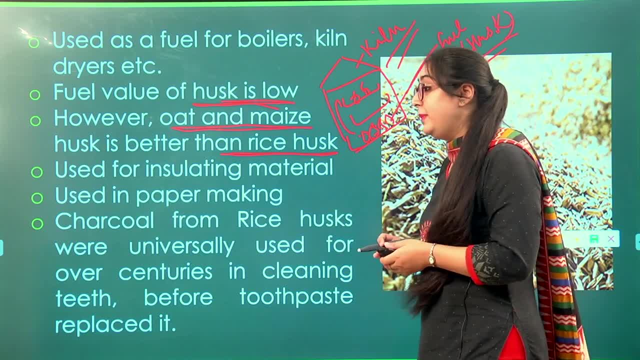 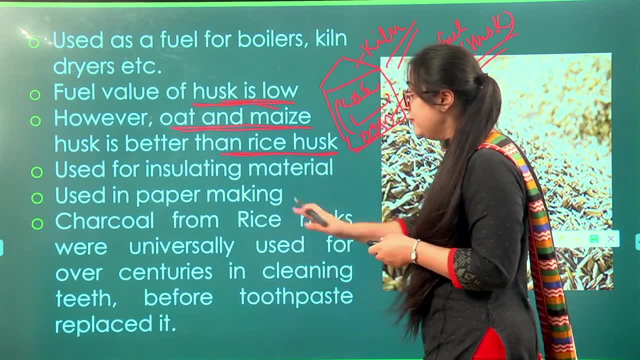 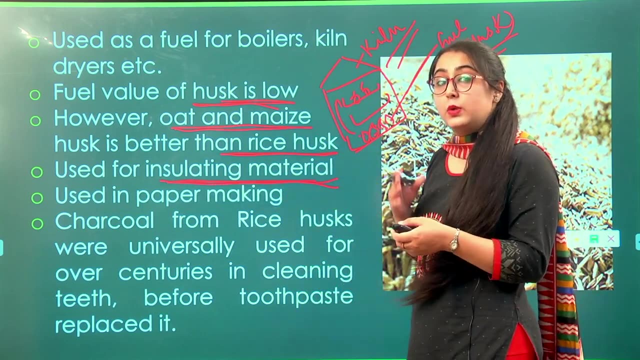 And even what can happen is that the rice husk can be put into use by As a good fuel source by modifying it somewhat, So we will be looking at that later. It is used for insulating material also, So what husk can also be used as an insulating material? 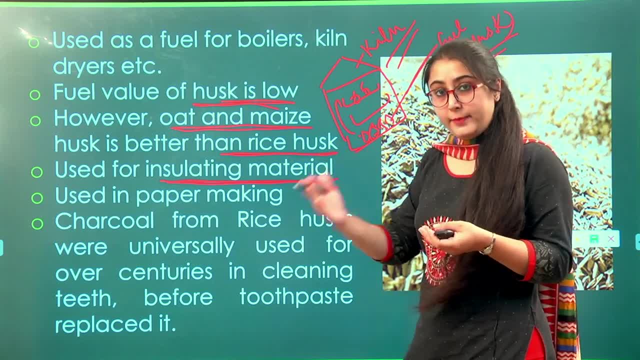 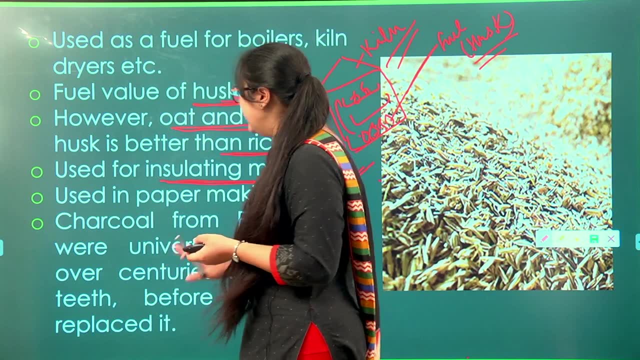 Since it helps to block the air coming And hence it has a very good use as an insulating material as well. And then it is used in paper making. So the reason husk is being used in paper making is that, If we notice, in the beginning itself we discussed 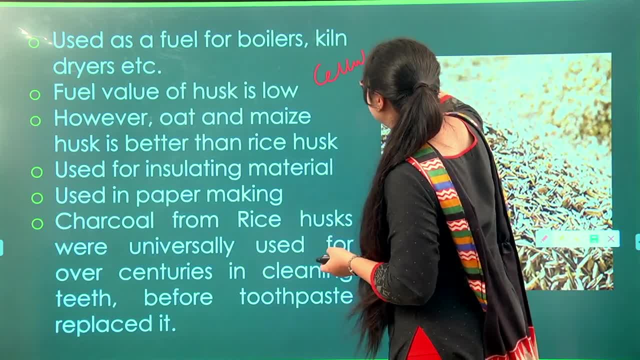 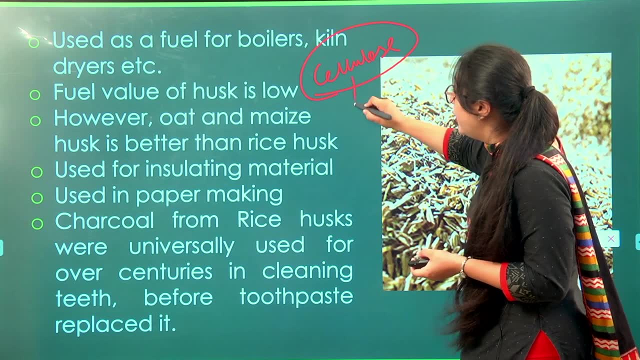 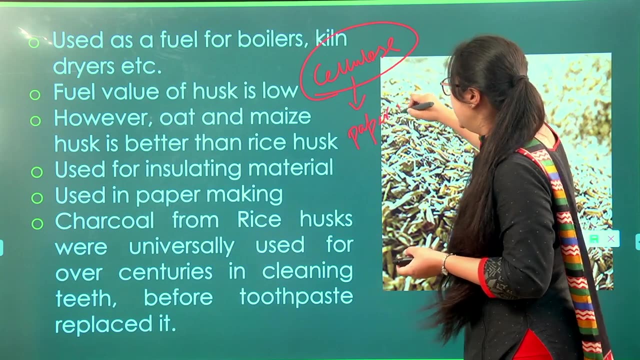 That husk contains cellulose. So once it contains cellulose- See, cellulose is the main component Which is responsible for forming of paper. So since husk contains cellulose, It can also be brought to use as a paper making. It can be brought to use in paper making. 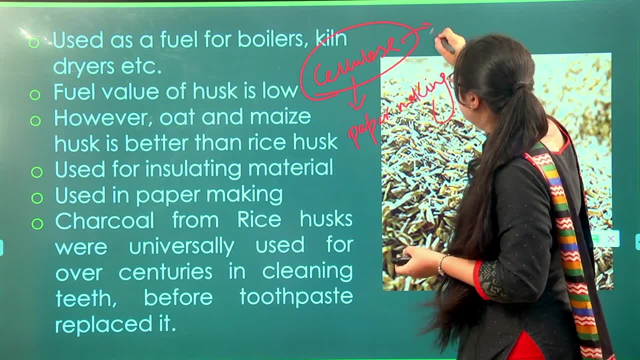 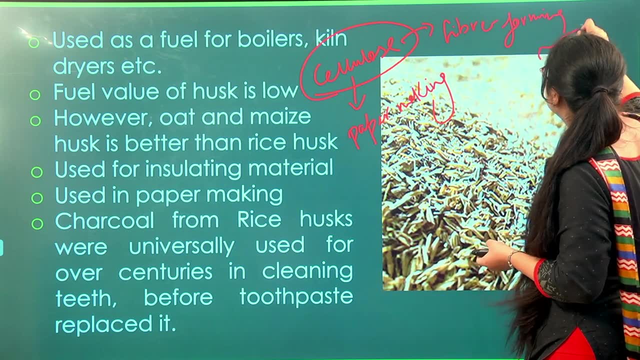 And cellulose is the main component in the paper, Which gives the fiber forming ability. So, because of its fiber forming ability of the cellulose, The cellulose forms a structure And it is able to make the desired texture required in case of a paper. 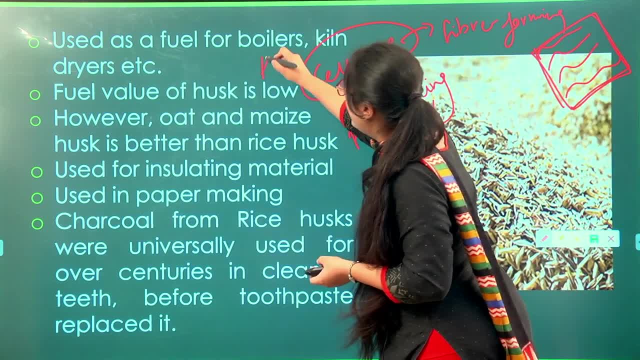 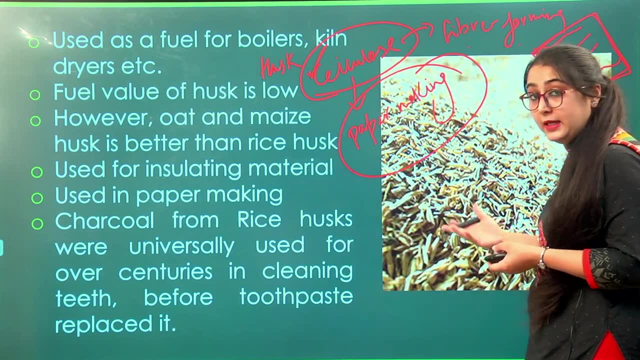 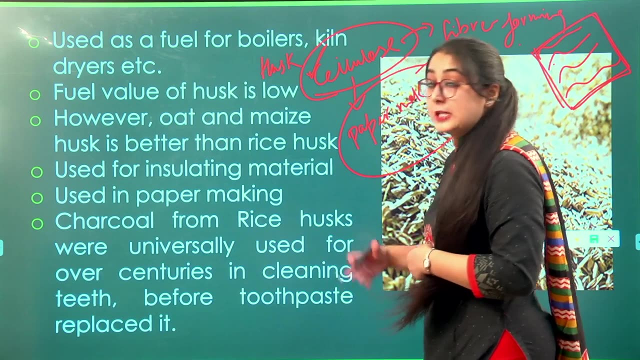 So since husk- again Now husk- contains cellulose, It will have the same fiber forming properties And it can also be brought to use in the paper making industry. So the paper making industry also utilizes husk, And then charcoal from the husk has been used universally. 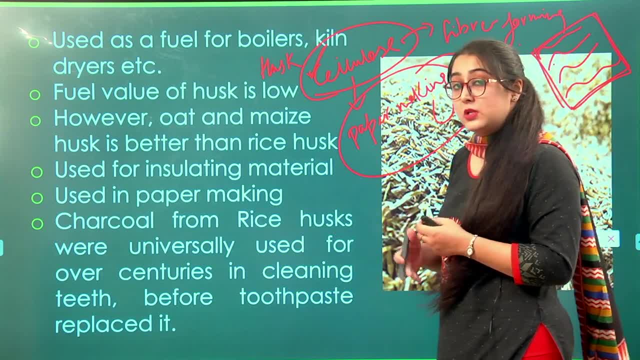 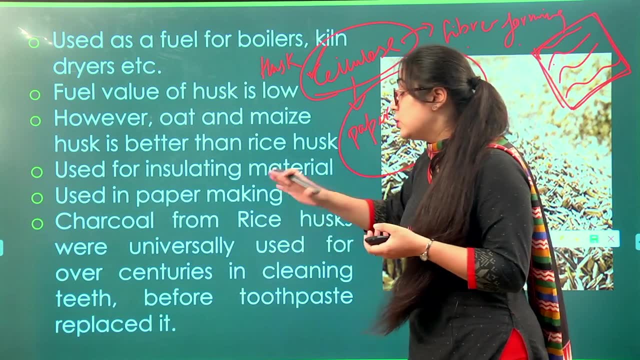 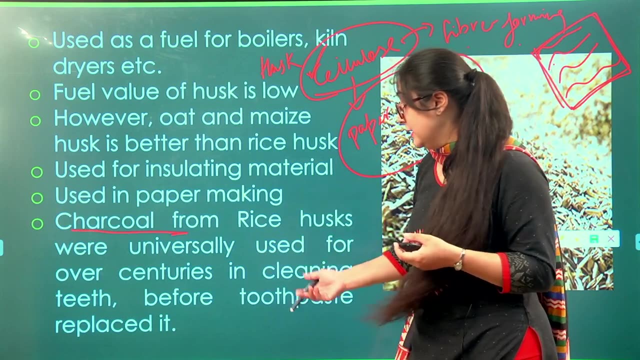 The husk contains charcoal, Which has been used, as we know That charcoal is a very, very good cleaning agent. It is known for its absorbing properties. So charcoal, because it contains charcoal, It has been used to clean teeth by people from centuries. 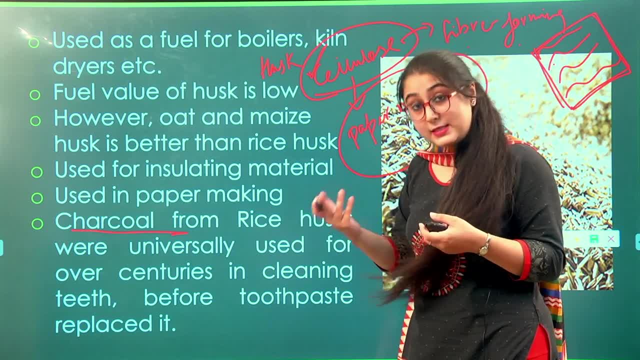 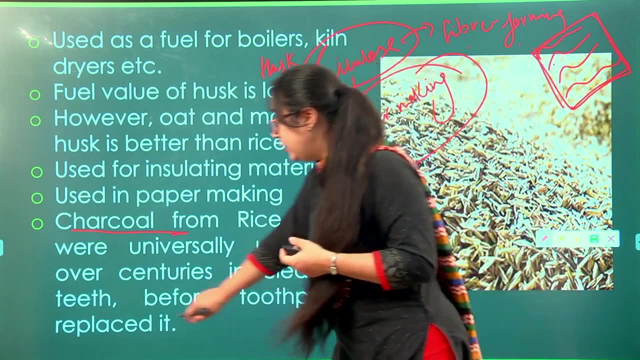 So before all these toothbrushes and toothpaste came into existence, People were utilizing husk even to clean teeth And to maintain oral health, So it has been used for cleaning tooth Just before toothpaste replaced it. So now toothpaste has basically replaced. 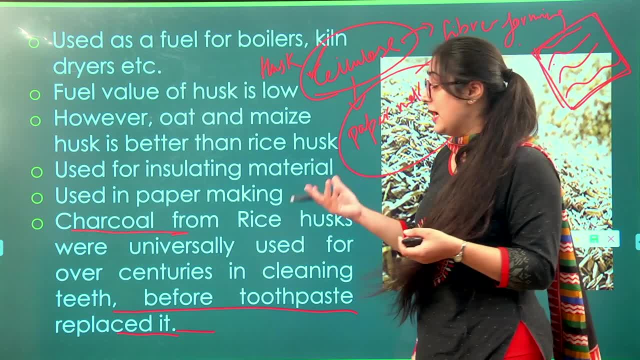 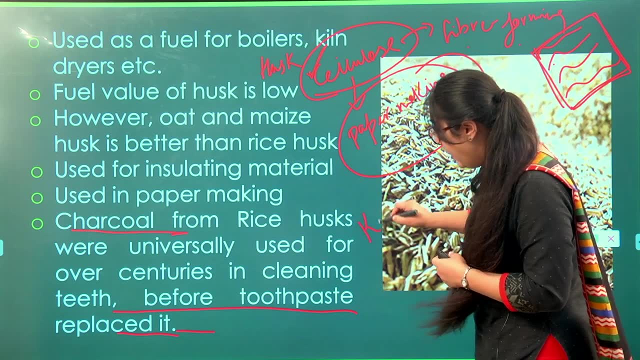 Almost all the use that husk was utilized As an agent for cleaning the teeth, And mainly in India. if we look at where it has been used, Mainly in Kerala. In Kerala, husk has been used for very, very long time As a good agent for cleaning the teeth. 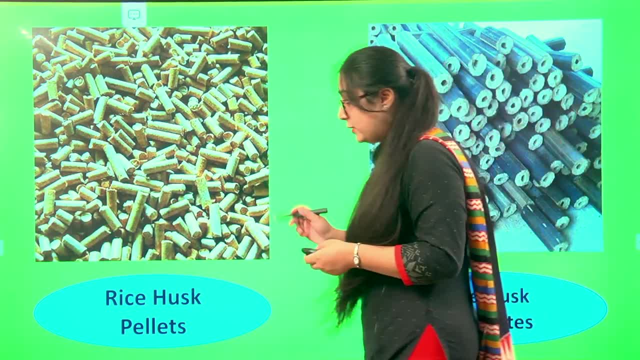 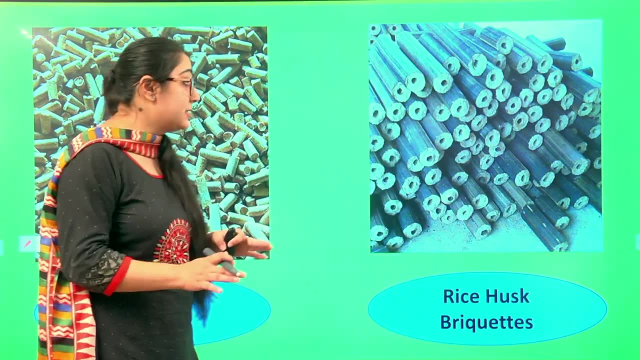 So now looking at some more. So, just as I told you right now, That husk has a use as a fuel, But it has a low fuel capacity. That is why husk is being utilized In the form of husk, Rice husk briquettes are being made. 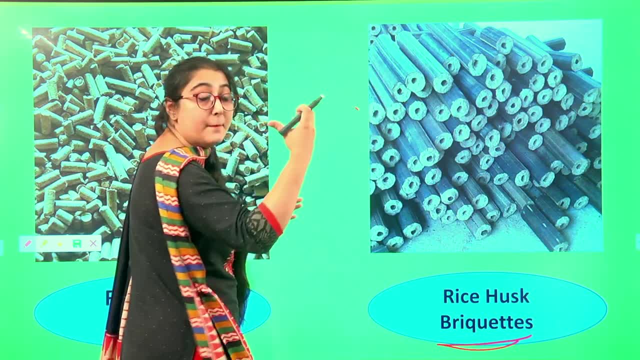 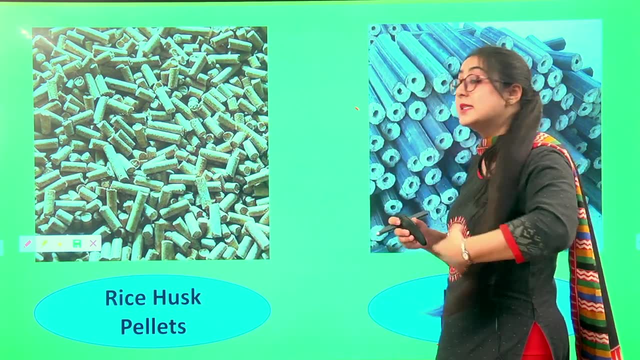 So if you look at over here, It is converted into a different compressed kind of a form, And similarly we have rice husk pellets. So what happens is Because the rice husk is somewhat loose And the fuel value is not very high. 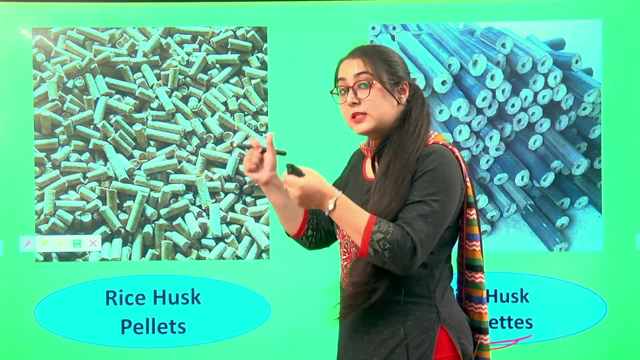 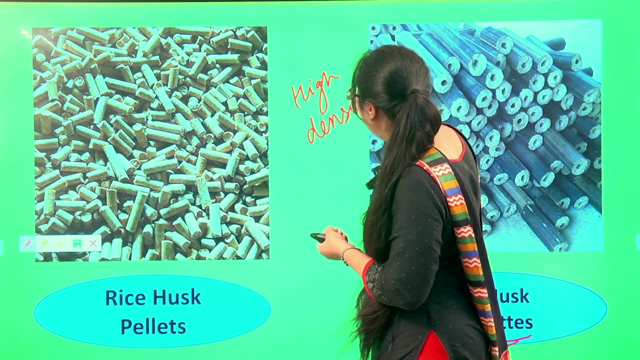 What we can do is We can convert the husk into this compressed kind of a form, Into a very. So what will it do? It will convert your husk into a very high density Form, And this high density Because now it will have higher density. 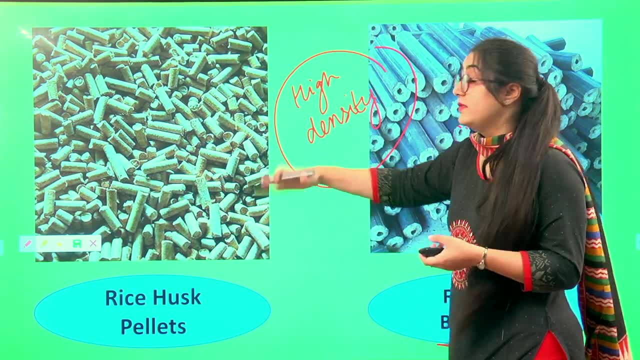 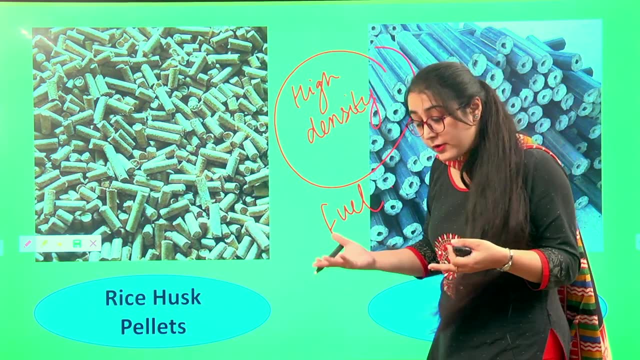 As compared to the loose husk, It can be utilized very, very efficiently As a fuel. So husk can be brought to a number of uses as a fuel In the kill dryers, boilers and many other functions In various other equipments and machineries. 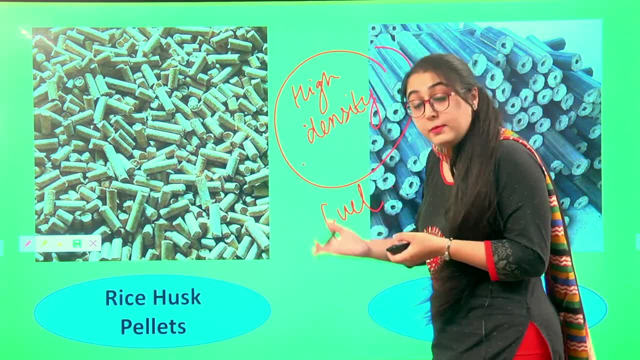 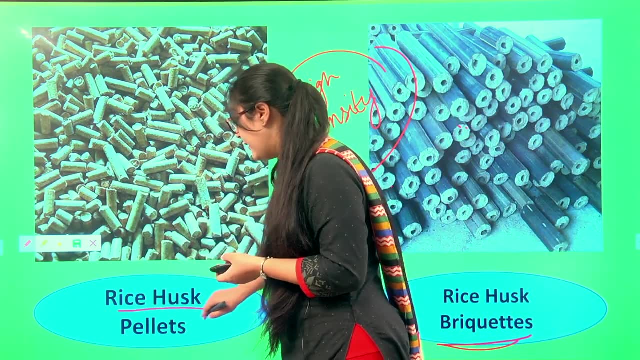 And for the betterment of its fuel value. Since its fuel value is somewhat lower, It can be converted into high density products Such as rice husk pellets, And then we have rice husk briquettes. So in both of these forms, 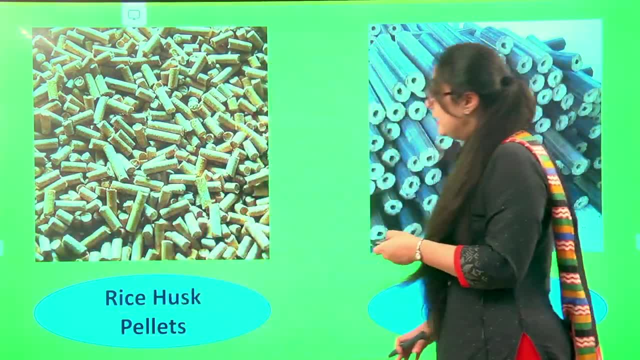 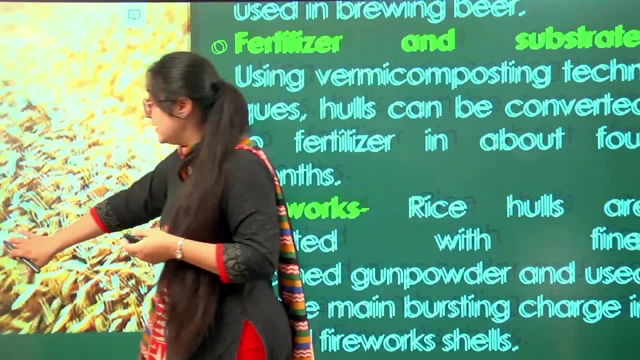 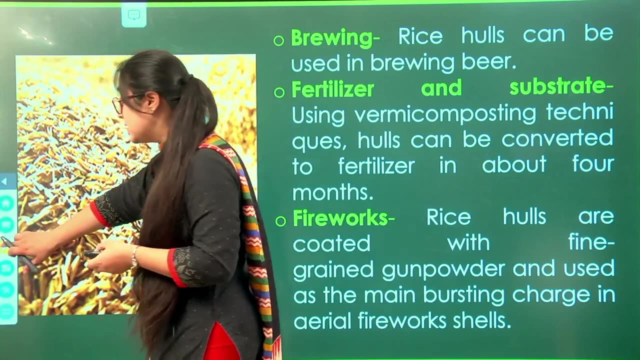 It can be utilized as a very good source of fuel. Next we have Brewing fertilizers and fireworks. So husk also find uses in the brewing industry. So husk also finds uses in the brewing industry. So generally Rice husk are used for brewing of beer. 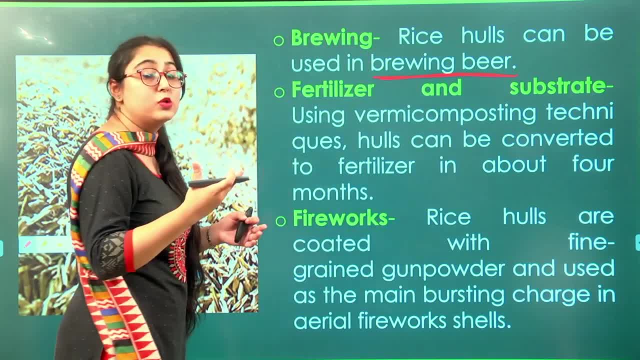 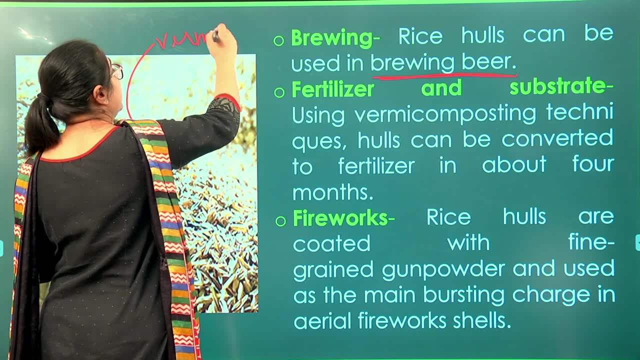 So they can be utilized For that purpose And also as a fertilizer and a substrate. So what we can do is This husk. with the help of vermicomposting, We can convert it into a good fertilizer. So what will happen is: 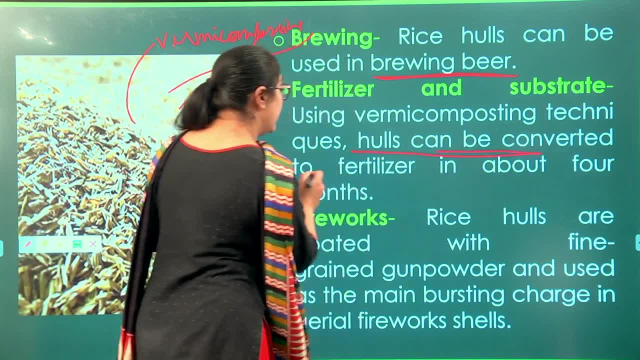 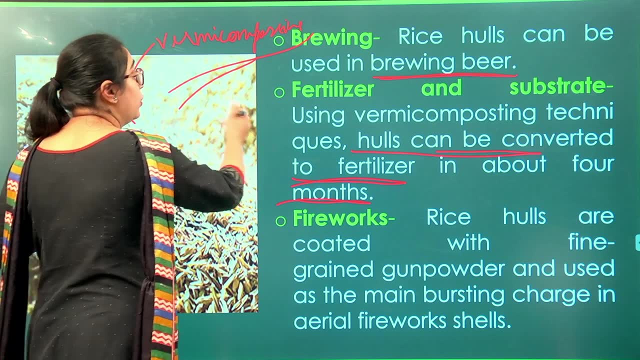 During vermicomposting, Hulks can be converted into very, very good fertilizers In about 4 months. So it will take this whole process of Converting the husk into a good fertilizer With the help of vermicomposting. 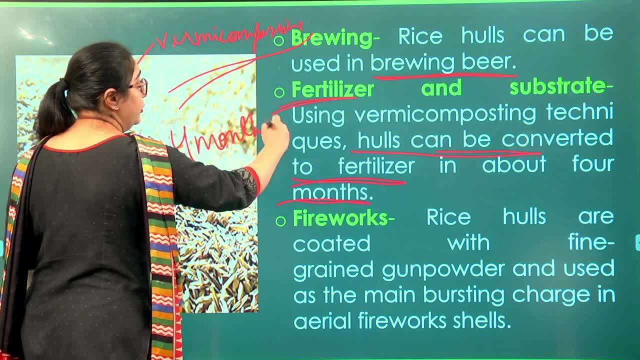 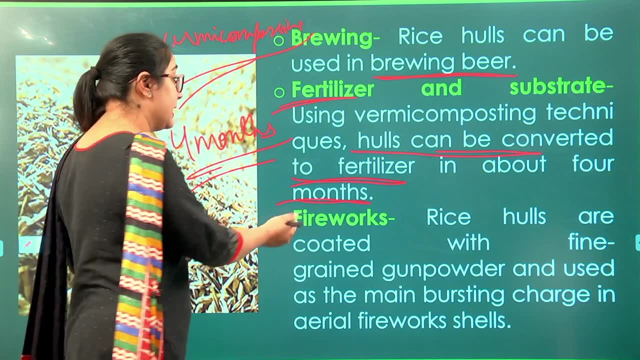 Will take around 4 months, And after that It is ready to be used as a very, very good Fertilizer and a substrate, And it can help in the Providing the nutrition to the plants And hence It has a very good use as a fertilizer. 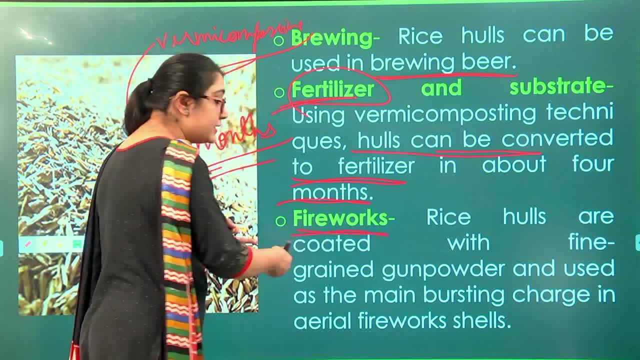 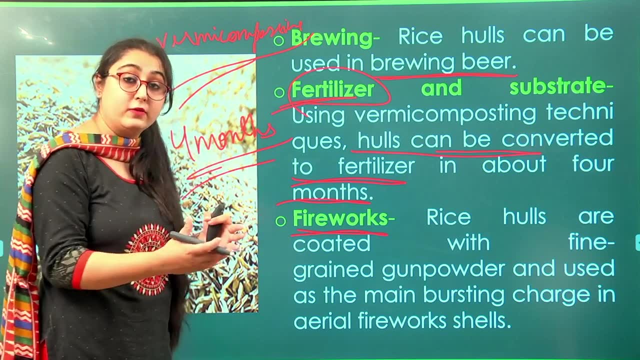 As well. Next is the fireworks. Now, this is A very interesting one to see over here: That husk Even finds use in the fireworks. So for the production of fireworks By this industry also, husk is being utilized. The reason is: 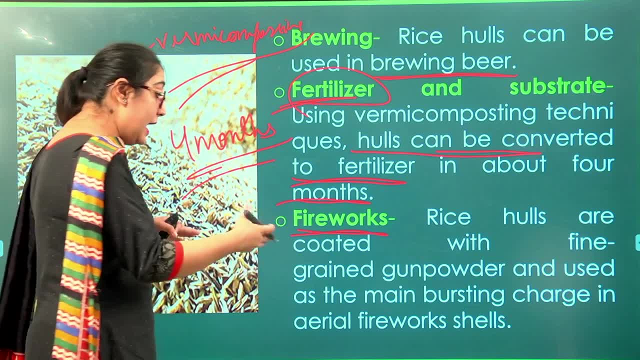 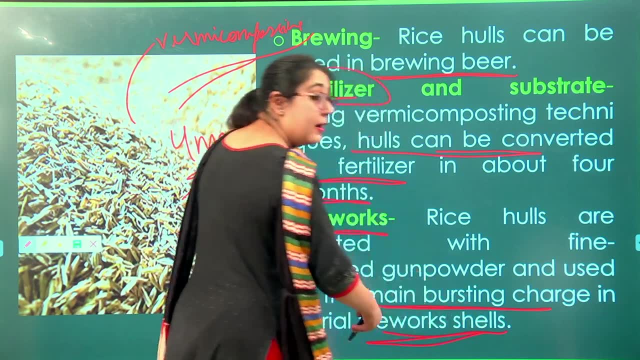 The husk can be coated with a gunpowder And it can be used for As a main Bursting charge in the Fireworks. So it is added in the fireworks shell After coating with a gunpowder And it can also be utilized in the fire. 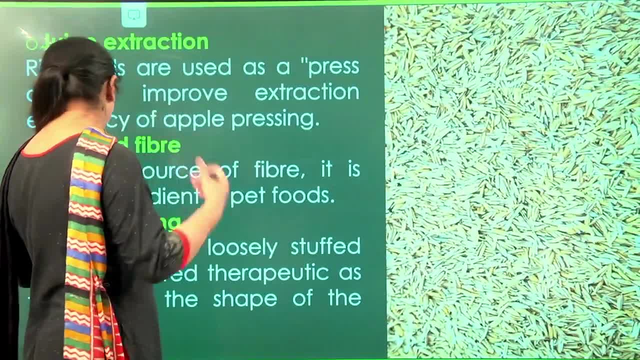 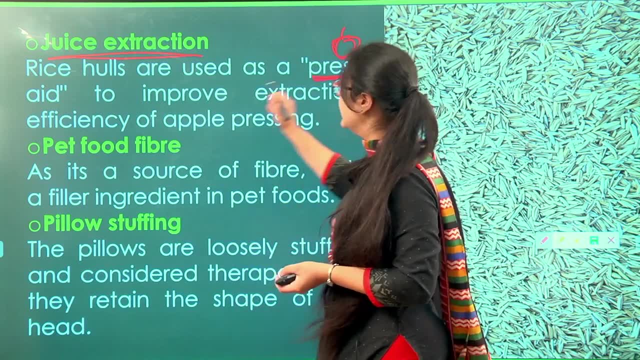 Fireworks. So now Some more uses we have is First. one is the juice extraction Hulks can be used as an extraction aid, As a press aid, Help in pressing And improve the efficiency of apple pressing. So it has been utilized very, very much. 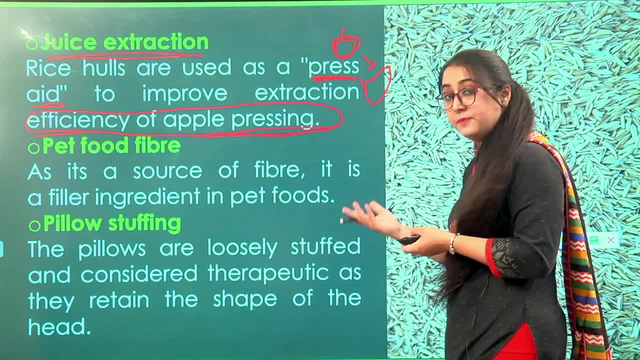 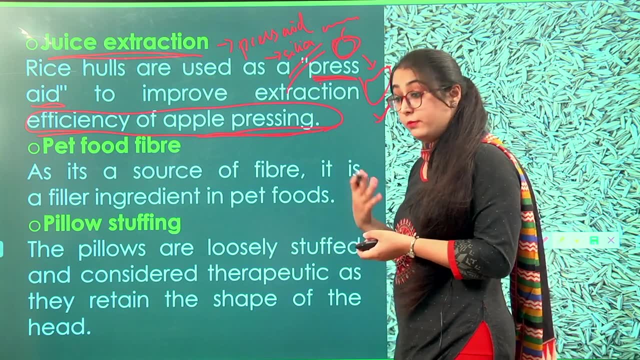 For the apple, Apple pressing, And It can be used for certain other fruits also. So next, We have as a pet food, fiber. We have discussed this also in brief, That because of High content of fiber present in the husk, 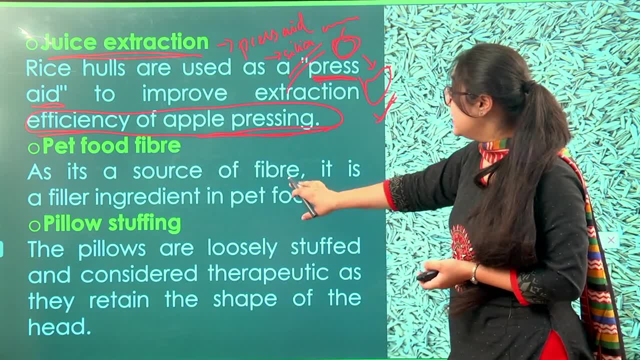 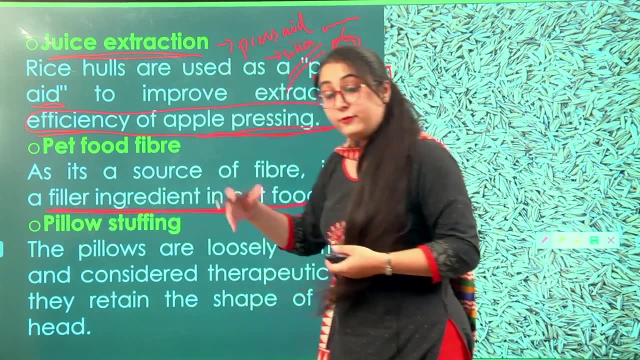 It can be used in the animal feed And, Because of the source of fiber, It is a filler ingredient in the pet. So what we can do is We can add this in the Pet foods as a filler ingredient, So the foods which are containing husk. 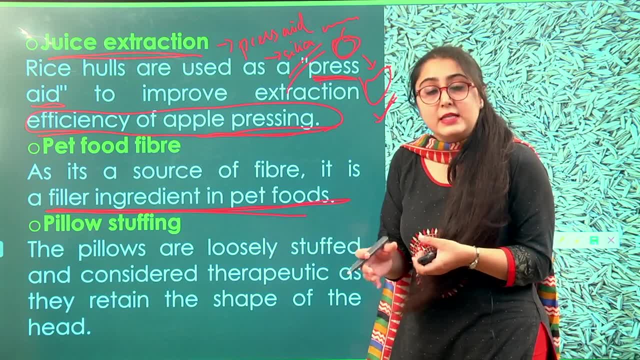 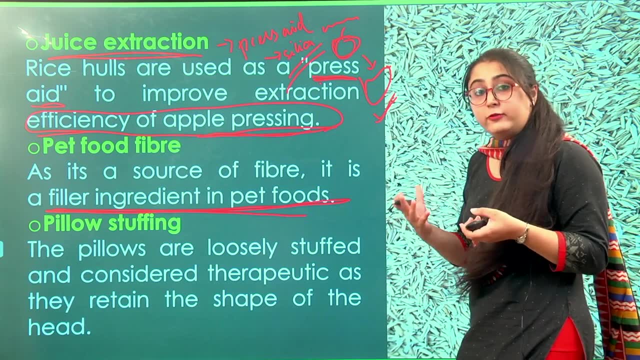 Because of high fiber, It will give a feeling of fullness For a larger amount of time To the animal, Because fibers will not be digested in the body. They will remain in the body for a very, very long time And give a feeling of fullness for long. 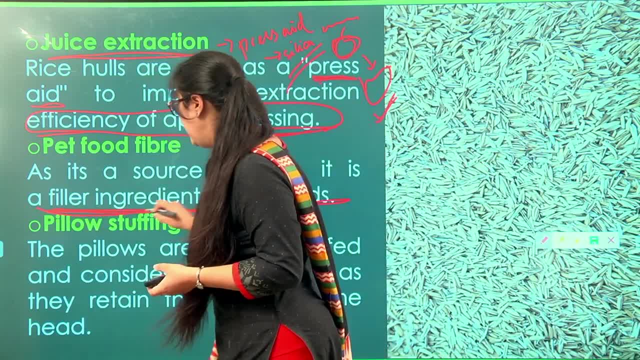 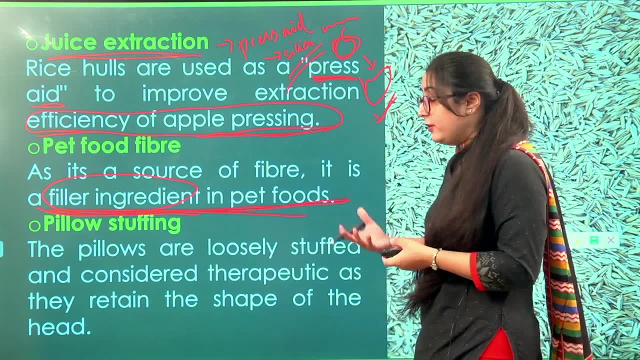 So, because of the property of fiber, It can be added as a filler ingredient In the pet foods. Next, we have used as a pillow stuffing. So if we, If we see the structure of the husk, It is such That it is able to retain very, very good shape. 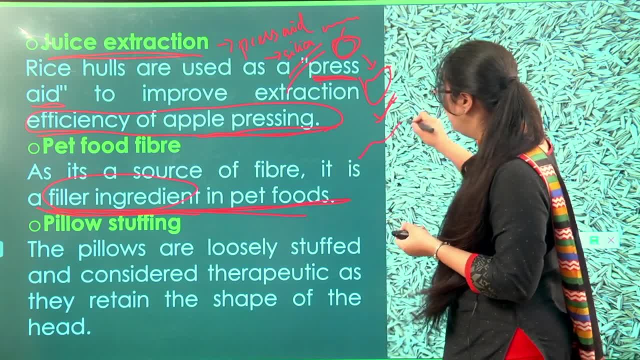 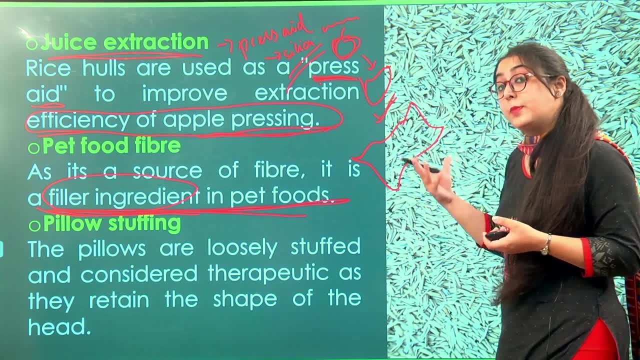 So it can be added to give the desired fluffiness In case of a pillow, And what will happen is The pillow will retain its shape, Retain the shape of the head. For that reason, It is a very, very good stuffing for the pillow. 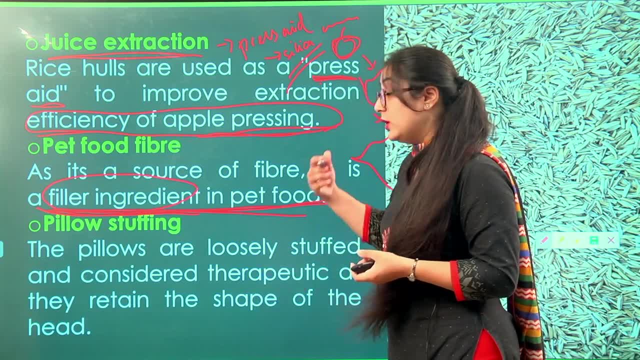 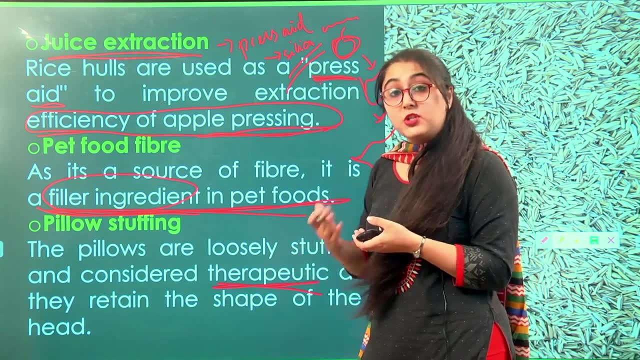 So pillows are loosely stuffed And are considered. So the use of husk for pillow is considered therapeutic. Why it is considered therapeutic? Therapeutic meaning giving a beneficial health effect- Because it retains the shape of the head. So once it retains the shape of the head, 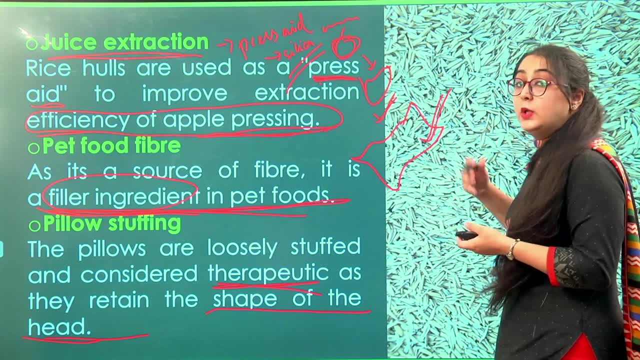 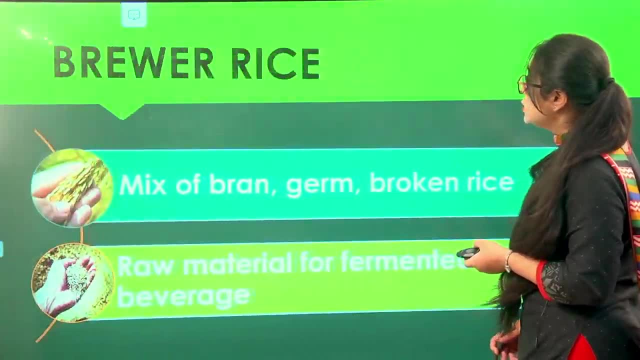 It will be very, very comfortable. The pillow which is made Using this husk will be quite comfortable And, again for this use, it can be utilized. So now, next byproduct we have is the brewers rice. Now, the brewers rice, or the broken rice. 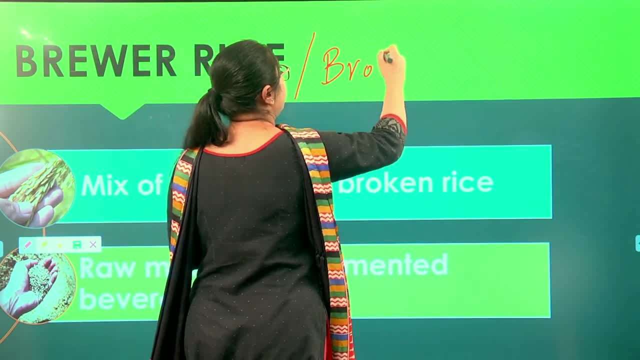 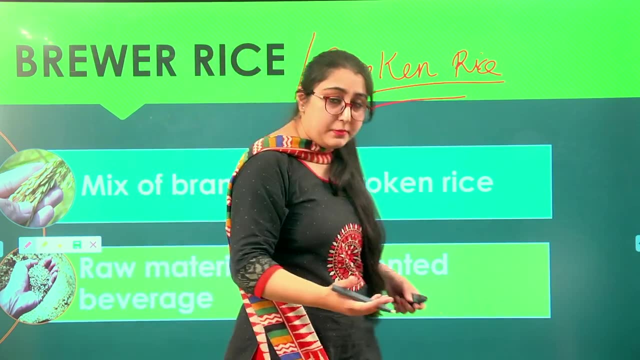 It is also known as the broken rice, So the broken rice only. we have the second name as Brewer rice. Both of them mean the same. Now sometimes we can obtain this Mix of bran germ and broken rice. The mix can be obtained. 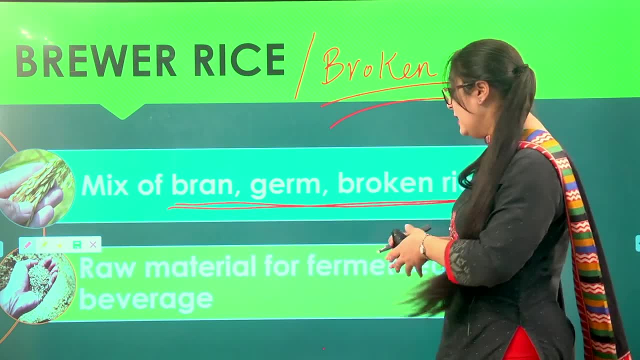 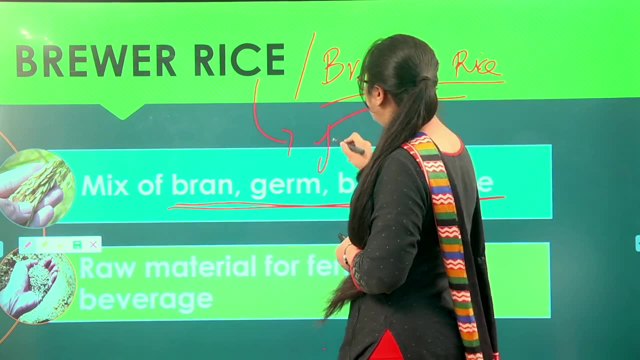 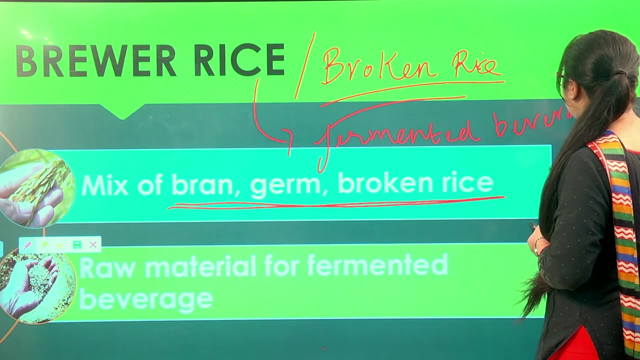 Sometimes it can be contaminated with the bran and the germ And the raw materials for fermented beverages. So it is a very, very good raw material For producing of fermented beverages, Meaning it will find a very, very good use in the alcohol industry. So for the fermented beverages it can be used. 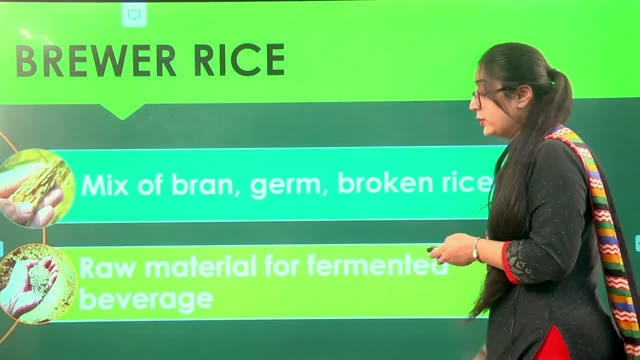 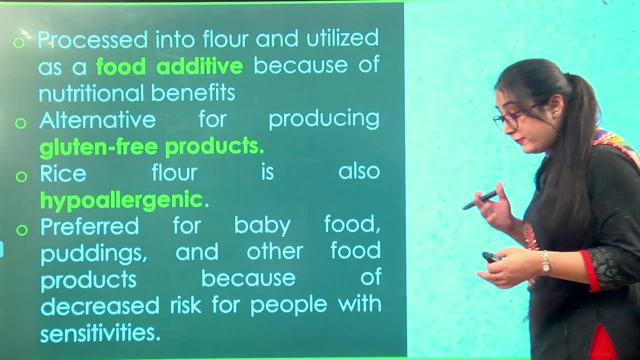 So now let us look at the uses of the broken rice, Or the brewers rice, in detail. So first one we have is that It can be processed into a flour. So before we discuss this point, We should know that, since rice does not contain gluten, 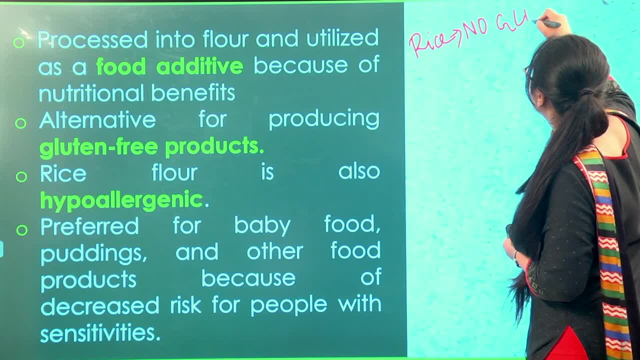 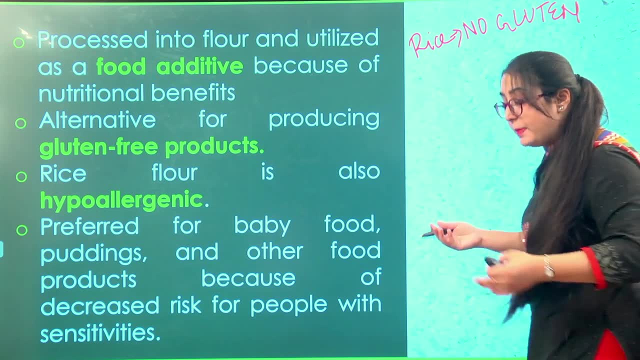 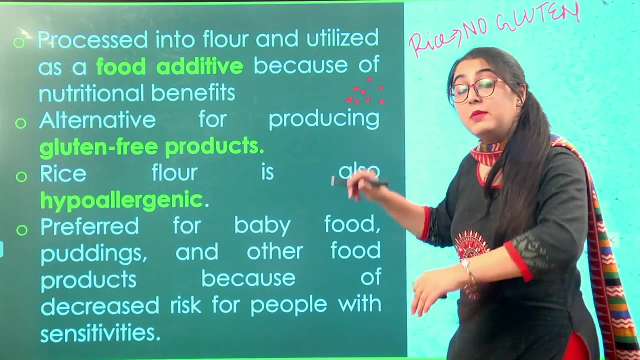 There is no gluten in the rice. Hence rice can be produced to make gluten free products. So what will happen is we have broken fragments of rice. So all these broken small, small pieces of rice need not go waste. They can be very easily converted into the flour. 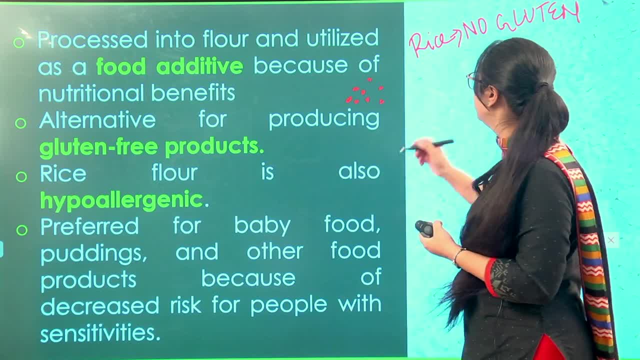 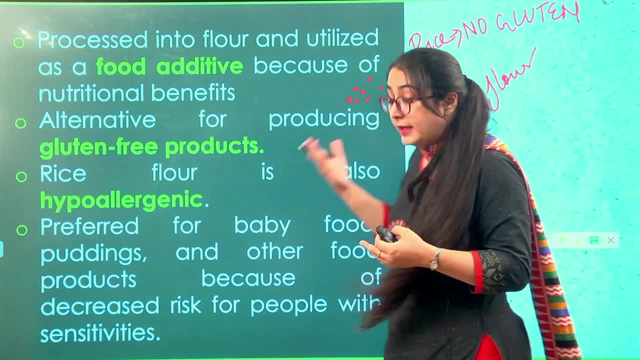 So they can be milled, and during the milling It can be converted into flour. So what we can do is we can make rice flour out of this rice, And once we are making rice flour out of rice, This rice flour can be utilized to produce a number of baked products. 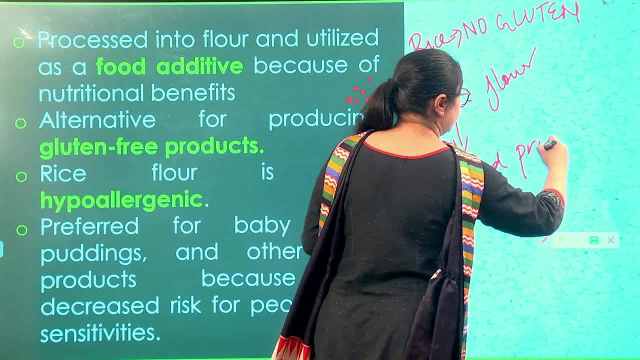 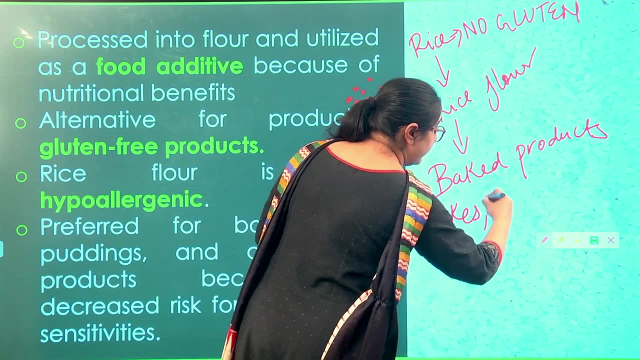 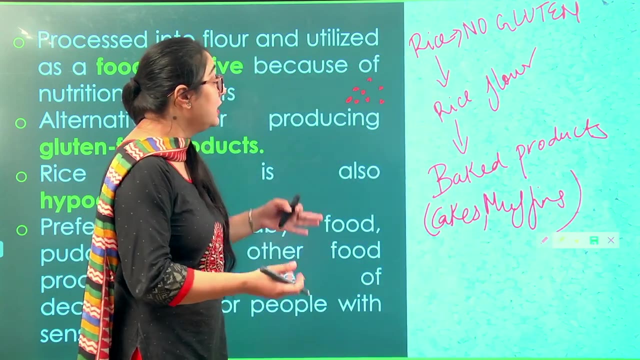 So, for example, the products which are made from the rice flour Include a number of products, for example, Even cakes, and then even certain muffins, Cookies. all of these have been made during the rice flour. So what is the need for producing baked products from the rice flour? 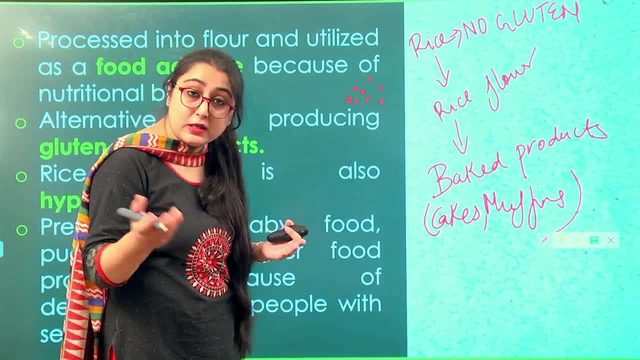 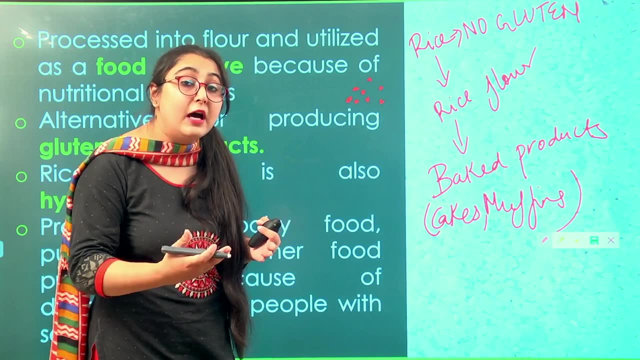 We already have a number of baked products in the market, Such as cake, muffin, biscuits, and all of them taste very, very good, But the need to make them instead of wheat flour or refined flour with rice flour Is that wheat flour and refined flour contain gluten. And people which are suffering from gluten intolerance, Or people suffering from celiac disease Who cannot consume gluten at all, Need alternatives which are gluten free. Now, because rice does not contain gluten, It is completely gluten free- It can be brought to producing a number of products. 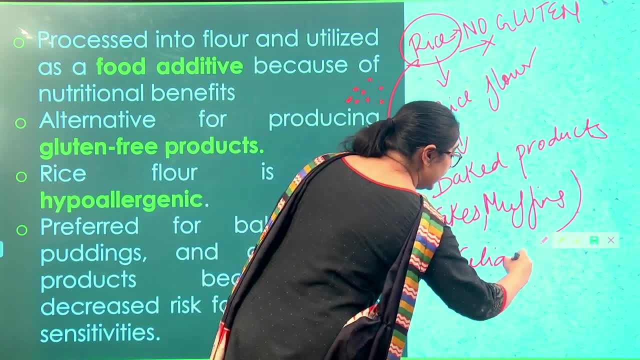 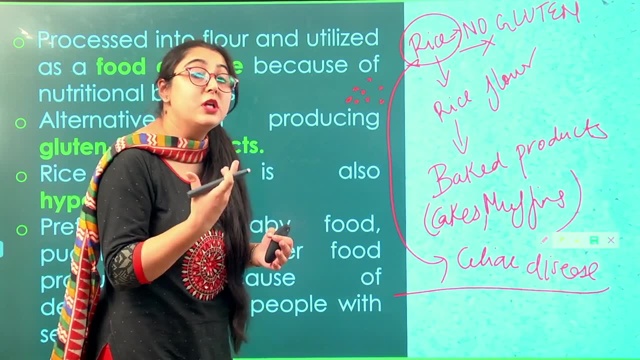 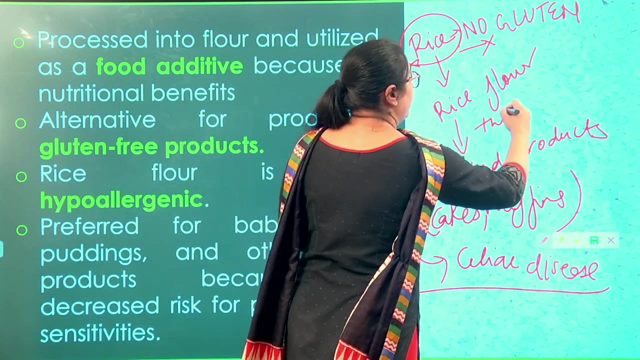 For people suffering from celiac disease. So this is where rice flour has a very, very good use, And also because of the good gelatinization properties of the rice starch, It can be utilized as a very, very good thickening agent also. So even, for example, in custard powders and all this. 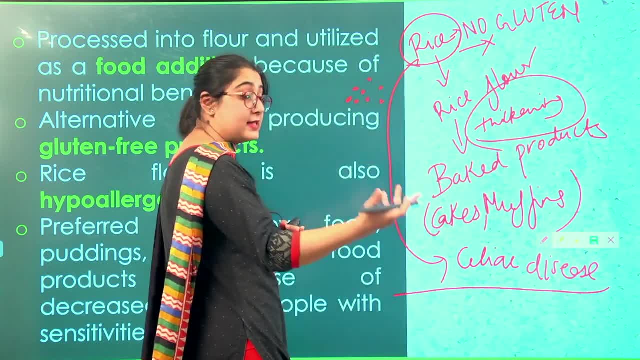 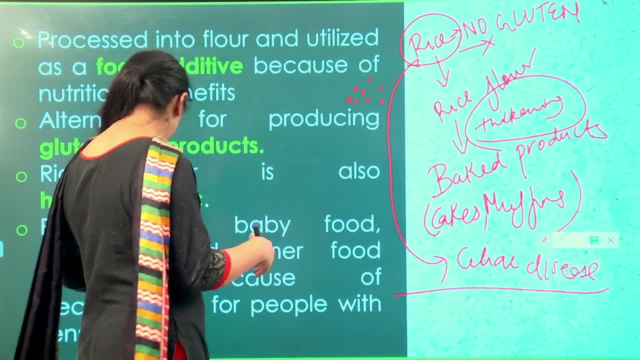 Where the desired consistency is there, Where the desired thickening is required, Rice flour can again be added. So rice flour can be used for a number of uses in the food industry. So again, if we look at the uses now, So it can be processed into flour. 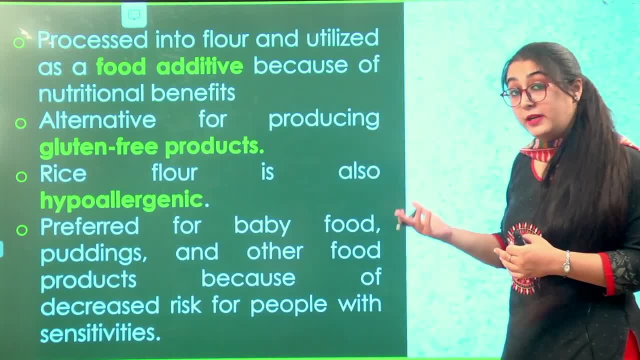 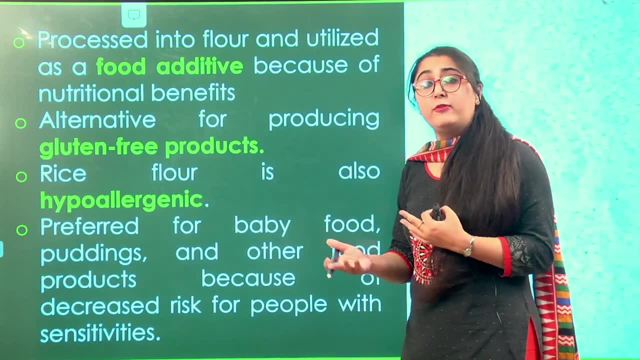 And it can be used as a food additive because of its nutritional benefits, So not only for the production of a number of food products, As we have discussed, for people for celiac disease Or simply for thickening agents, and all this Because it has a lot of nutritional benefits. 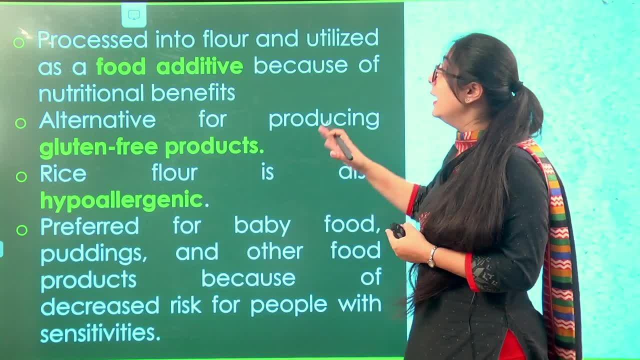 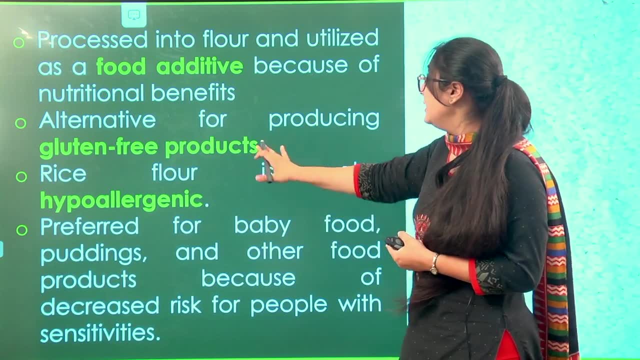 Because it will be rich in protein and fibers. and all of that It can be added as a food additive in some products. We can add it as an additive simply to improve the nutritional quality, And then it is an alternative for producing gluten free products. So, as we have already discussed, Because rice does not contain gluten, Its number of gluten free products can be produced from rice. For people suffering from gluten intolerance or celiac diseases, Rice flour is also hypoallergenic. So when we say hypoallergenic, 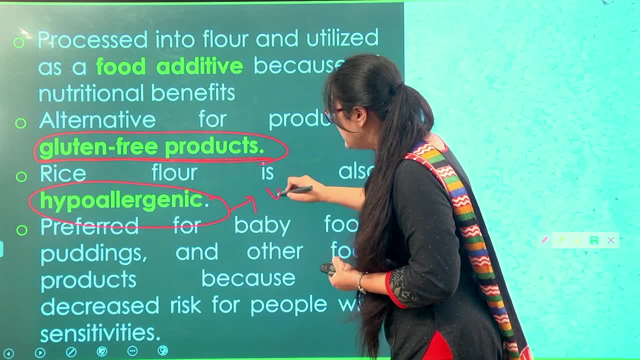 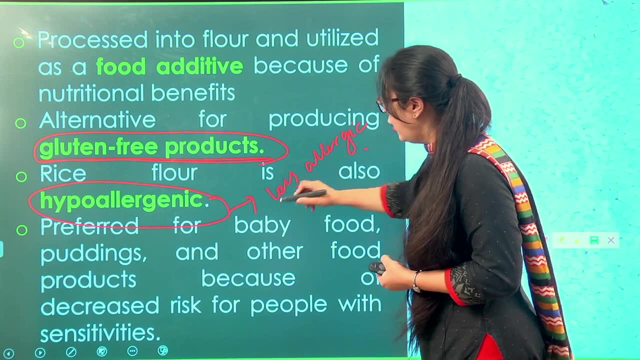 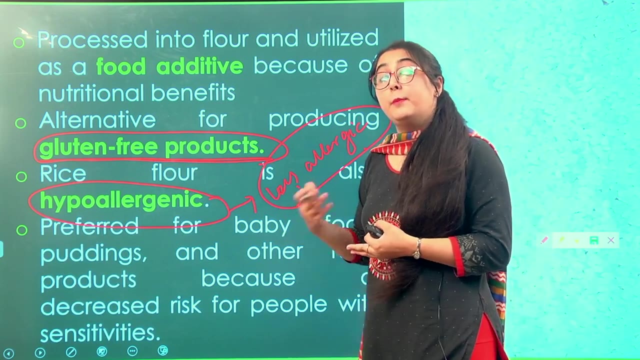 We mean something which produces very less allergic reactions. So if we compare, We have a number of food products which give a lot of allergic reactions to people. For example, we have peanuts and we have soya beans. All of these produce a number of allergies in a lot of people. 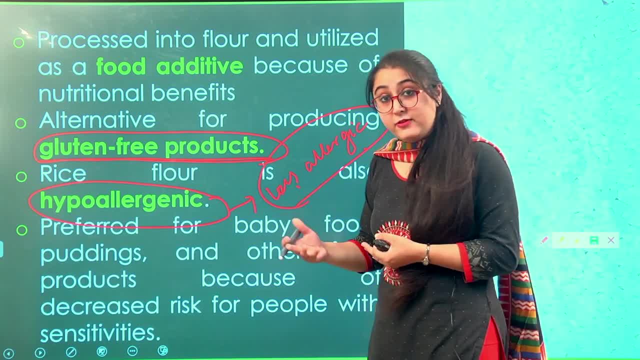 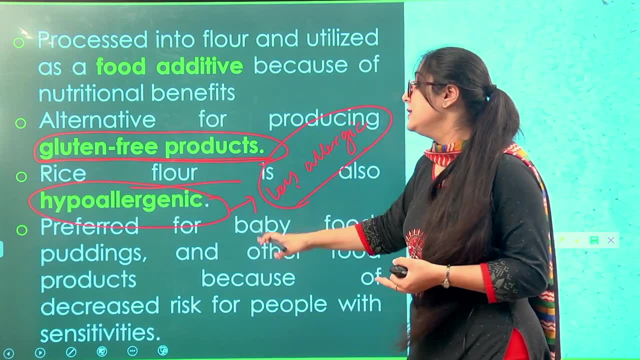 So for such kind of people, which are extremely sensitive And might suffer from a lot of allergies from the food products, Rice flour is a very, very good option. The reason being is that it is hypoallergenic, That is, very low cases or very low chances of allergies are being reported from it. 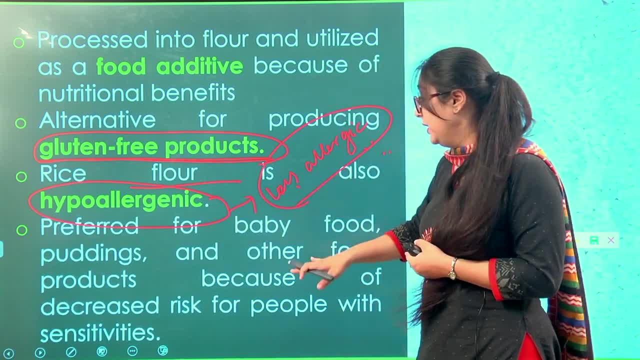 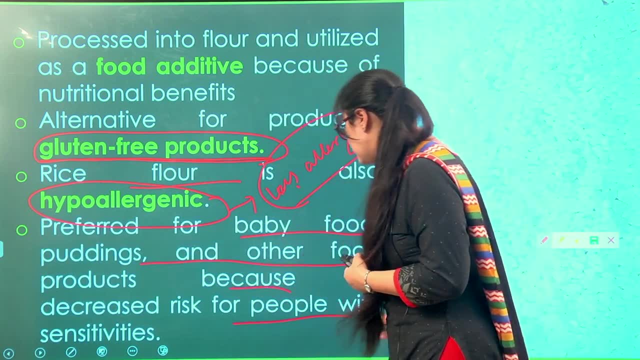 So for this reason, Because it is hypoallergenic, It is used for producing baby foods, puddings and certain other products Because of the decreased risk of people with sensitivities. So when we say decreased risk of people with sensitivities, 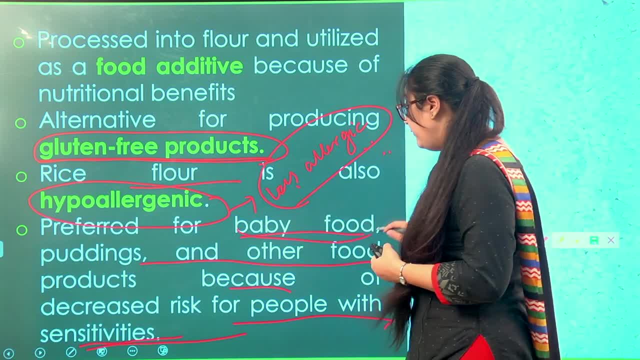 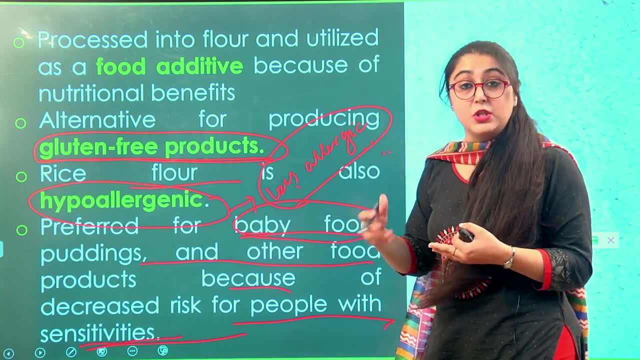 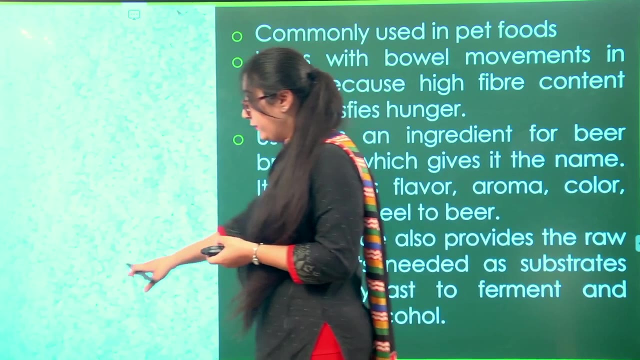 It can preferably be put to use for baby foods, Because there We want to extremely be focused, while producing the food product, That the food product should not cause any kind of allergy to the small child. So Now looking at more uses of the broken rice. 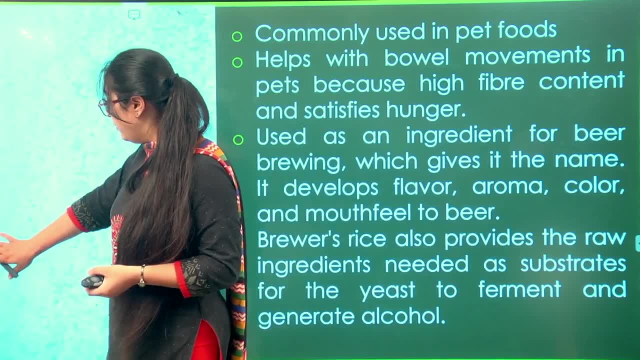 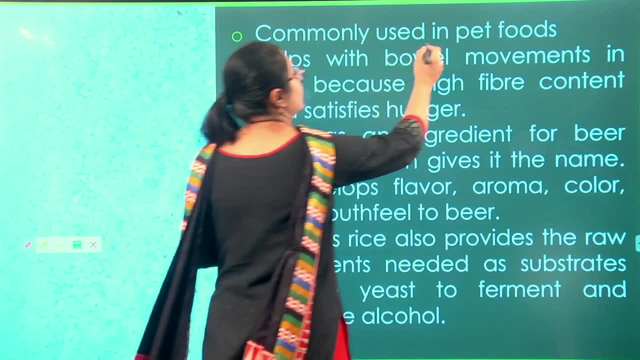 So broken rice has a number of more uses which it can be put to, And it includes that It can be commonly used in the pet foods. So, just like husk, It can also be brought to use as a pet food, Since it is a very, very good source of fibre. again, 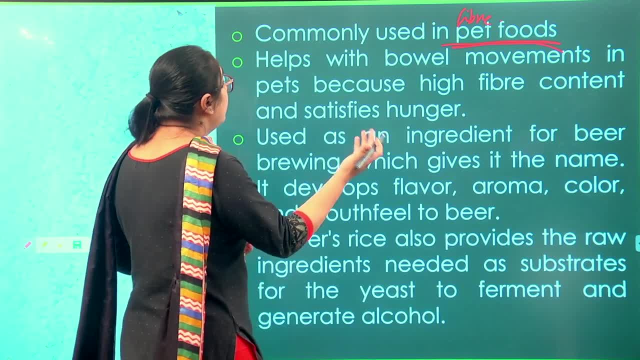 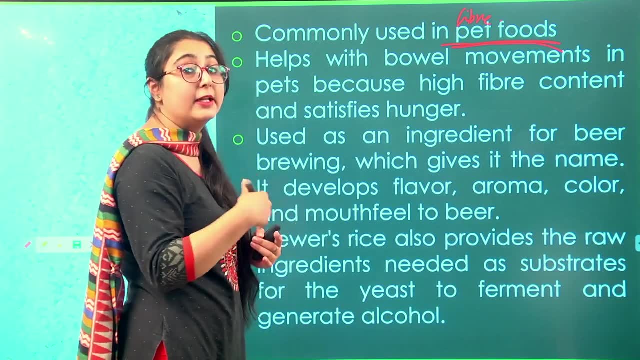 It helps. It helps with the bowel movement Pets- because high fibre content. So same reason here. also, Because of its very, very high fibre content, It can help in the bowel movement And give a feeling of fullness for long And thus satisfies hunger. 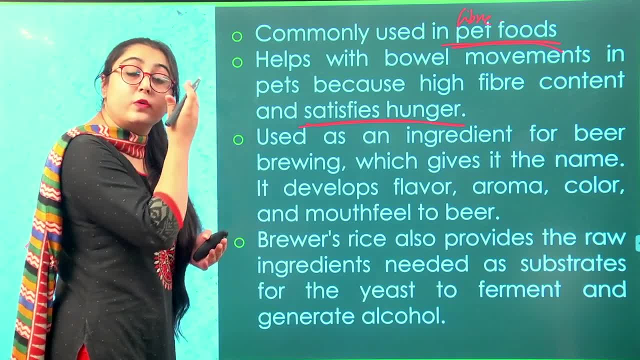 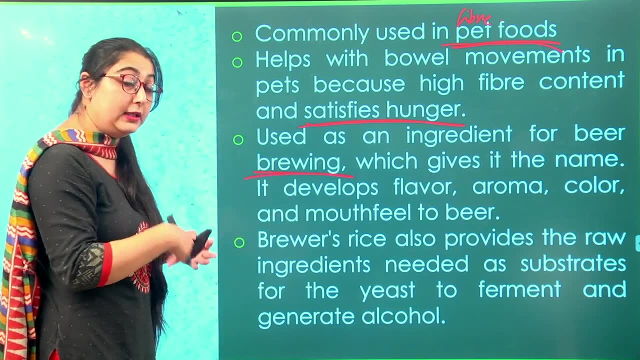 It is used as an ingredient in the beer brewing also. So one of the main uses of the broken rice Is that it is used as an ingredient for the beer brewing. For this reason only, The broken rice has got its desired name, That is, the brewers rice also. 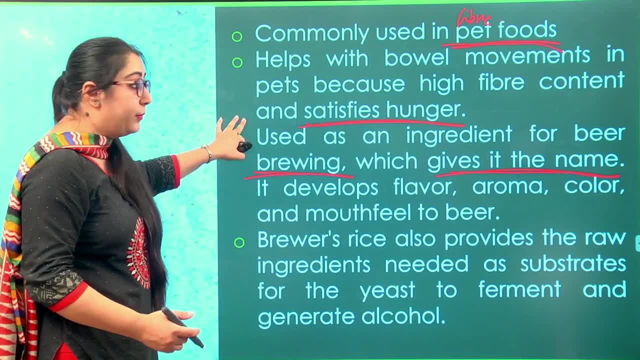 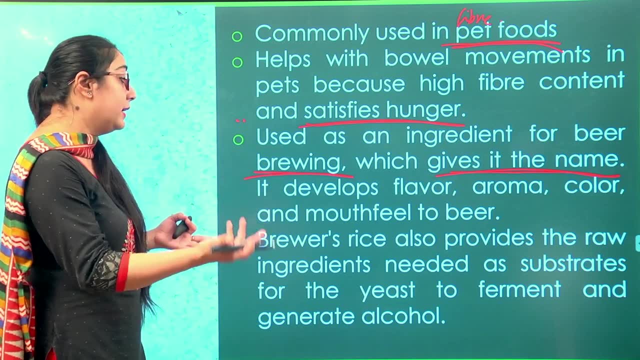 Because it has a very, very good use in the beer brewing And certain other alcoholic beverages. So what happens is, in the production of these beers, The flavour, aroma and the colour and the mouth feel Is. all of this is developing When we are adding the broken rice. 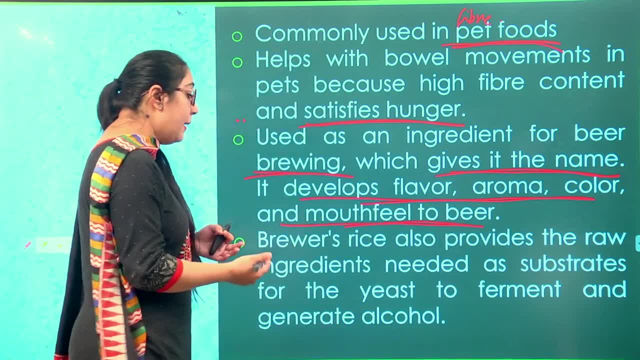 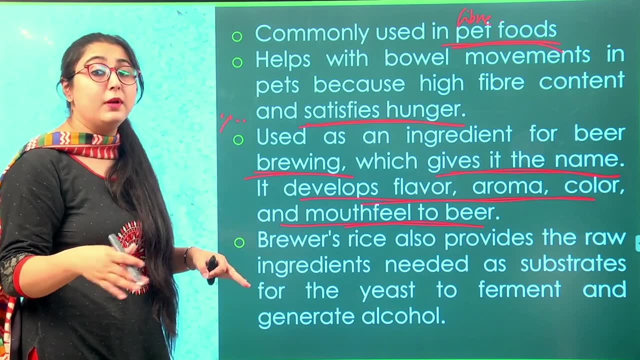 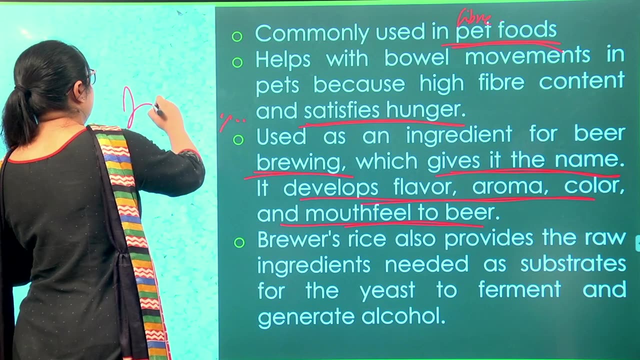 Mouth, feel flavour, aroma, all of this. But there is one disadvantage is that When we are utilising broken rice And not some other ingredient- For example, We can utilise barley hops- all of these are also utilised. The colour of the beer obtained is somewhat lighter in colour. 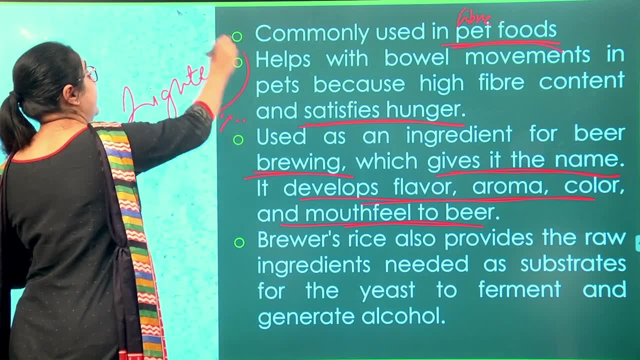 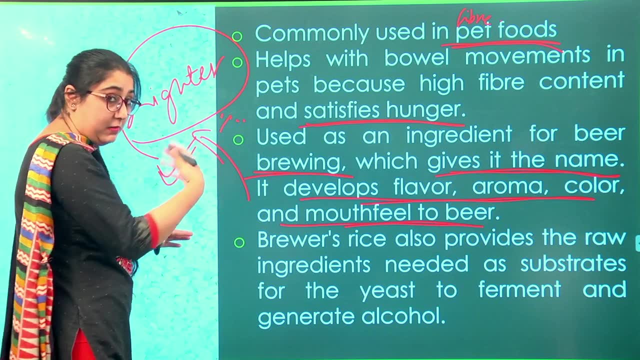 And when we go for beer, The lighter colour is not that desirable, But still, rice has a very, very good use. Even despite of the light colour, It is being used very, very much. The reason being is that It is much, much cheaper and easily available. 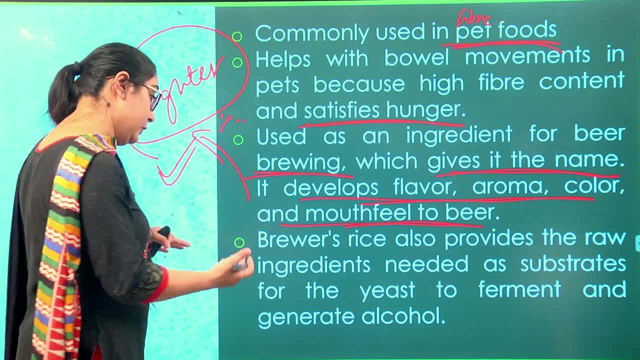 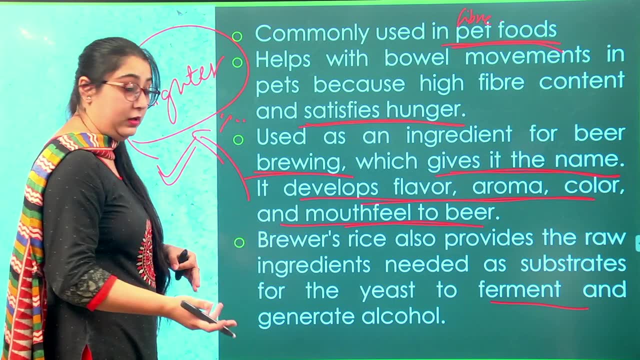 So it has a very good use And it gives a very good aroma. also, The brewers rice also provides the raw ingredients And it has substrate For the yeast to ferment and generate alcohol. So not only the good flavour or the colour, It also helps in giving the desired substrate. 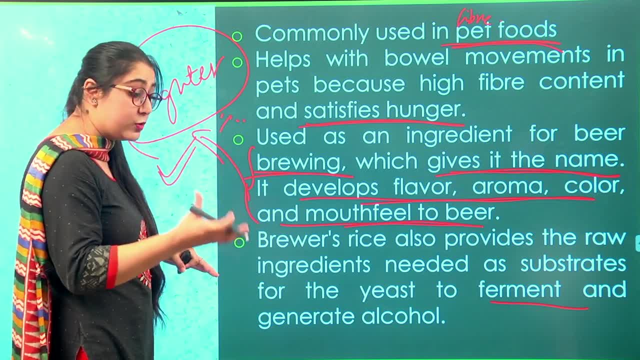 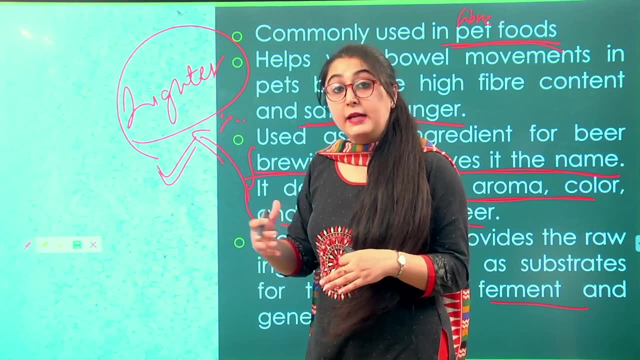 It acts as a very good substrate for the yeast Which is present in the alcohols Which we are adding in the alcohols So that the yeast can act on this broken rice And it can ferment and generate a good amount of alcohol. 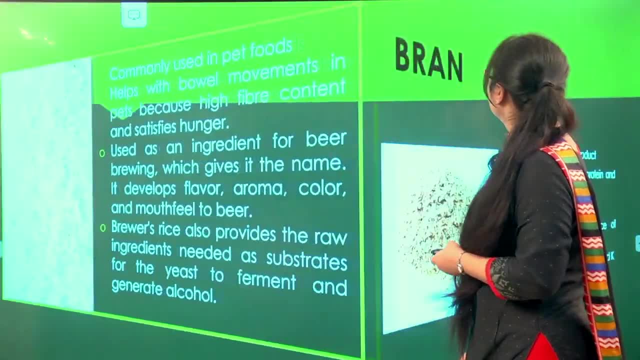 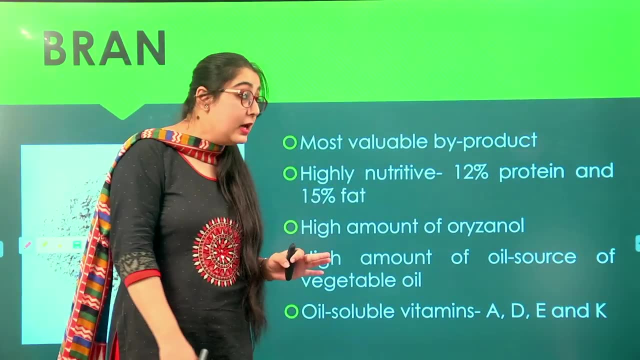 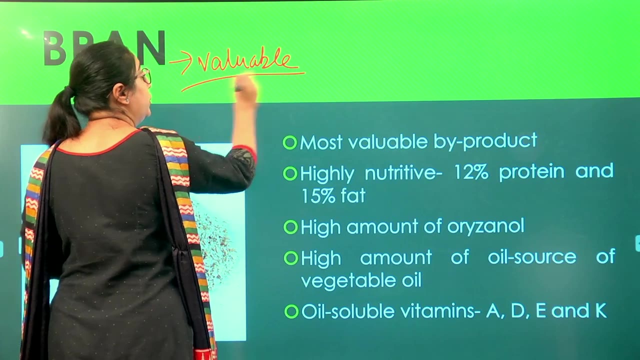 So, looking on this, So looking on to our third by-product, Or the final by-product which we have is the bran. So now bran is the most valuable by-product And the most important one Which we are to discuss. The reason being is that of its nutritional quality. 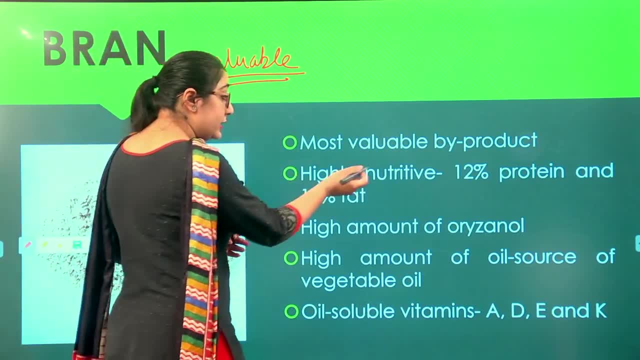 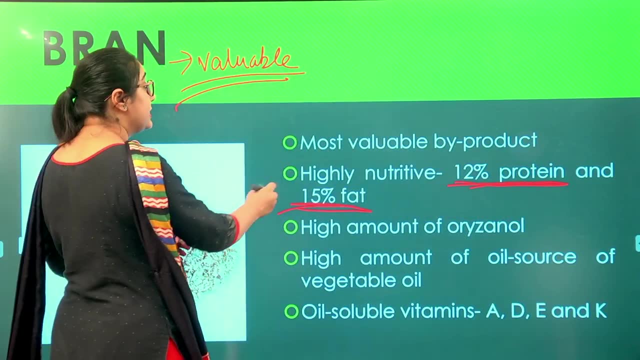 So the nutritional quality of bran is very, very high. So it is highly nutritive. It contains 12% protein And it contains 15% fat. For this reason, It is one of the It is the most valuable by-product of the rice milling industry. 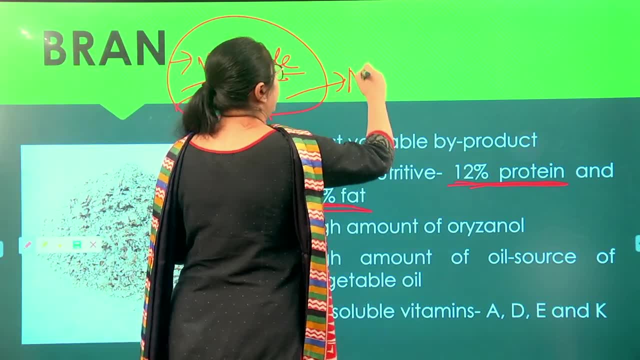 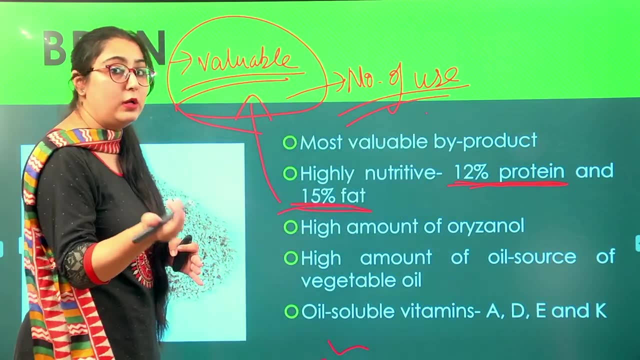 And for the same reason, It has a huge number of uses. it can be put to As a Because of a good nutrition. So high amount of orisonol as well. So why it contains high amount of orisonol? Because rice is a very good source of orisonol. 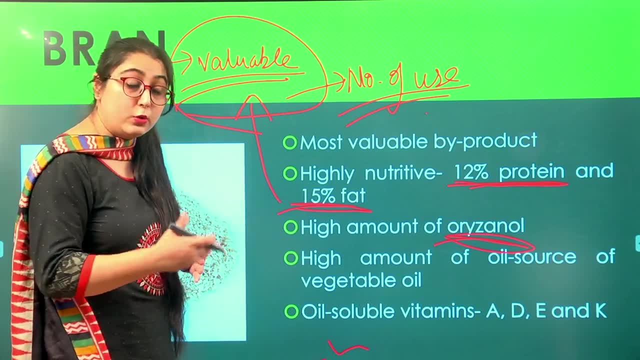 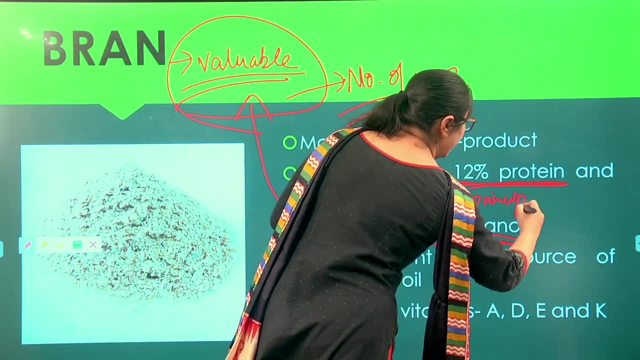 Right. And the bran coming from the rice also has a good amount of orisonol. So orisonol, As you already be knowing That, it is the principal Protein which is present in the rice. So the main protein present in the rice is orisonol. 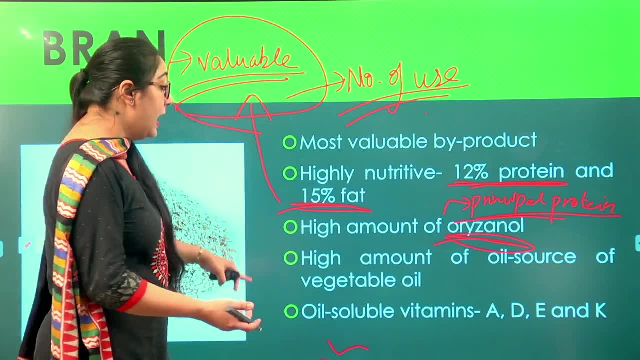 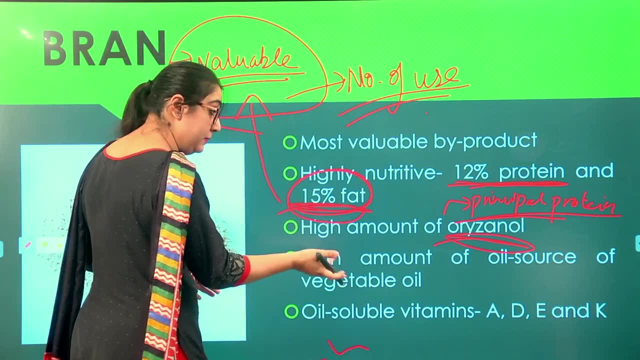 So it has very, very high in orisonol also And high amount of oil source of vegetable oil. So because it contains high amount of fat- That is around 15%- It can be used as a source of vegetable oil, So even oil can be extracted out of it. 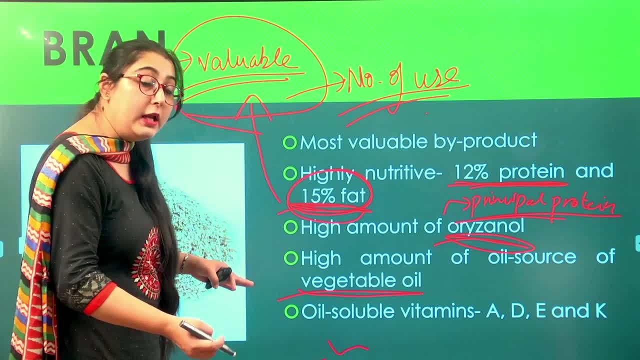 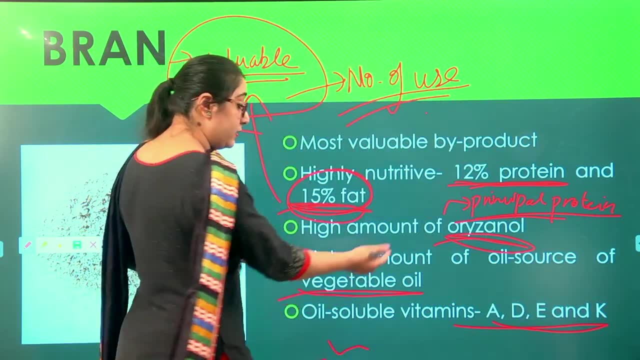 And because it is a very good source of oil, It will be a very good source of oil soluble vitamins as well, Such as vitamin A, D, E And K. Generally, vitamin E is present in very, very good quantities in the rice bran. 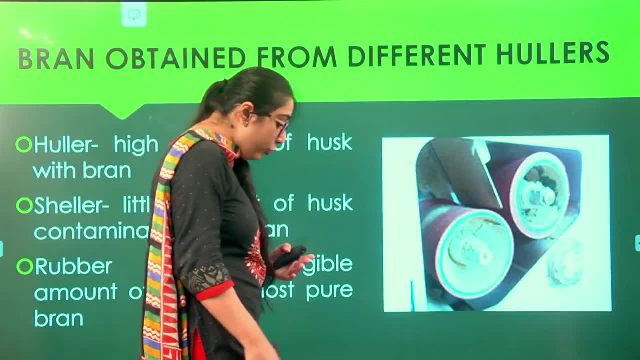 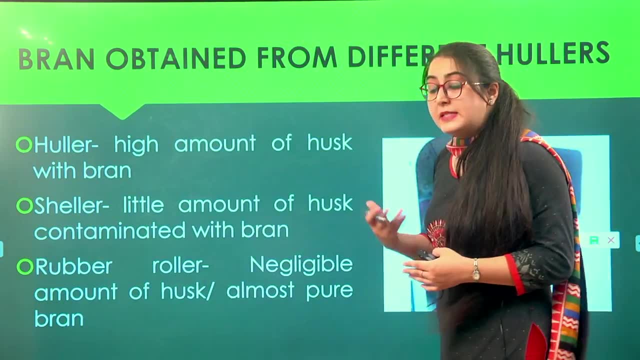 So bran obtained from different hullers. So before we study bran further in detail, It is very important to look at the bran which is coming from different hullers. So what basically happens is See bran has a number of uses. It can be utilized. 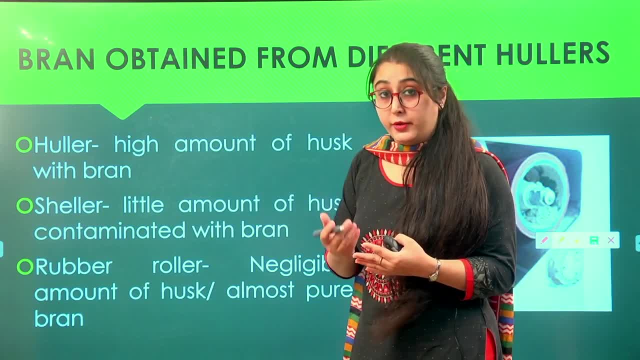 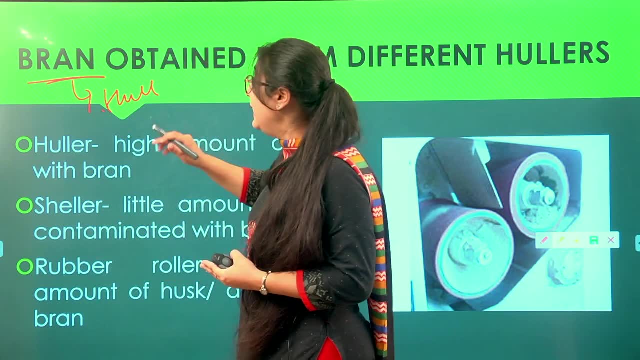 But for that purpose The bran should be very, very pure, And the bran should not be mixed with the hull Or with certain other raw materials. The main contaminant is that the bran can be mixed with the hull or husk. Okay, 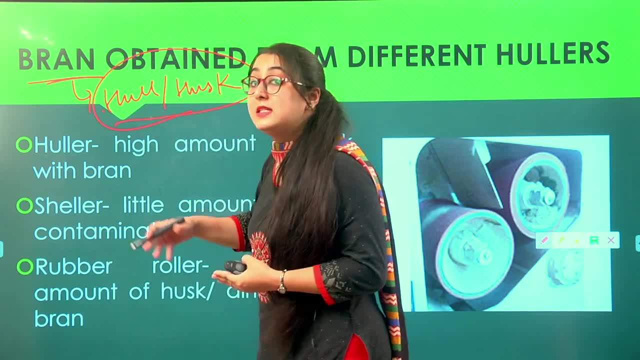 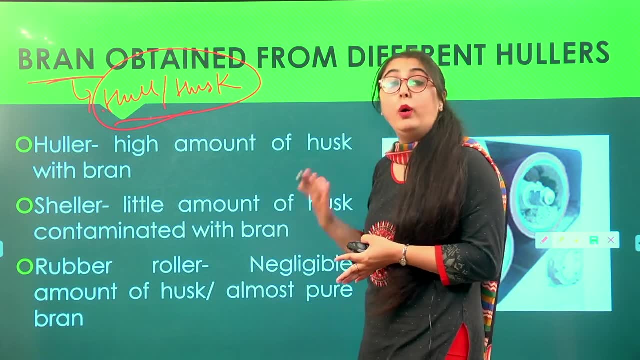 So it can be mixed with the husk or the hull, And if it is contaminated with amount of husk, Then it cannot be utilized very efficiently. So, for example, oil extraction is being done And the bran is contaminated with the husk. 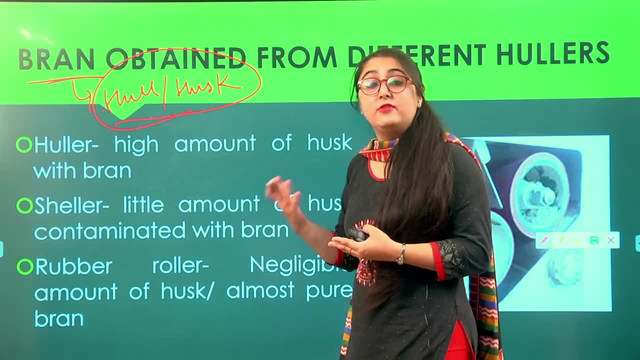 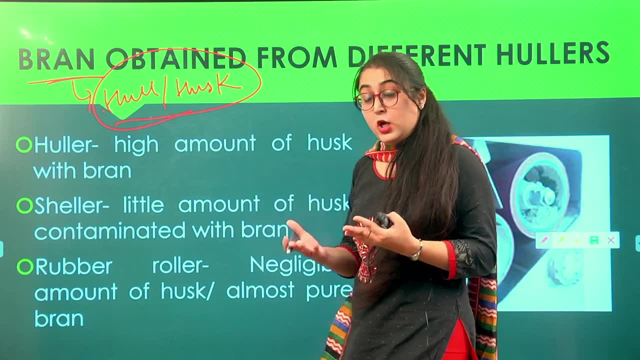 Oil extraction cannot be done very well And the result: efficiency all of that will decrease. So what we want is What is desired, is The equipment that we are choosing for the milling Should be done very, very wisely, So that not only the milling of the rice is done properly. 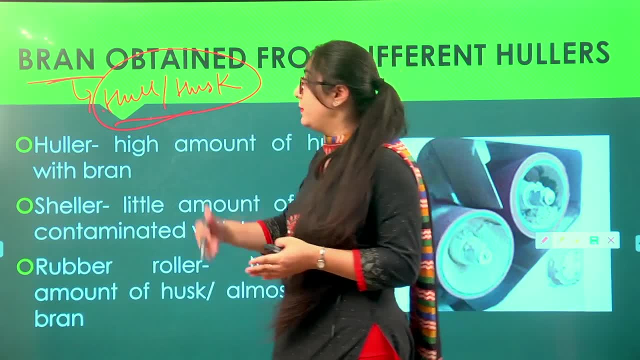 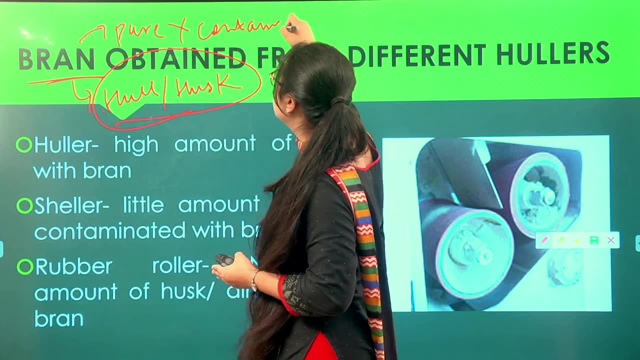 But also the byproducts which are being obtained, Such as bran. They should be pure in its form. They should not be contaminated. So if they are contaminated, What will happen is They cannot be put into good use. So for that reason, we are studying the bran. 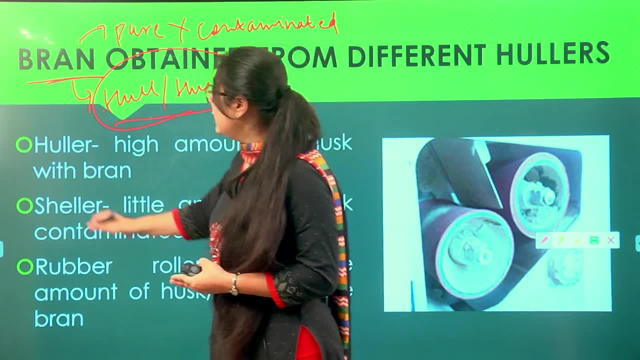 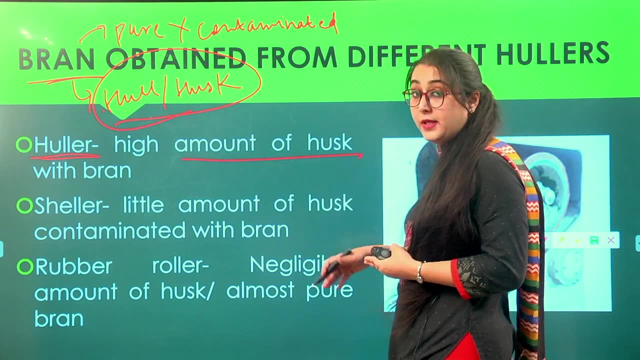 Which is being obtained from different equipment. So if we look at the bran, If we look at the bran coming from certain hullers, It contains very, very high amount of husk. with the bran is present, It is contaminated in very high quantity with the husk. 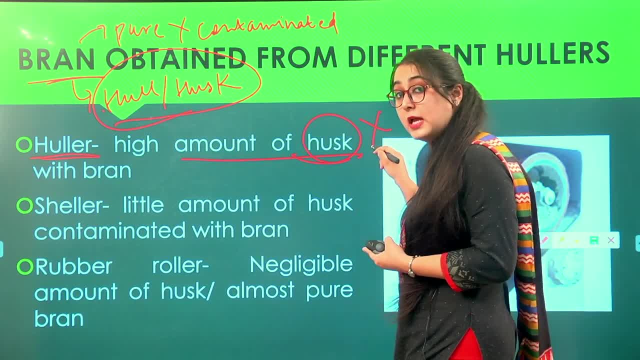 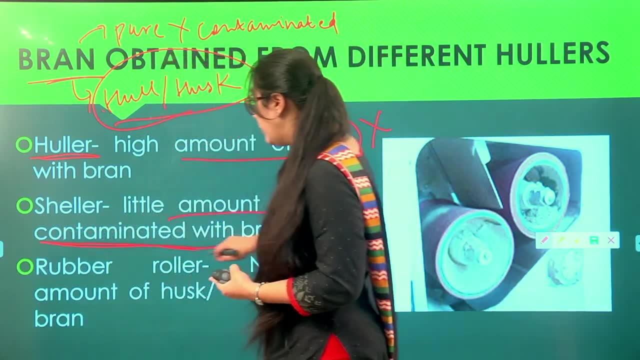 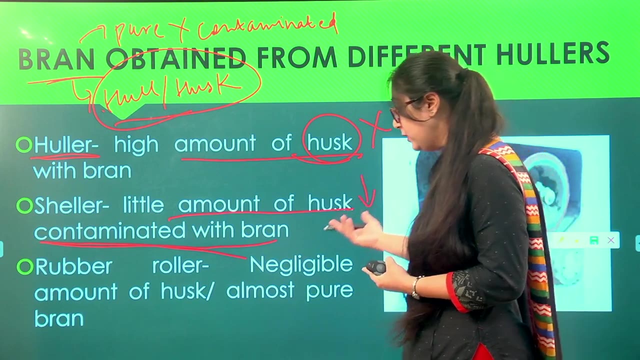 And hence it cannot be brought efficiently to use as a good byproduct. And then, if we look at certain shellers, also, Little amount of husk is contaminated with the bran. So here also we have little contamination of husk And again there will be a problem in putting it as a use as a good byproduct. 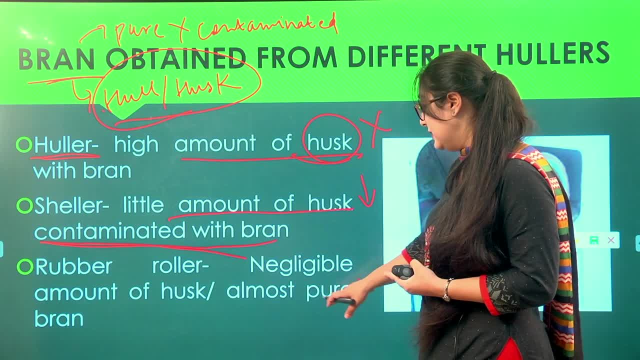 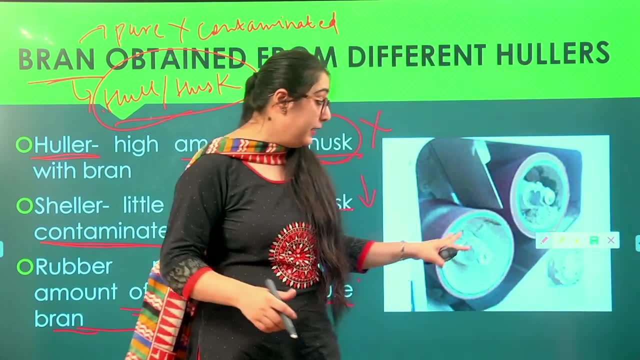 And then rubber rollers, So negligible amount of husk or almost pure bran will be obtained. So when we are utilizing the rubber rollers, Which we have discussed during the milling, As they are very, very modern And very, very good equipment for the milling of the rice, 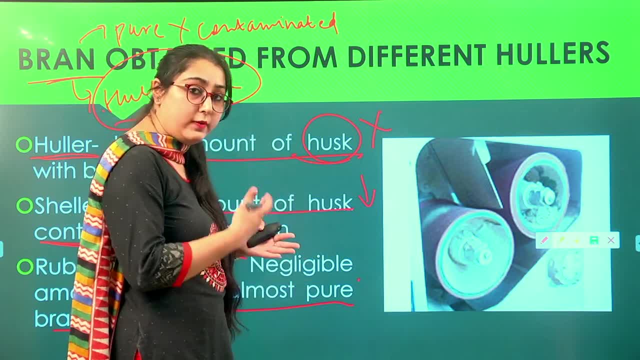 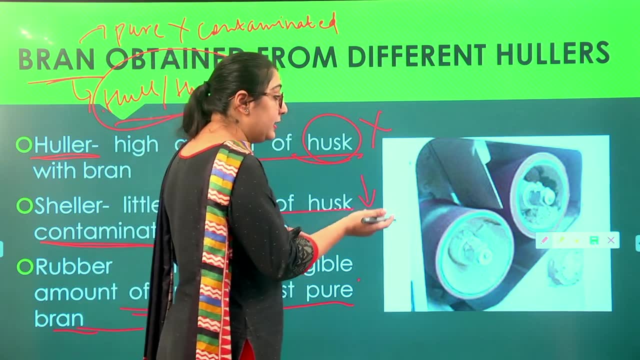 So whatever husk that they are, So whatever bran which is being produced After milling utilizing the rubber roller is almost pure And it is not contaminated with husk, Since the rubber roller removes around 90 to 95% of the huskiness. 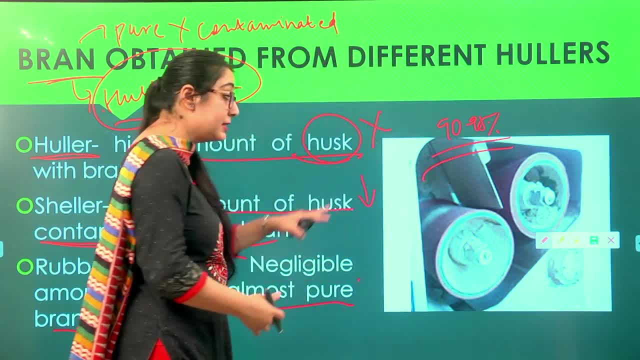 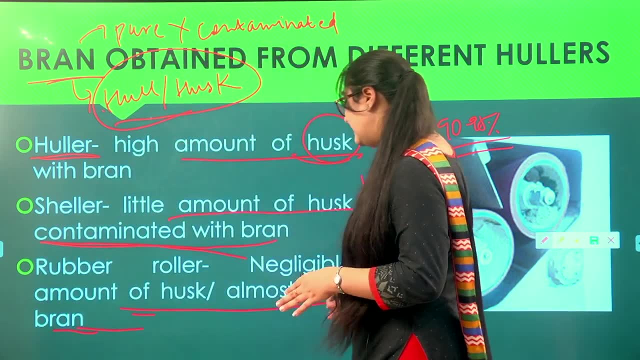 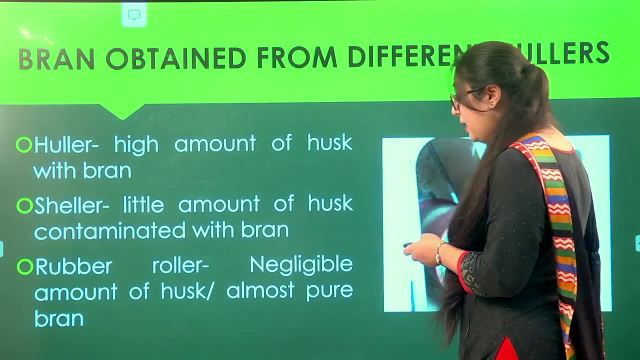 In a single pass, as we have discussed during the milling. It is very, very efficient equipment. So for the same reason the bran which we are obtaining from this Will be very, very less contaminated or almost in its pure form. So this kind of bran can be put into very, very efficiently to use as a byproduct. 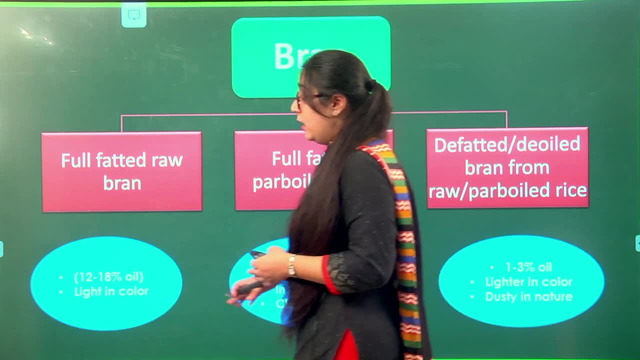 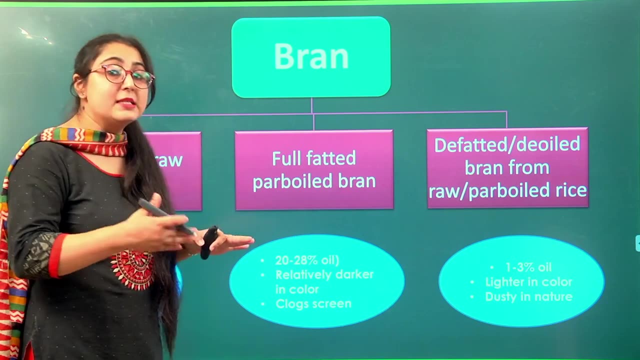 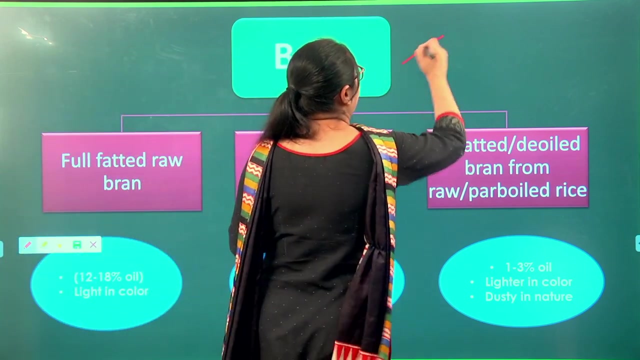 So bran. basically, when we say bran, We can think about bran in three different forms over here. So what can happen is It is divided on the basis of the oil content. So bran can be coming from. See, the bran can be coming from two kinds of rice. 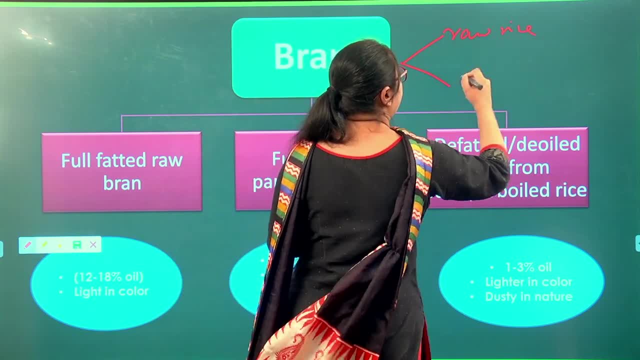 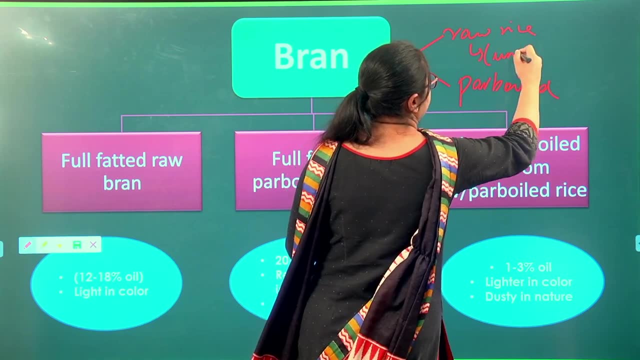 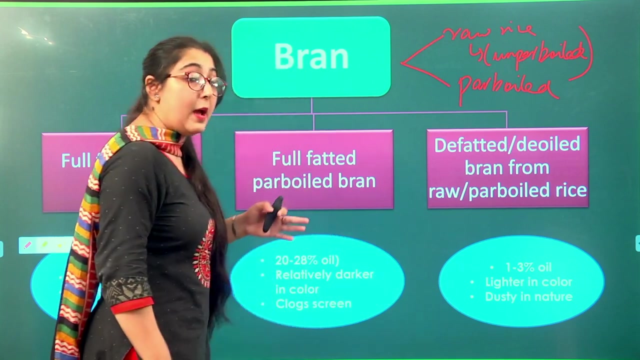 Either the raw rice or the parboiled rice. So once we say the raw rice, We basically mean unparboiled rice. Okay, So raw rice is a term utilized for unparboiled rice. So now, what happens during parboiling is. 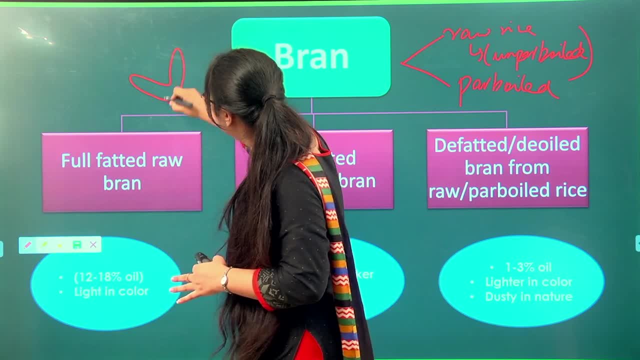 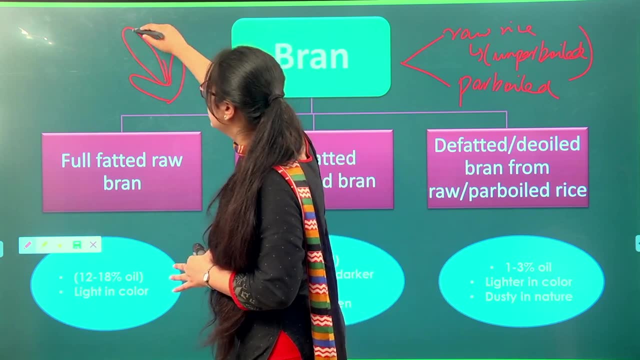 The. The rice is enclosed in the husk And it is being boiled in the husk. So what happens is The oil which is present in the outside From the husk is diffused into the endosperm. So what happens is: 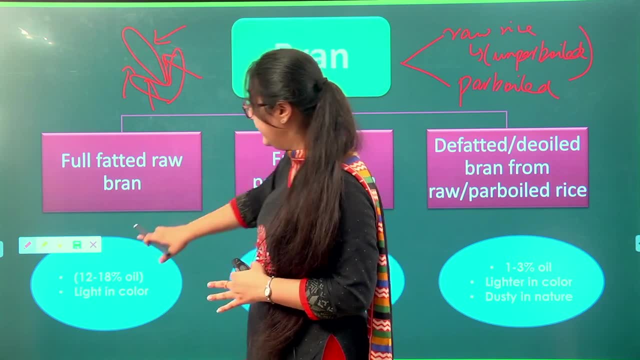 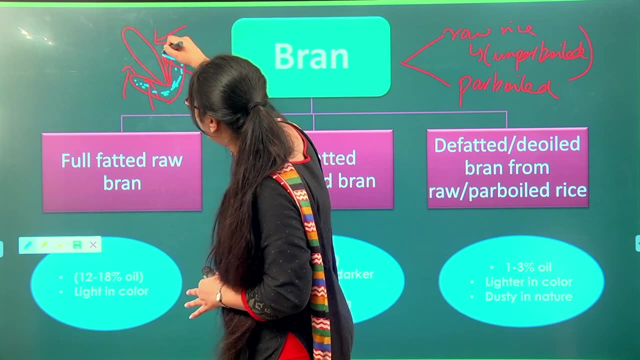 The nutritional quality of the rice increases, And not only the nutritional quality. Certain oil, pigments which are present over here, The oil which is present over here. It will diffuse along inside And it will be carried to the bran. The oil will migrate into the bran. 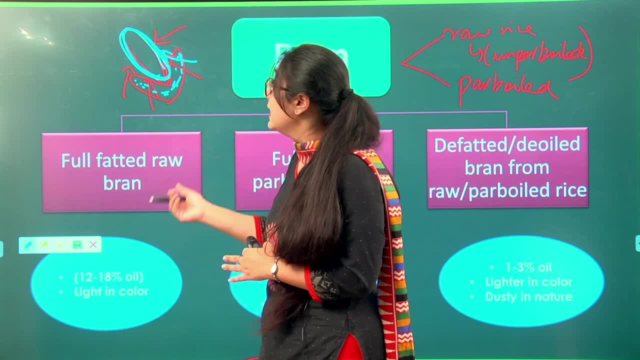 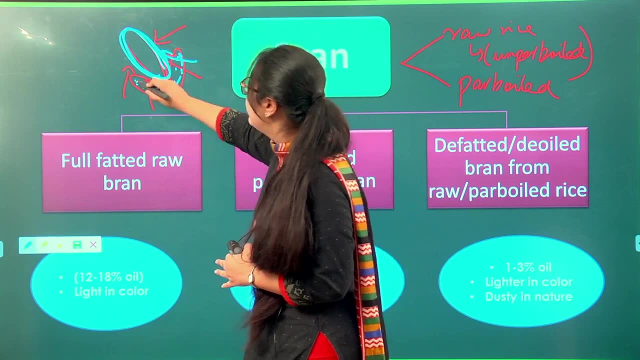 So what will happen is, In case of parboiled rice, The bran which we are obtaining Will have higher amount of oil for the same reason, Because the oil has diffused from the husk into the bran And thus the oil which was initially present in the bran has increased. 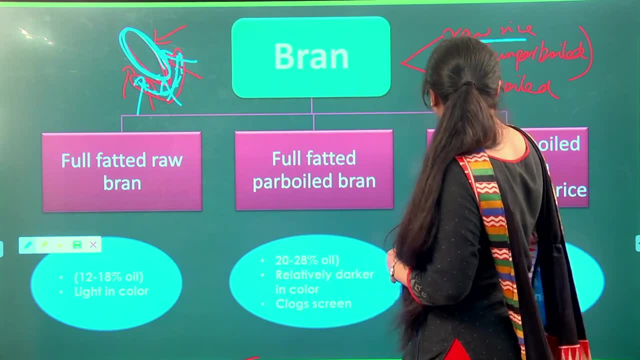 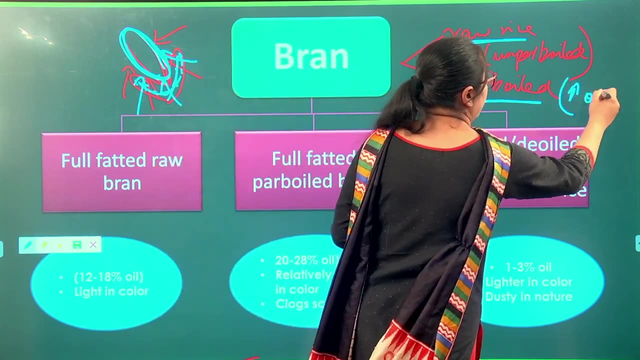 So the bran, which is present, of two types. Either the raw rice or the bran can be coming from the parboiled rice. The parboiled rice will be having a Higher oil content And the unparboiled rice will be having a low oil content. 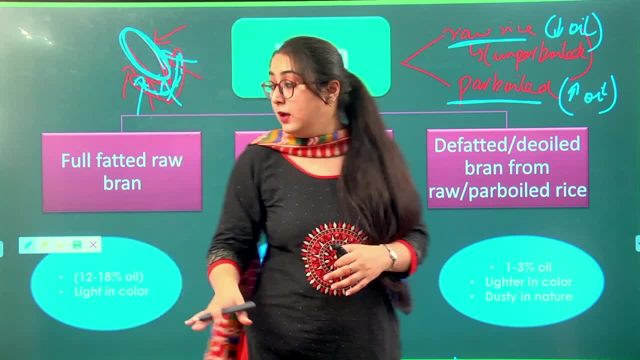 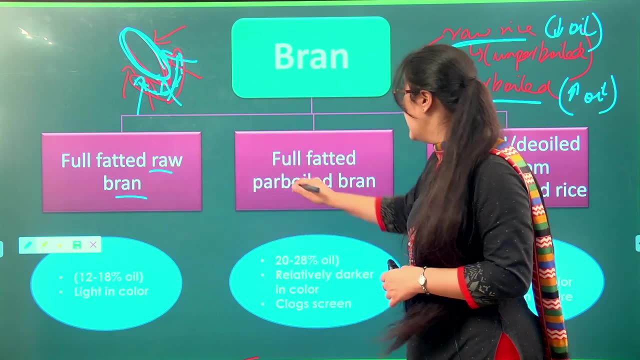 In comparison to each other. So now, if we look at them, basically, The bran can be full fattened coming from the raw bran- That is, the unparboiled rice, And the full fattened coming from the parboiled bran, That is, from the parboiled rice. 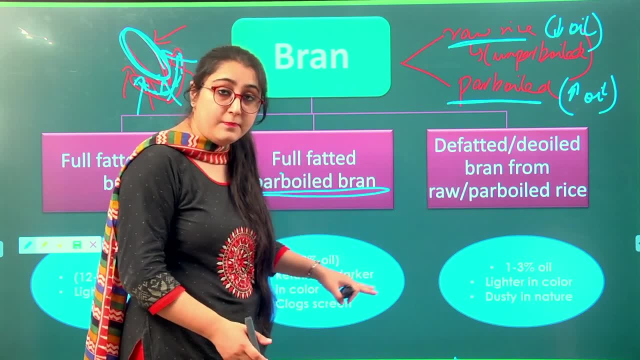 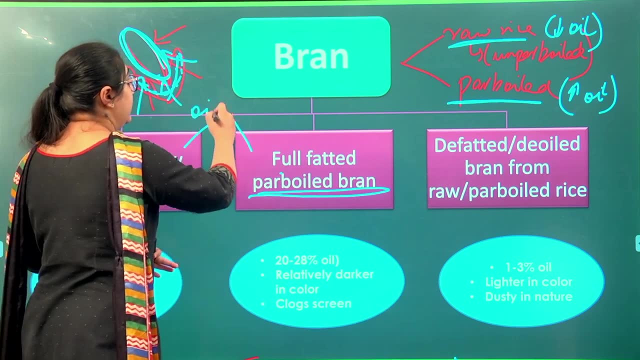 Or we can have a de-fatted or de-oiled bran That can come from both of them Once the If both of them- is utilized for oil extraction. So we have utilized oil out of it. So once we remove all the oil out of the bran, 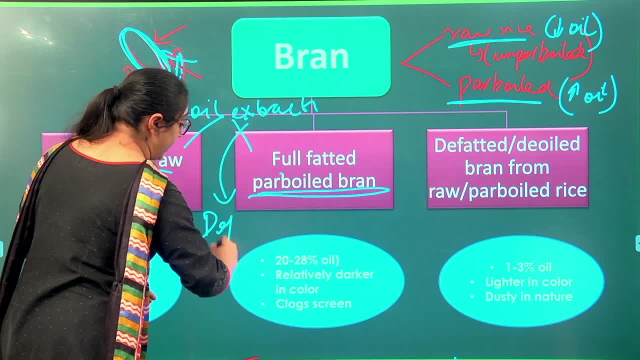 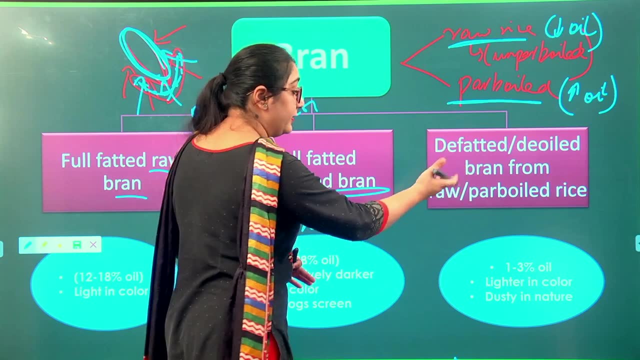 What is left is the de-fatted bran. So what we are discussing over here Is the de-fatted bran or de-fatted oil, Which is coming either from the raw rice or from the parboiled rice. It is almost one and the same thing. 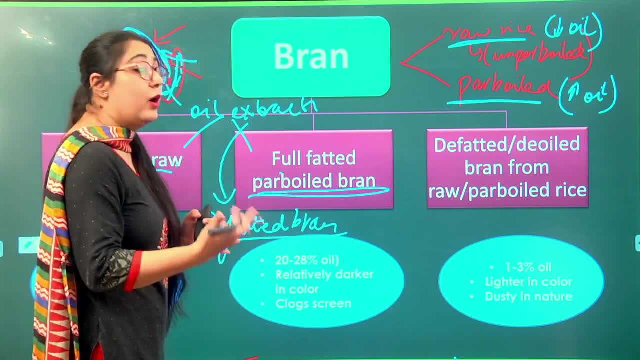 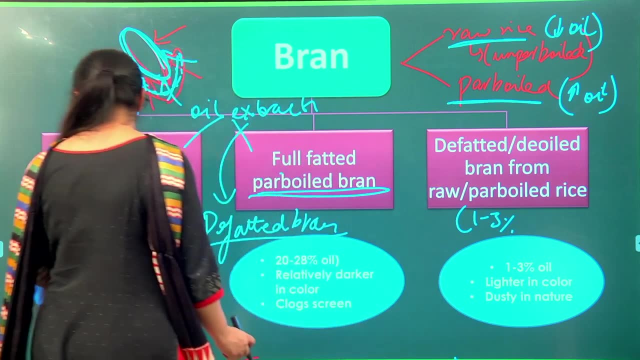 Because all the fat has been removed, Then whatever bran we are left with will contain very, very low amount of fat. That is around 1 to 2 grams. That is around 1 to 3 percent. So now, if we look at it again, 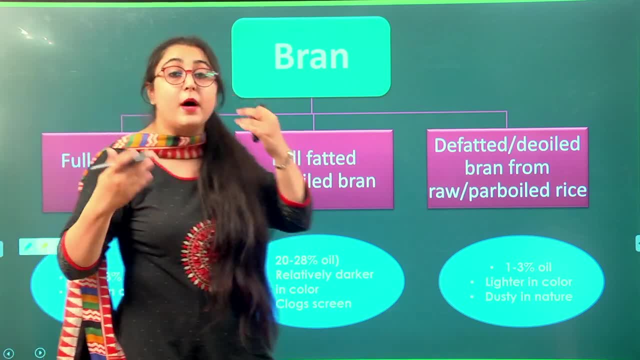 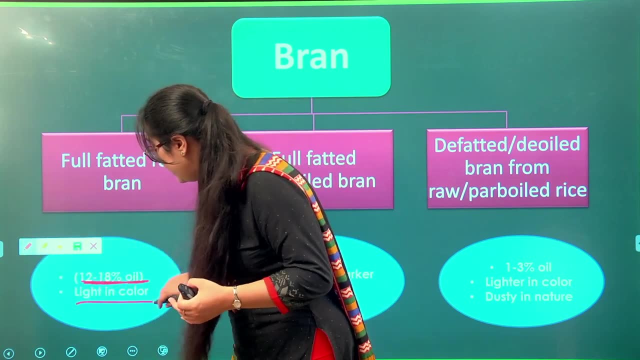 So what we have is full fatted raw bran Coming from the unparboiled rice Will contain oil. around 12 to 18 percent of the oil will be present And it will be light in color, So as the amount of oil will increase. 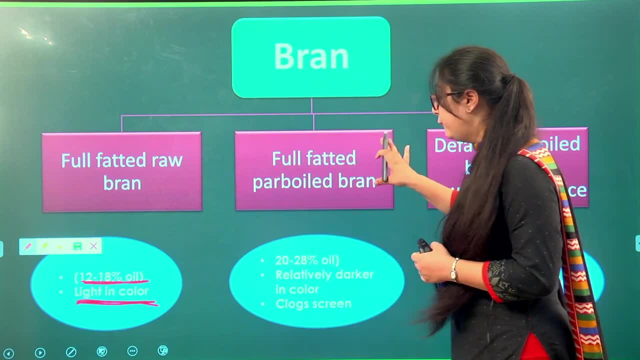 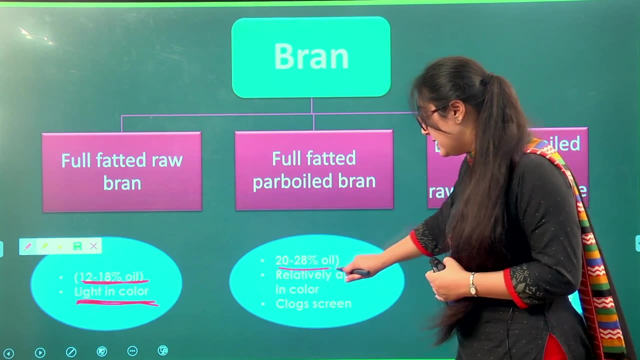 The color will also get darker. And then here the full fatted parboiled bran, Which is coming from the parboiled bran. Because it is parboiled, It will have higher oil content, So the oil present here is 20 to 28 percent. 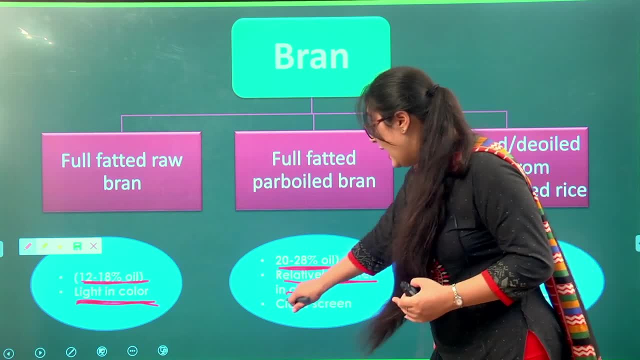 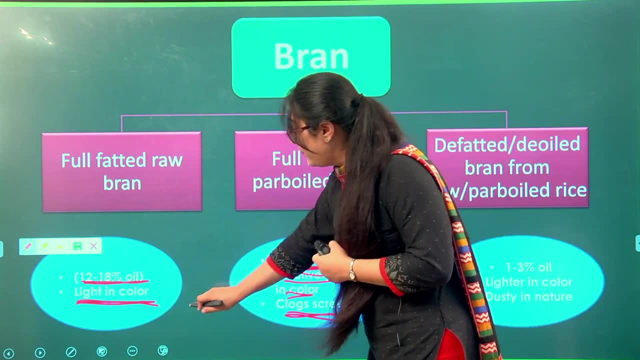 And it will be relatively darker in color And, because it has very, very high oil content, It has chances to clog the screens. So, whatever processing method or whatever we are doing, When, once we are utilizing screens for the processing, What can happen is 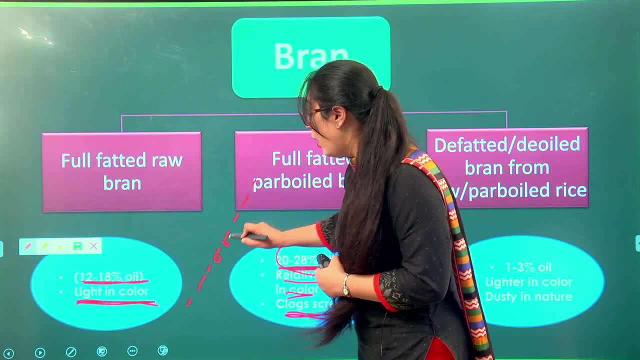 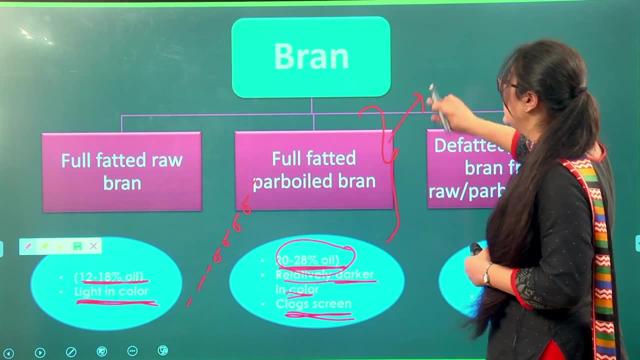 Because of its high oil, It can clog or block these screens, And this is one disadvantage When dealing with the full fat parboiled bran That what can happen is Clogging can occur in this case While processing of the bran. 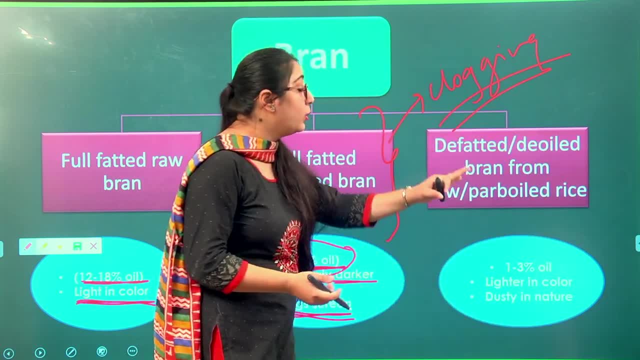 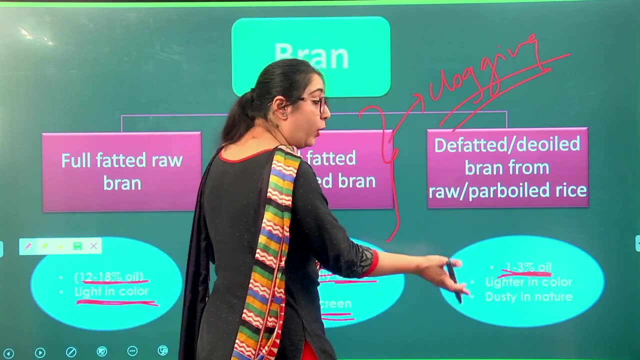 This can be a problem. Then we have the de-fatted or the de-oiled bran From the raw or the parboiled rice, Which is only 1 to 3 percent of oil, Because all the oil has been extracted out of. 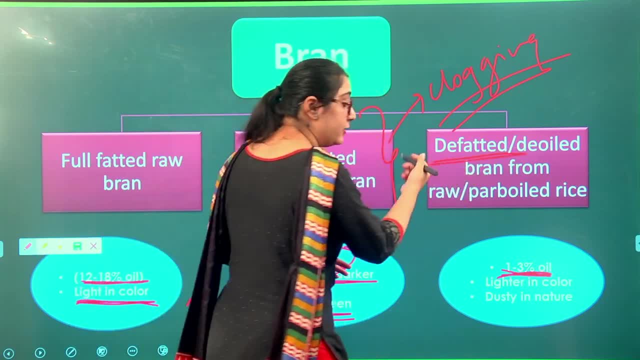 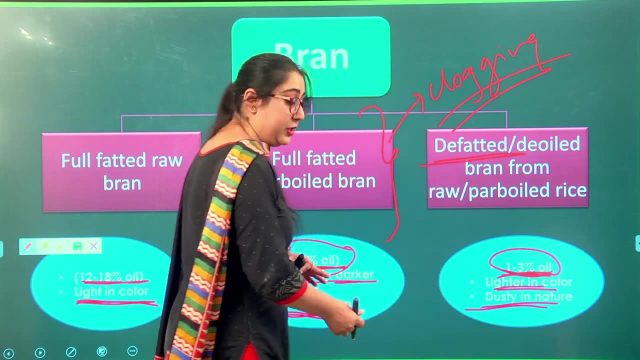 Out of both of these, when the oil is extracted, What is left is the de-fatted bran, And the oil content as a result will be very, very less. It will be lighter in color And it will be somewhat dusty in nature. So because it contains very less oil, 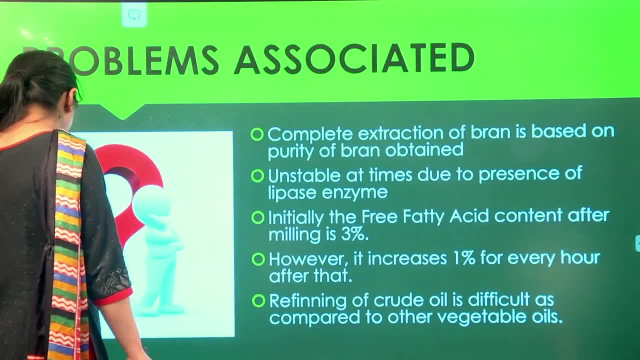 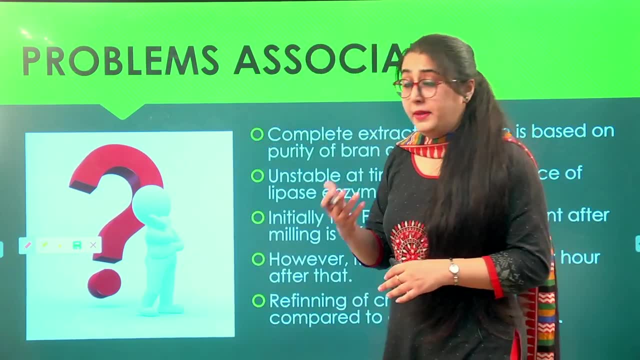 It will be lighter in color. So now, what are the problems associated with the utilization of bran? So, once we are utilizing bran, There are a number of problems which are coming. So these problems need to be looked after Because, as discussed, all these problems will hinder the 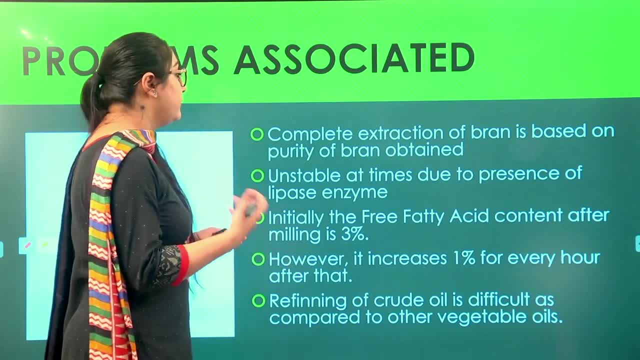 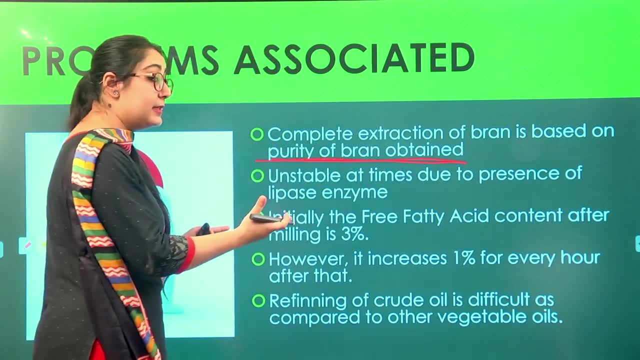 Efficient utilization of the bran as a good by-product. So first one is: the complete extraction of the bran Is purely based on the purity of the bran Right. So we have discussed it that How pure the bran is will decide Whether it can be put to use as a oil extraction. 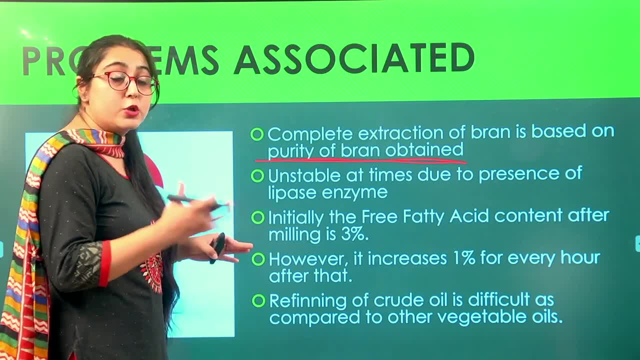 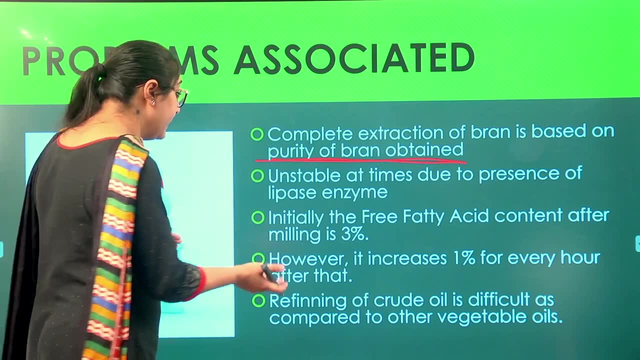 Or for certain other uses also. Whether it can be put to use So it should be pure. It should not be contaminated with the husk Or with certain other materials Such as the broken rice or the germ, And it can be unstable at time. 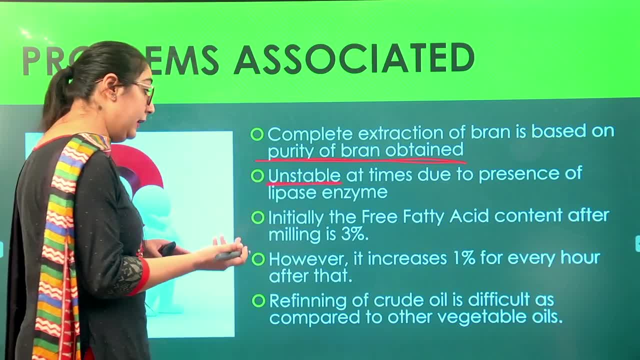 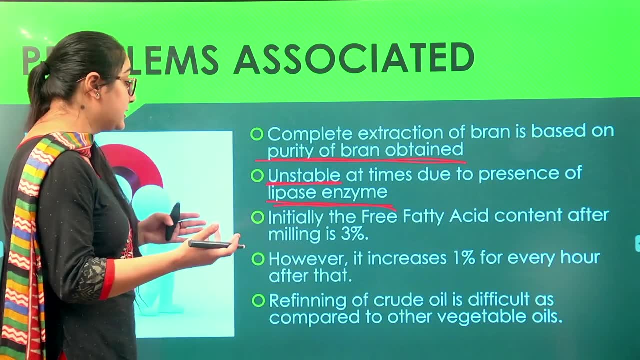 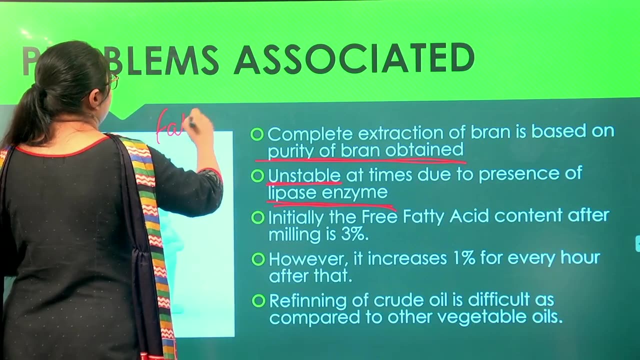 So, because the bran contains a very high amount of oil, What can happen is There is presence of lipase As well, Which can sometimes make it unstable. So what this lipase enzyme will do. So whatever are the fats in the 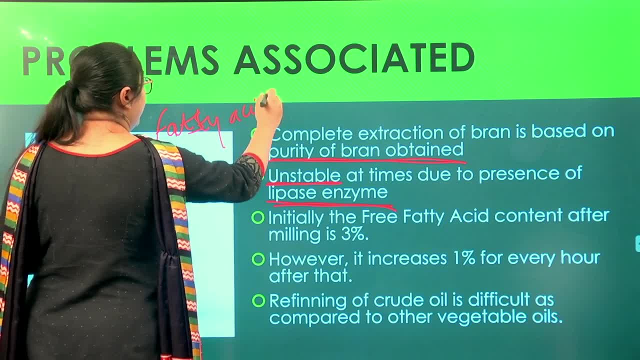 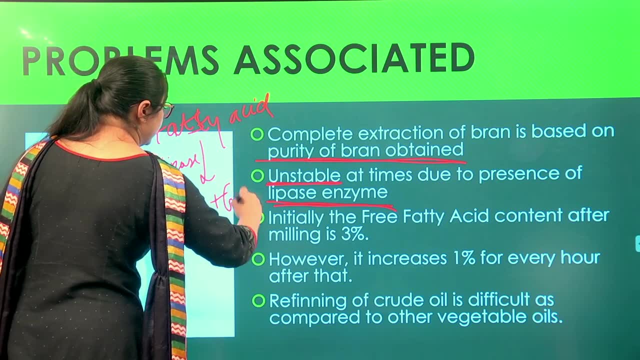 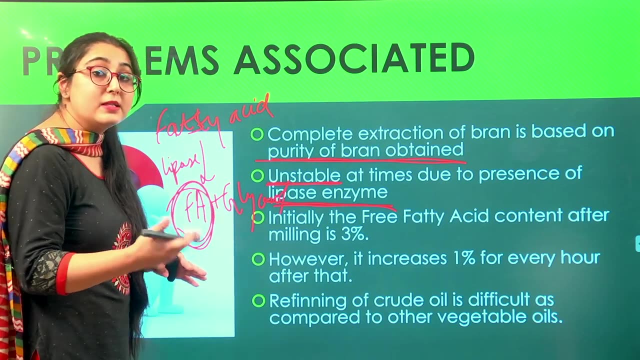 Whatever the fatty acids we have, They can be broken down. Because of the lipase enzyme, They can be broken down into fatty acids And glycerol. So this is undesirable. Once these fatty acids It will be broken down, It will give an undesired odor. 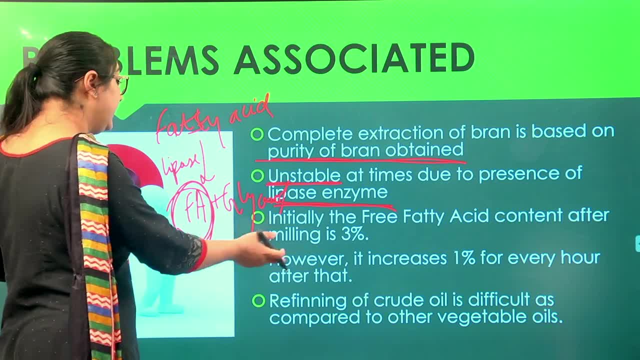 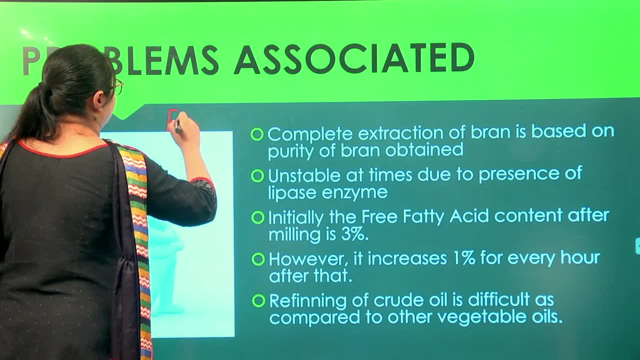 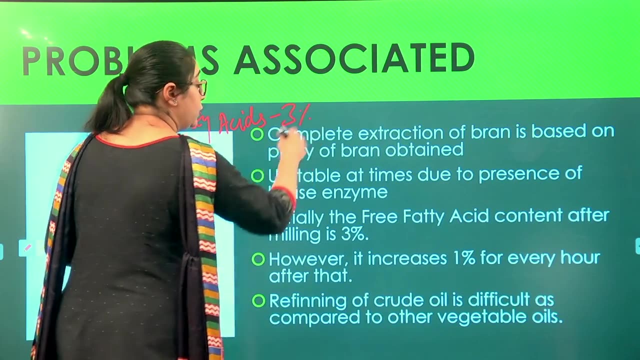 Undesired taste as well. So, initially, the free fatty acids content. So basically, We have fatty acids Okay, Which are only around 3%, But what will happen is Because of this presence of lipase enzyme And certain other reasons. 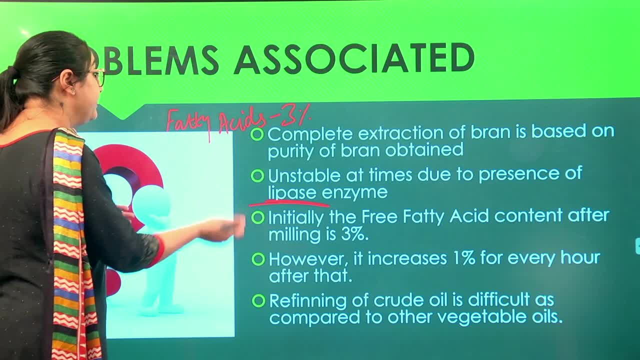 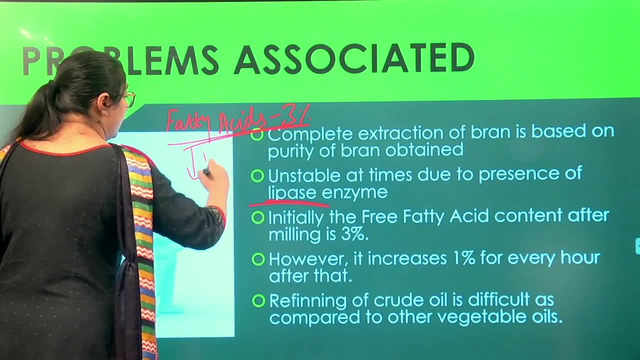 The rice bran is very, very unstable And after milling The free fatty acid content Can keep on increasing every hour. So initially The fatty acid content is 3%, But one hour after that, If it is kept After milling, It has been removed from the rice. 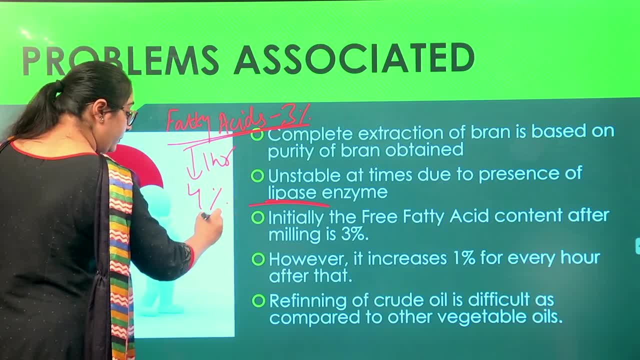 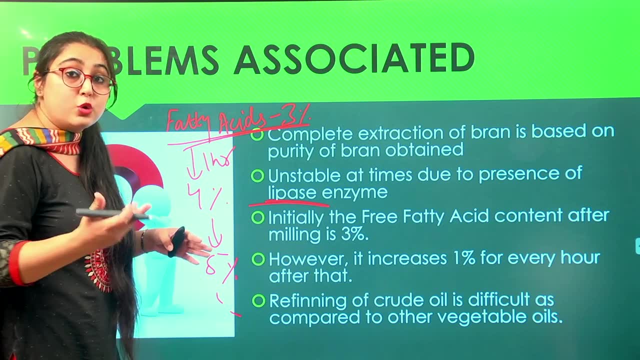 Then it is kept, The free fatty acid become, Will become 4%, After that The free fatty acid will become 5%, And so on. Every hour it will keep on increasing. So the free fatty acid content Is increasing at a very, very high rate. 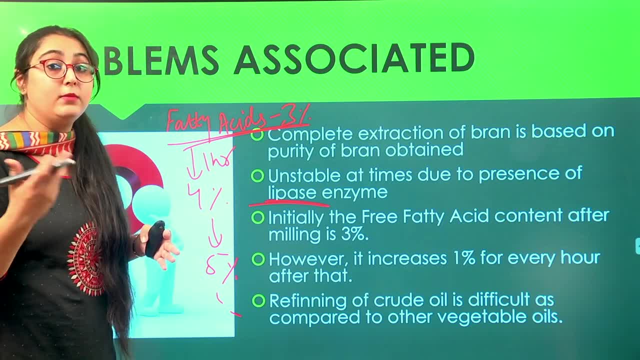 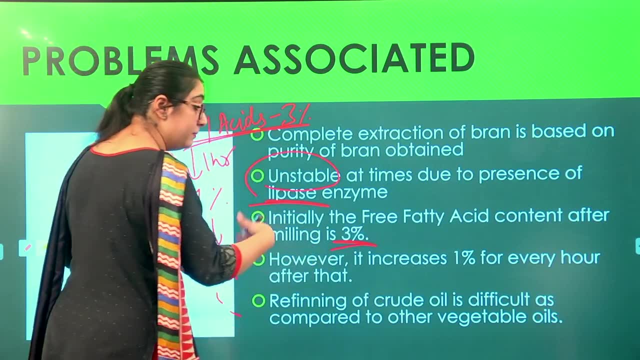 Which is going to limit The uses the bran can be put into. So because of these reasons, It is very, very unstable And initial free fatty acid content Is only around 3%, But it is going to increase Every hour after that. 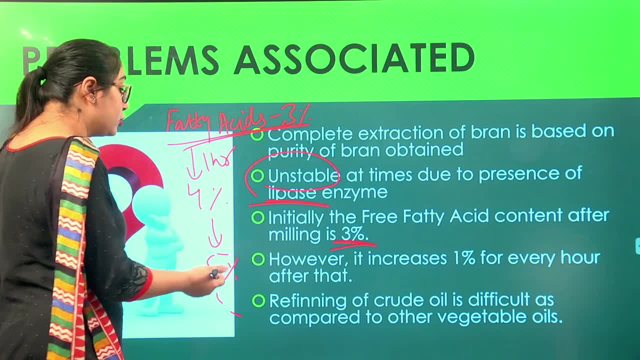 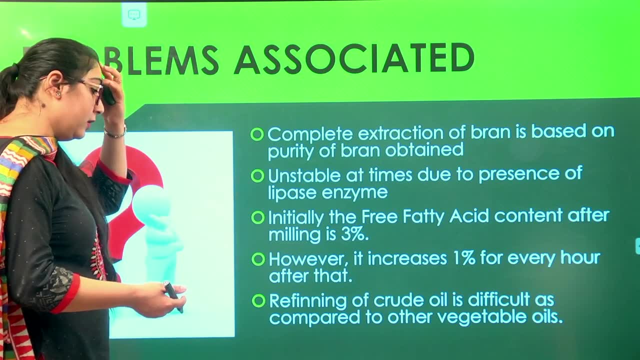 Once it has been removed from the rice During the milling, So even during the refining Of the crude oil is difficult As compared to other vegetable oils. So once we will discuss The oil extraction process, This point will be clear to you. 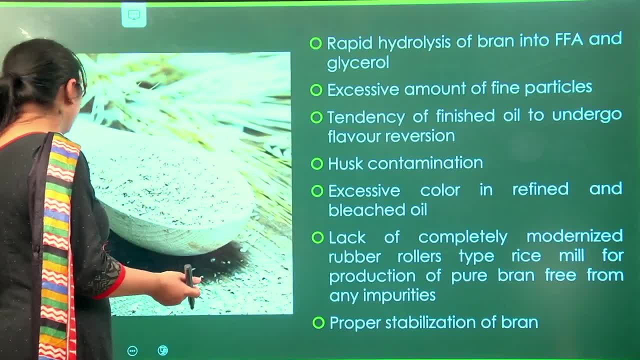 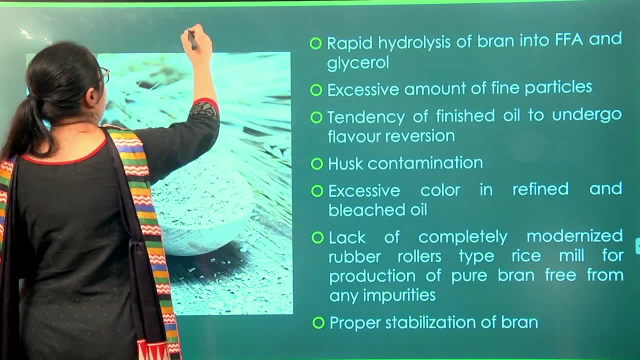 So also more reasons, More problems, which are Rapid hydrolysis of the bran Into free fatty acids And glycerol, As we had discussed That what can happen is Because of the presence Of the lipase enzyme. It can be. 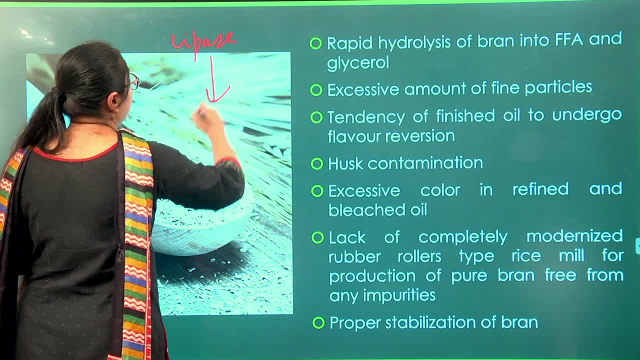 The fat can be broken down Into the free fatty acids As well as Glycerol, Which is very, very undesirable. So hydrolysis of the fat Is occurring Because of lipase enzyme Or water Or certain other reasons. 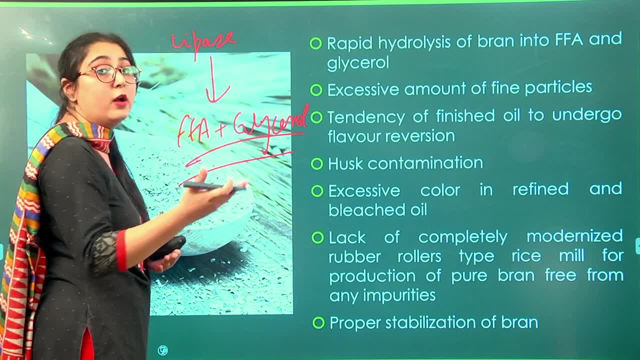 And it is converted Into the free fatty acids And the glycerol, Which is not desirable Excessive amount of fine particles. So sometime, A lot of time, It is going to increase Because of the presence Of the lipase enzyme. 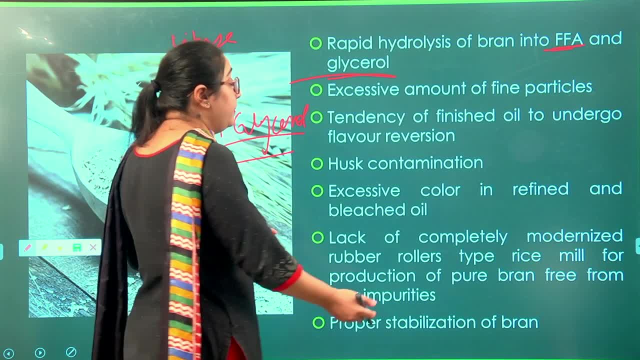 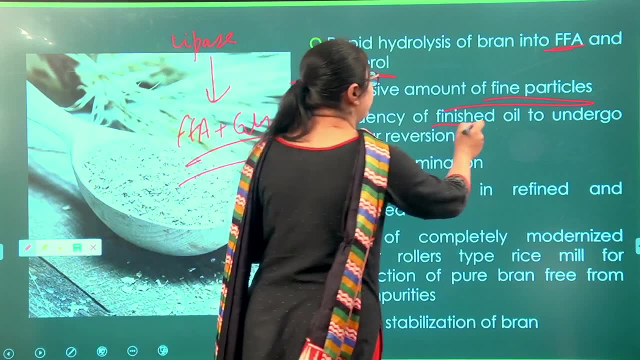 It can be. The fat can be broken down Into the free fatty acids, So sometime A lot of fine particles Can be present In the bran, Which is again Undesirable, And then Tendency Of the finished oil. 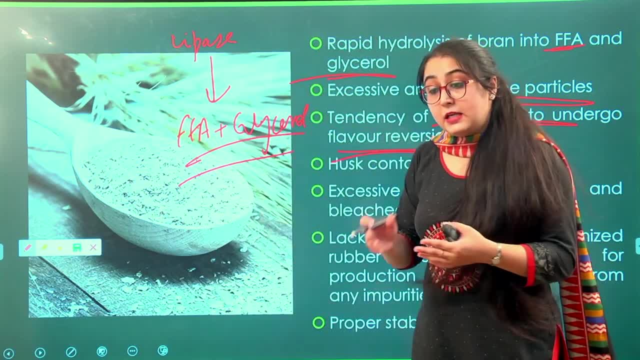 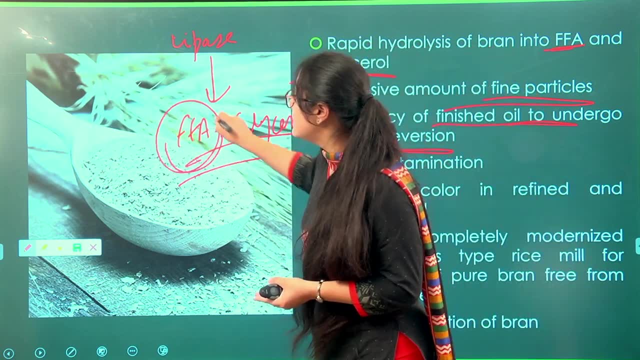 To undergo Flavor reversion. So even After the oil Is, Even after the oil Is removed From all the undesirable Free fatty acids Which are giving the See, these Free fatty acids Will be responsible For giving a bad. 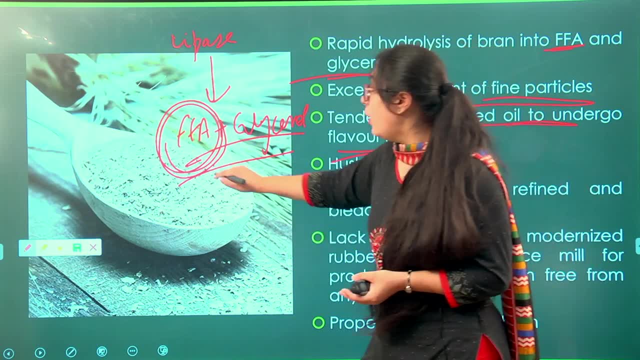 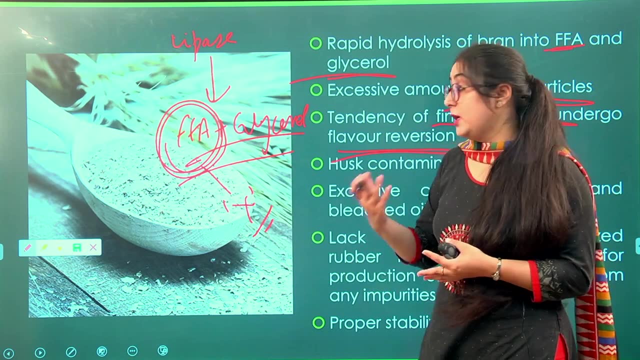 Odor, Bad taste. So during The refining Process Of the oil We will be removing Its flavor And taste. But what can happen In case of rice bran oil Is, even After the refining, The flavor. 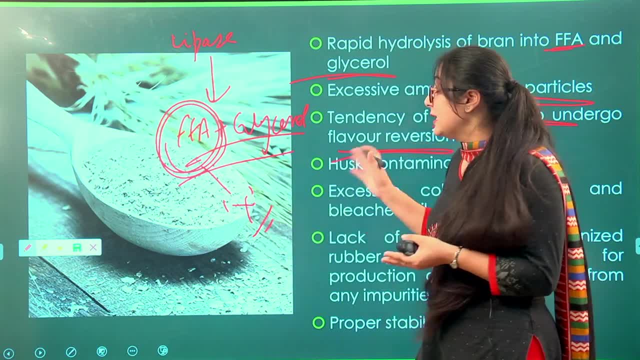 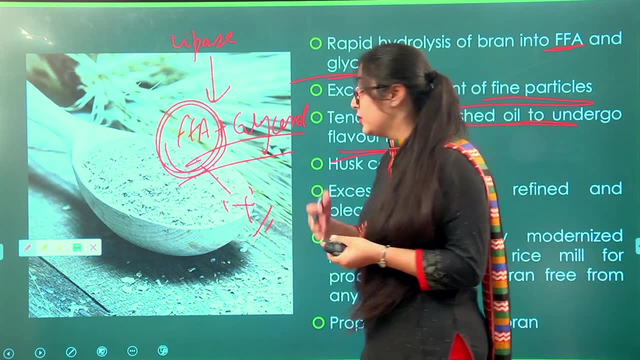 Has been improved During the refining, That flavor reversion Can happen. The rice Can go back To the Same flavor From which The flavoring Substances Which we have removed. And because of that Flavor reversion, 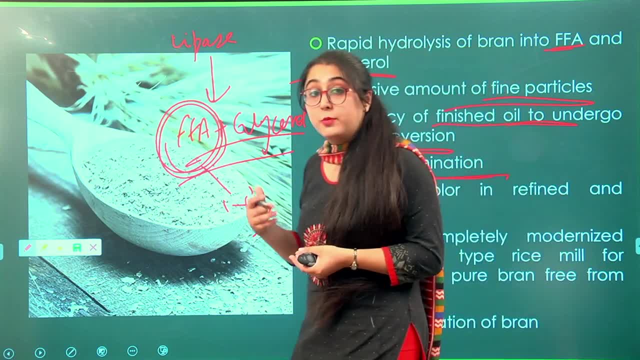 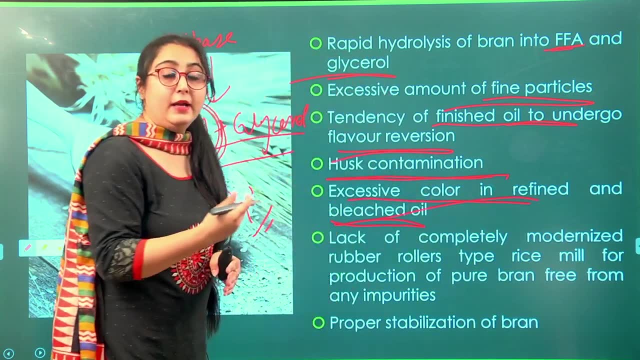 Is occurring, Which is again Undesirable, And it can be contaminated With the husk, As discussed. That is also. One major Problem Is The rice bran, Because of The bran Is brown In color. 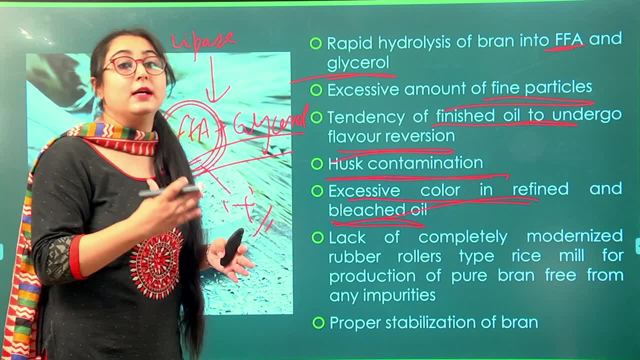 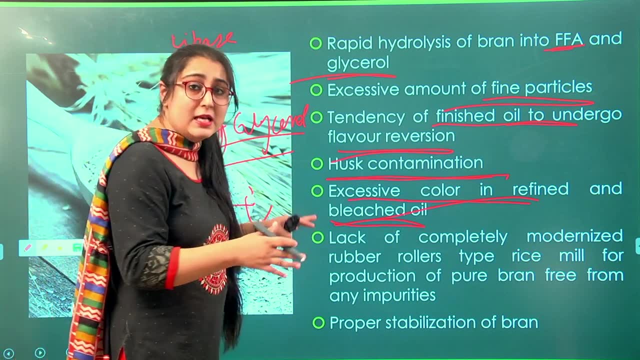 Right. So what happens Is the oil Which is produced From the rice Bran oil Is not As light In color As being produced From other Vegetable Oil. So the oil That we use At home, 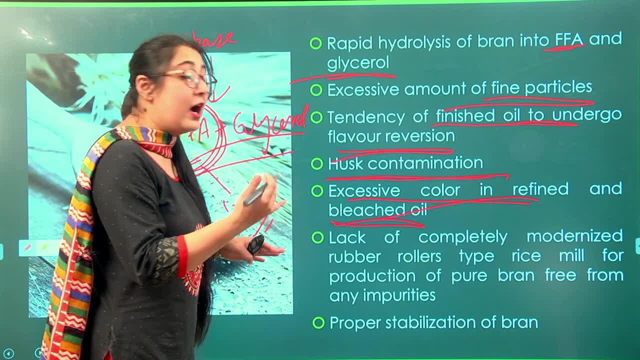 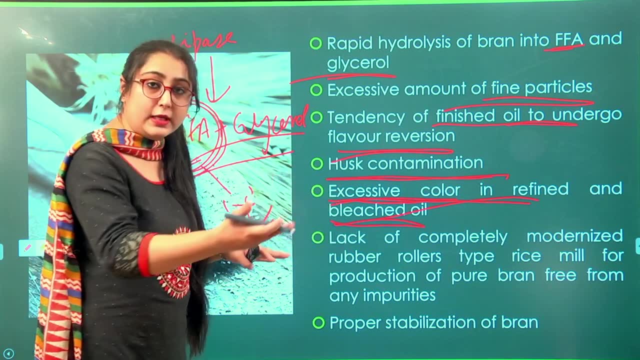 Obtained From certain Vegetable Oils, Such as Sunflower, And then From other Vegetable Oils, And This refining And the bleaching We will be looking at During the oil Extraction Or 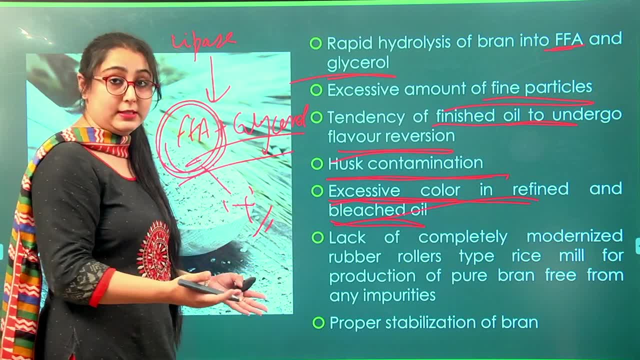 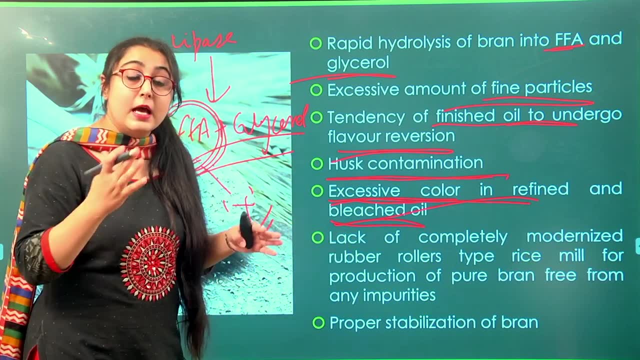 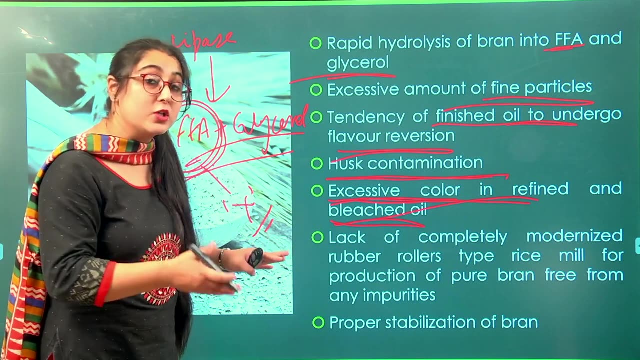 What these steps Are. Lack of Completely Modernized Rubber roller Type Rice Mills For the production Of pure Bran, Free From any impurities. So just, We have already Discussed Previously. 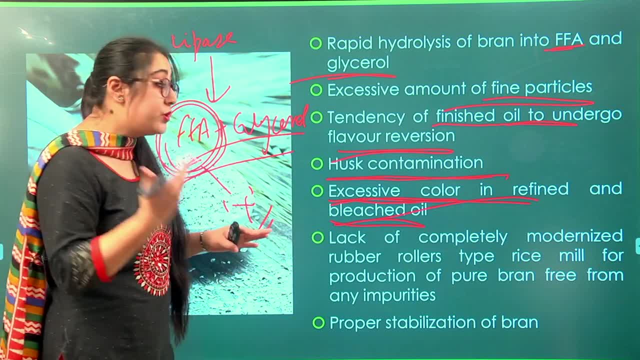 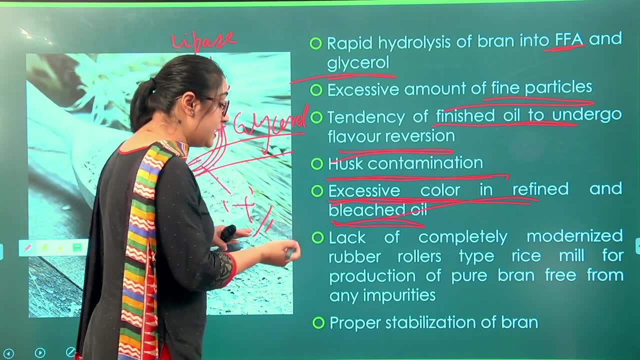 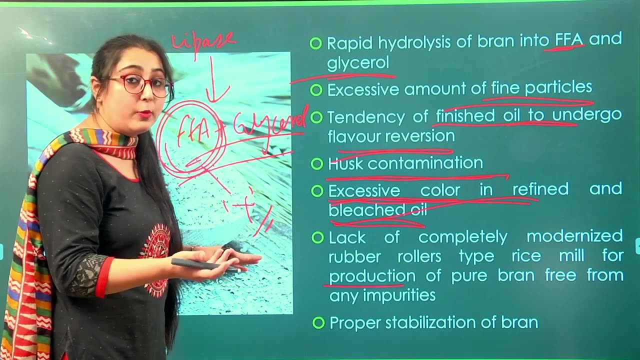 That There are A number Of farmers, A number Of industries Which are Still Dealing With the Hullers Or Shellers, All of this Because Of which The bran Can be. 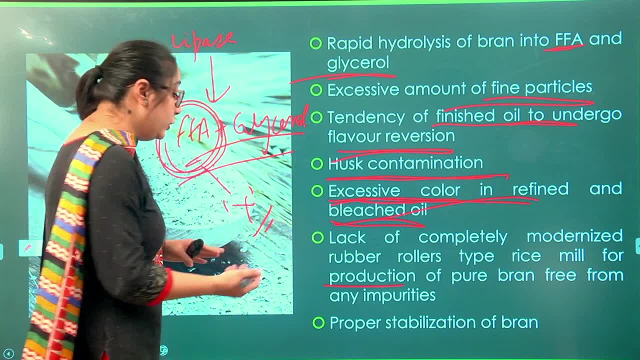 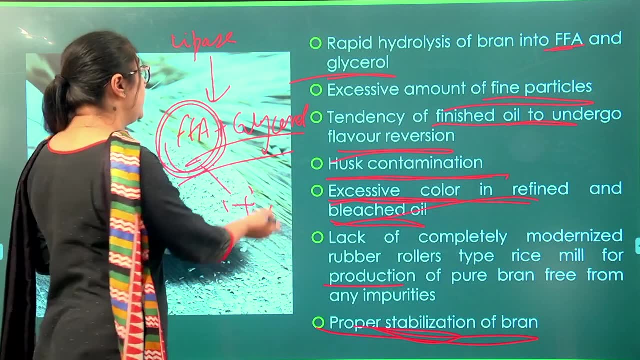 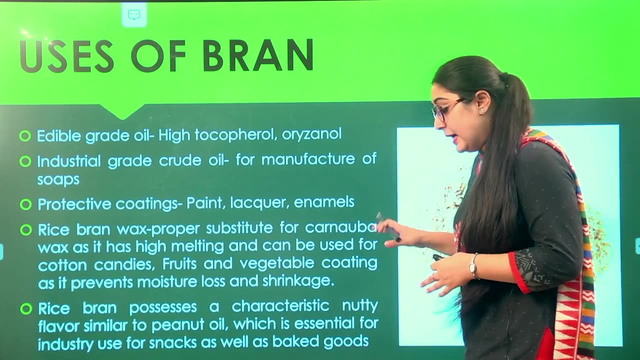 Contaminated And Because Of the same Reason, It can Not Be Put To Proper Utilization, And Certain Other Reasons. So Now, Going On To The Uses, 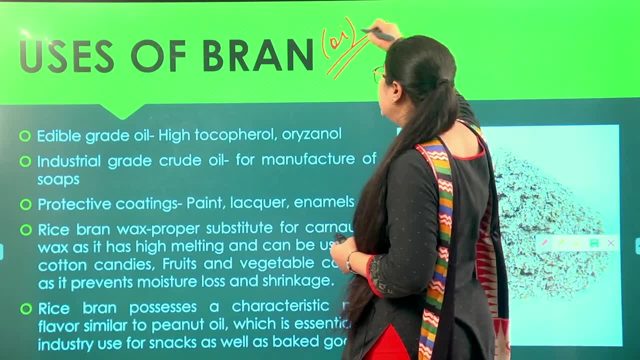 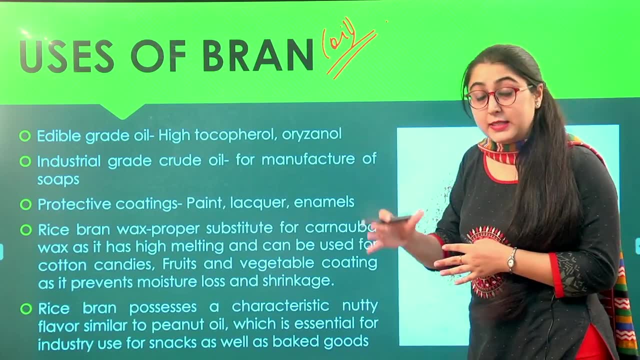 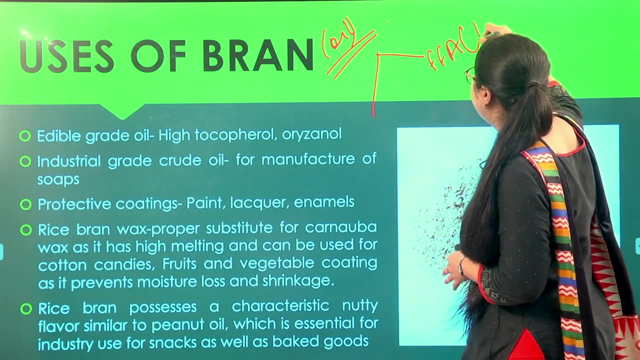 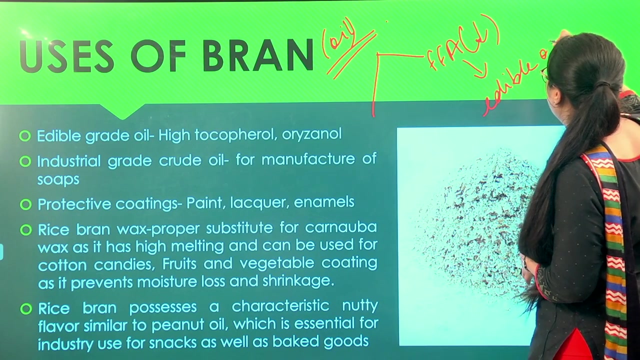 Of The Bran. Now, The Use Of The Bran Will Obviously Depend On Its Purity, And The Bran Has High Free Fatty Acid Content. It 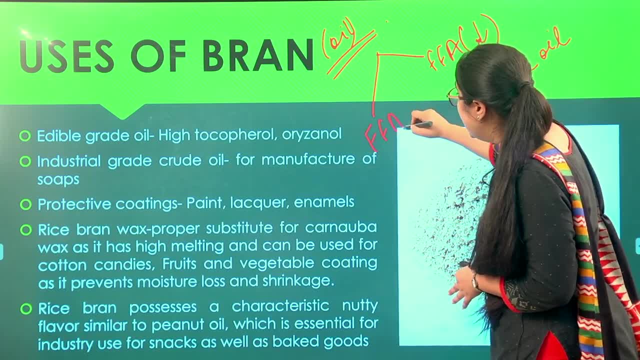 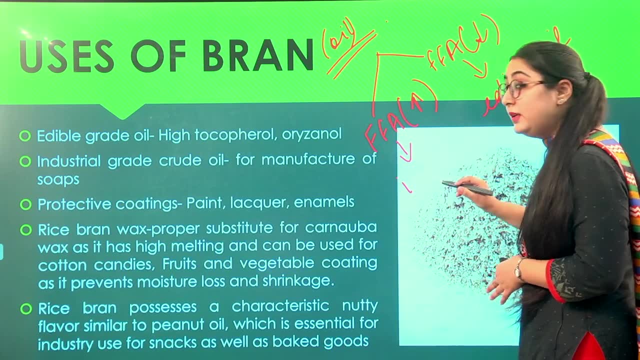 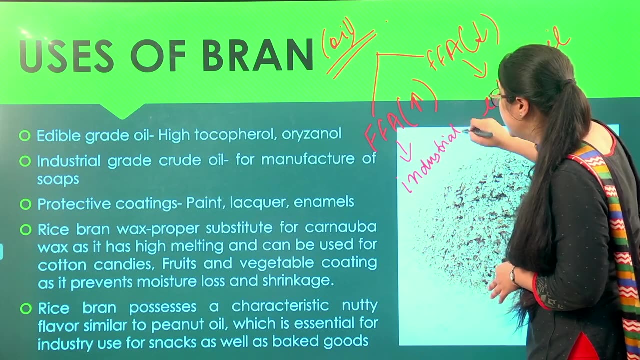 Can Be Very Easily Utilized To Produce Edible Oil. But On The Other Hand, If We Have Bran Which Has High Free Fatty Acid, 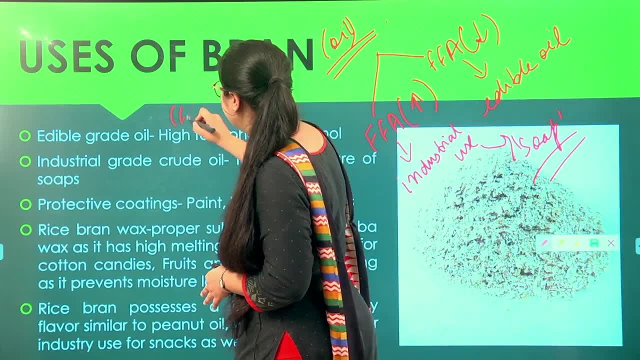 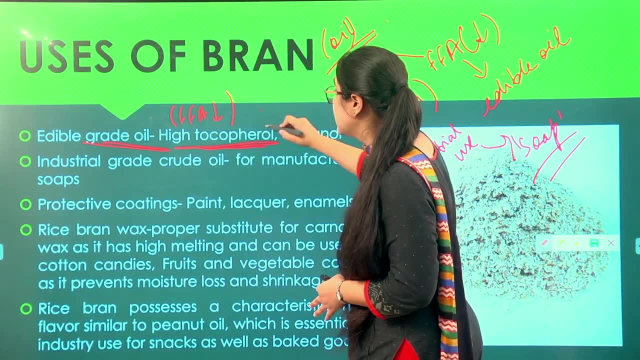 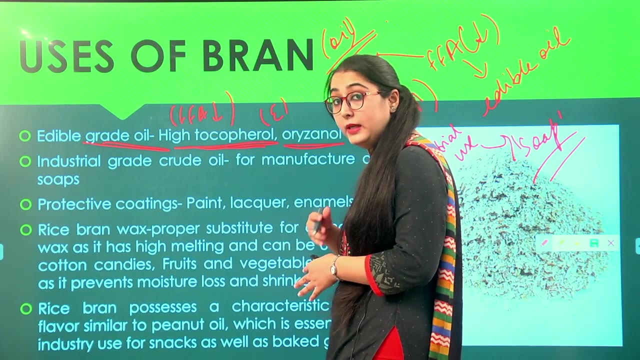 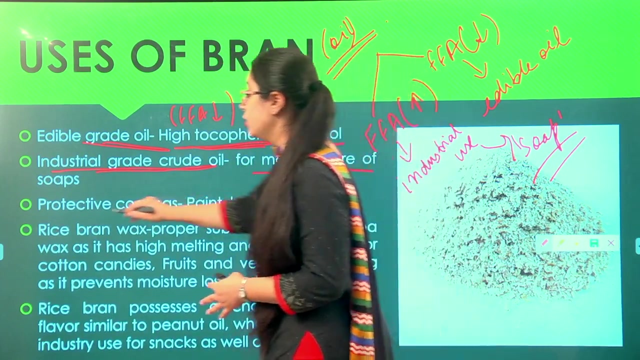 Soap Manufacturing. So If The Free Fatty Acid Content Of The Rice Is Very, Very Low, We Are Going To Make Edible Grade Oil In. 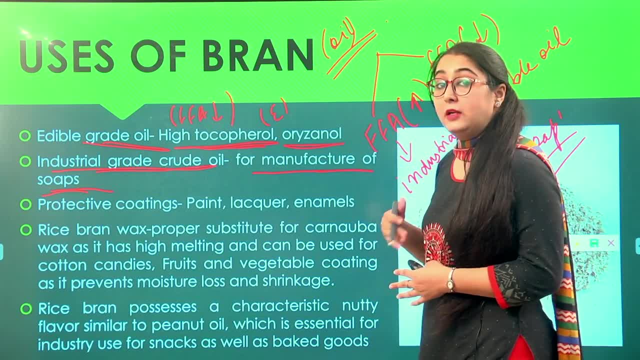 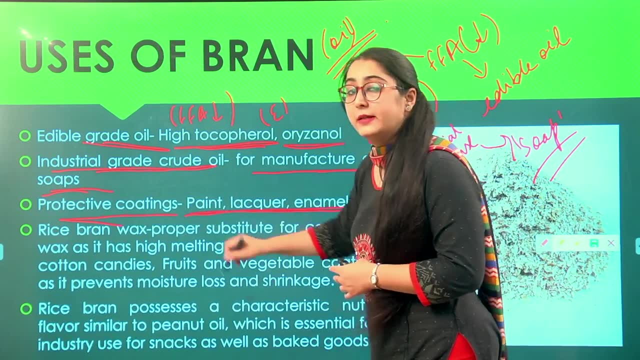 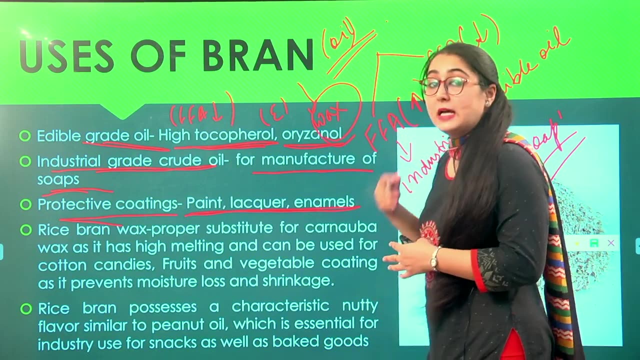 It, And It Can Be Made To, Can Be Used To Make Protective Coatings, And Thus It Is Utilized In Paint, Lacquer And Certain. 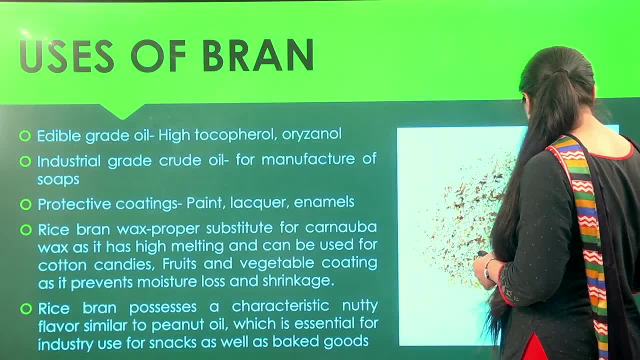 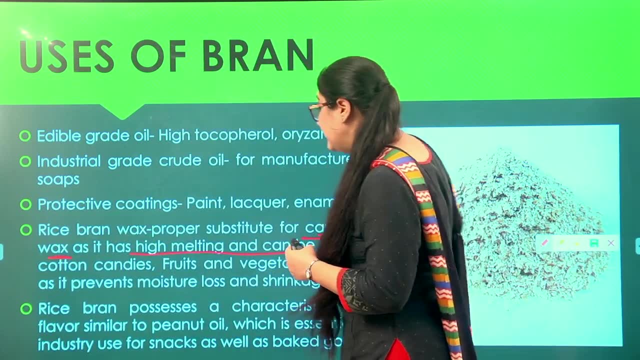 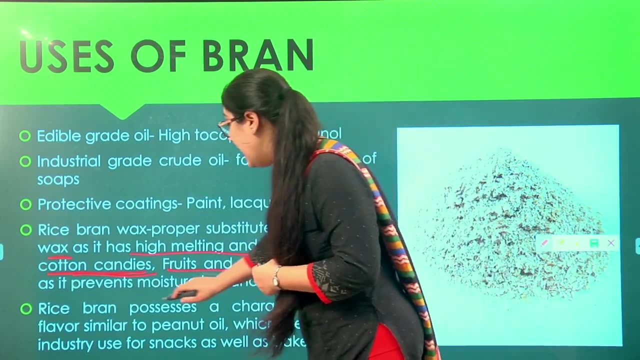 Other Enamels As Well. As We Know Wax Because Of Its Very High Melting Point, And It Can Be Utilized In Cotton Candies. 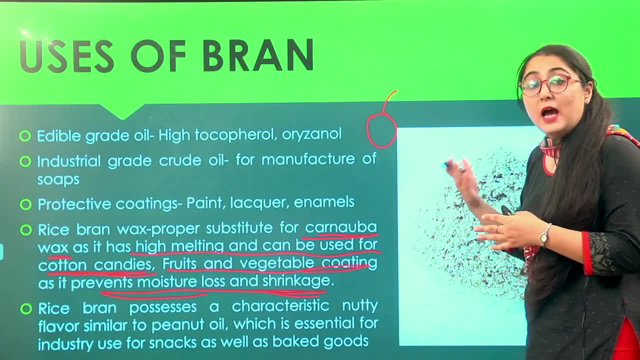 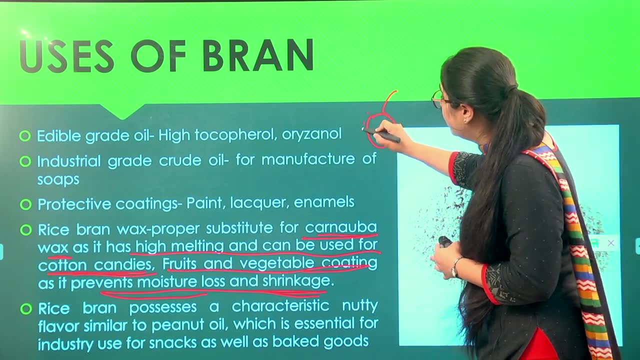 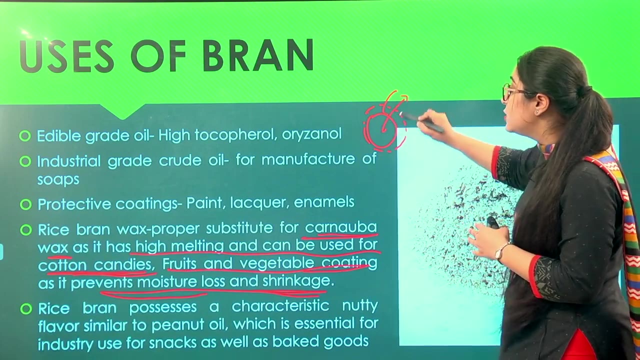 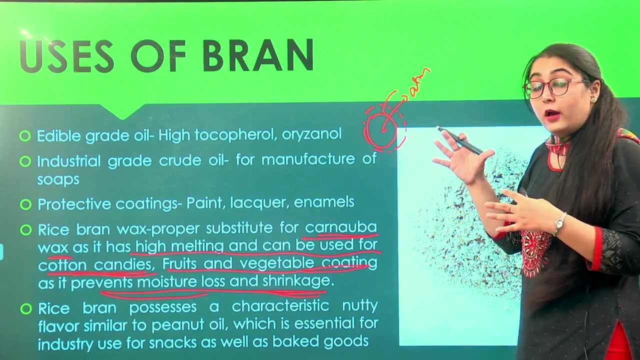 As Well. It Is Being Utilized Even For The Coatings Of The Fruit. It Is Going To Have A Barrier And It Is Going To 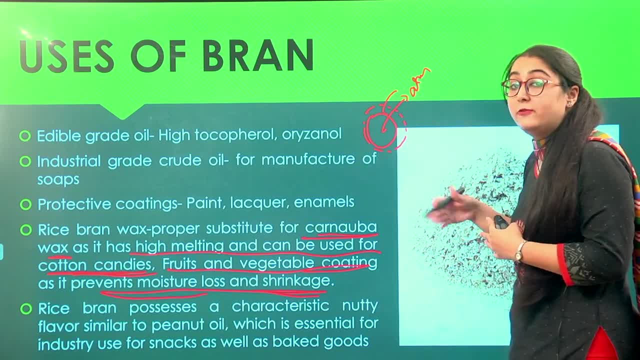 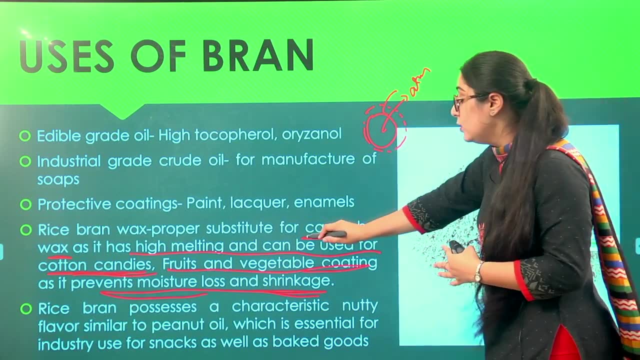 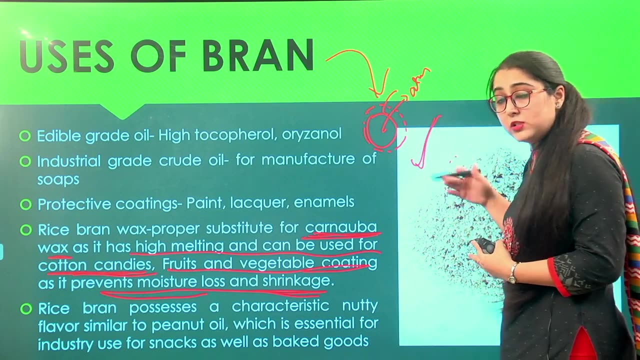 Prevent The Loss Of Moisture From The Food To The Atmosphere So, As A Result, The Fruit And Vegetables, To Preserve Them For Longer. 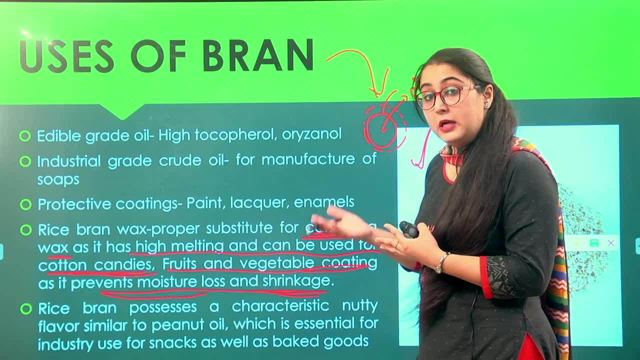 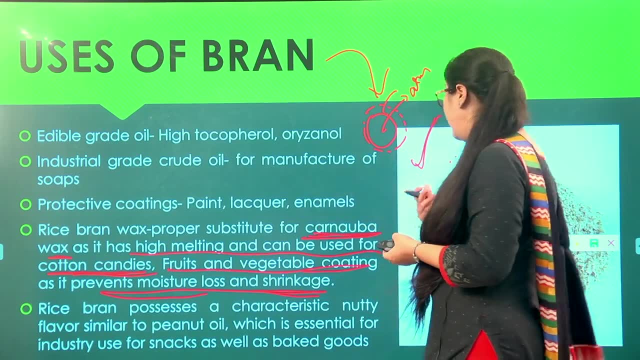 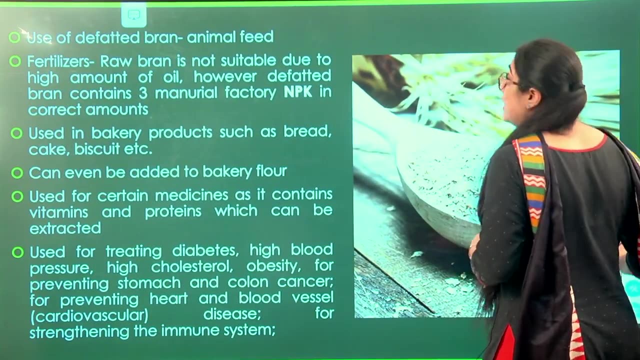 Time Rice Bran Possesses A Characteristic Nutty Flavor Which Is Similar To Peanut Oil. It Also Has A Very Good Nutty Flavor, Just The. 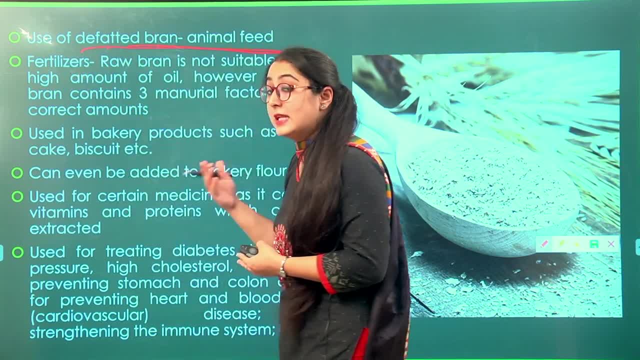 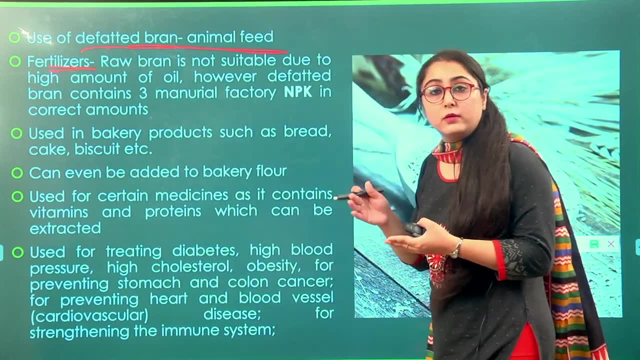 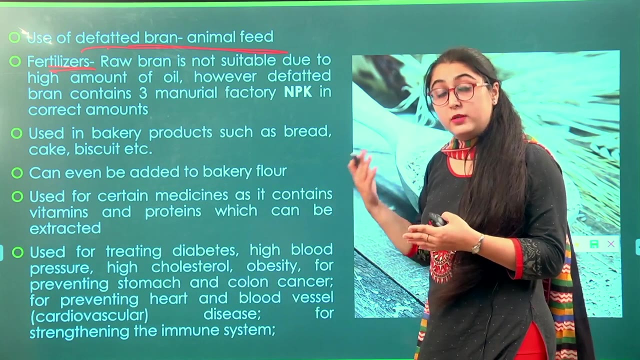 Fat Has Been Removed Can Be Utilized To Make As An Animal Feed. It Can Be Given To The Animals As A Food And Then 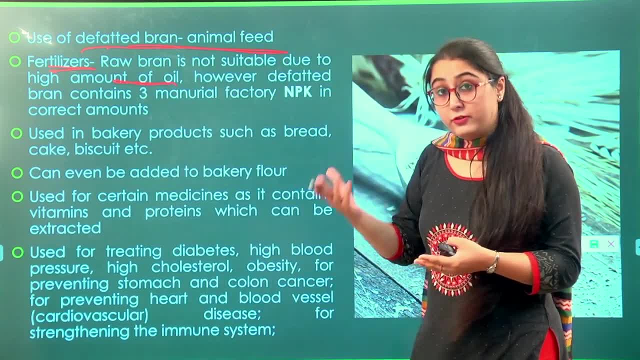 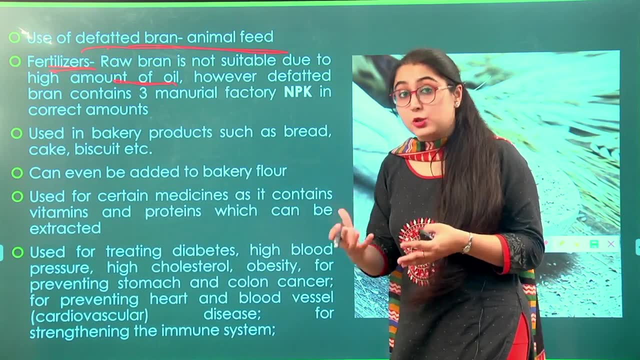 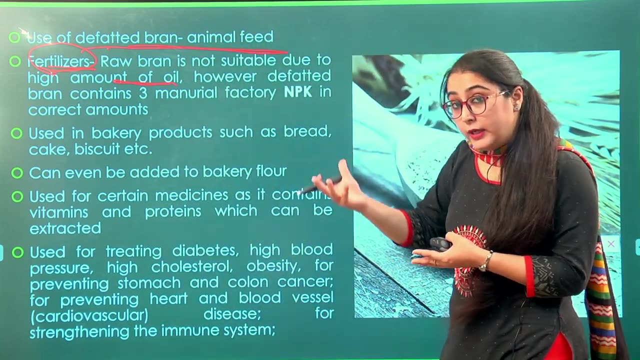 Even In Fertilizers. So Since The Oil Extraction Has Already Been Done From It, Even The Leftover Solid, Solid Meal Or The Cake Does. 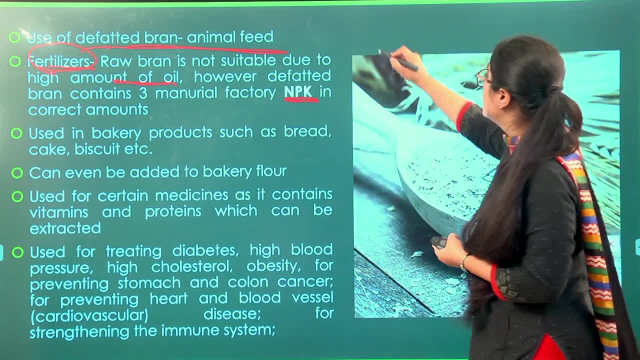 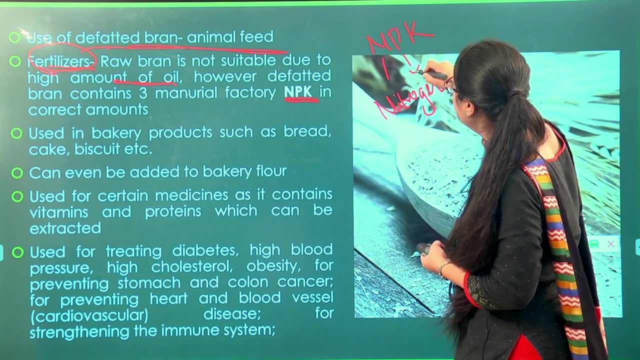 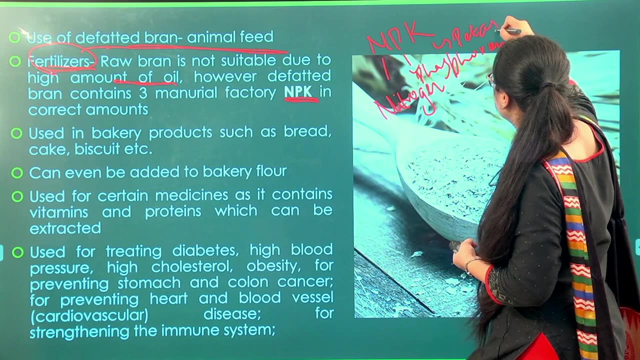 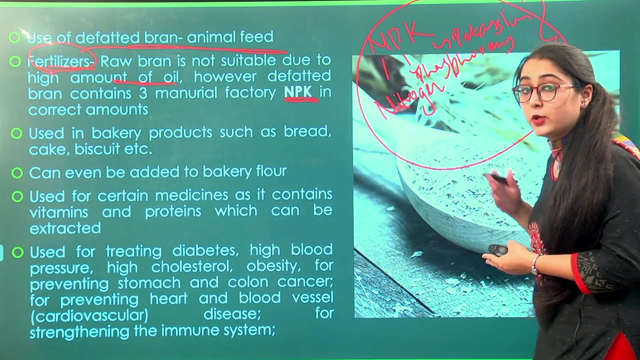 Not Go Waste. It Can Also Be Utilized As An Animal To Make As An Food. It Can Be Given To The Animals It Can. 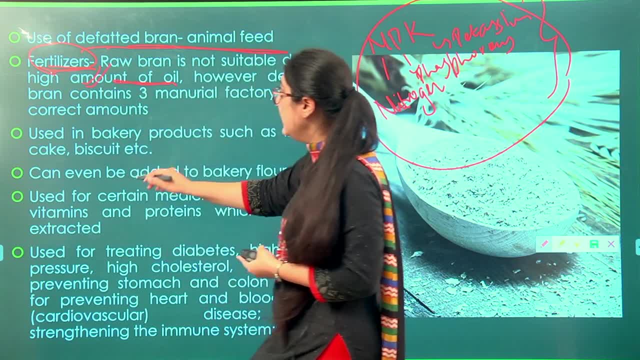 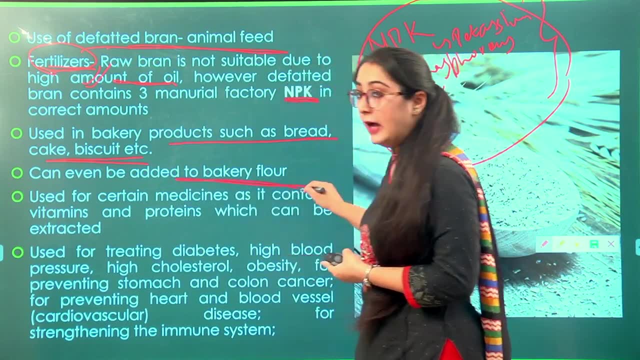 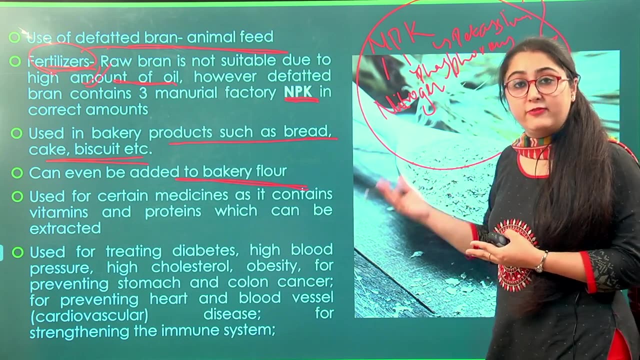 Be Utilized As A Food, As A Meal. It Can Be Added To Quality, Because The Rice Plan Is Very, Very Nutritive, Contains High 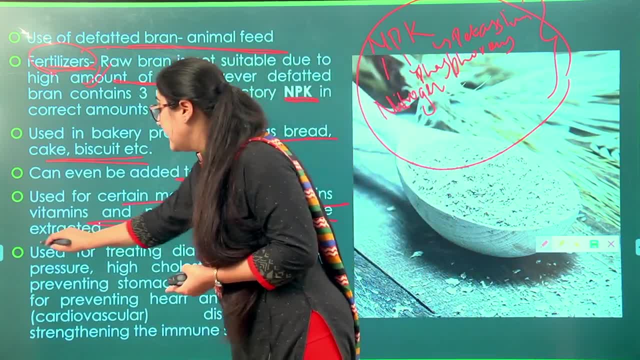 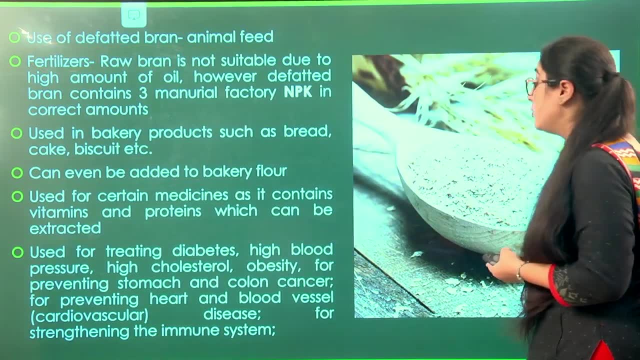 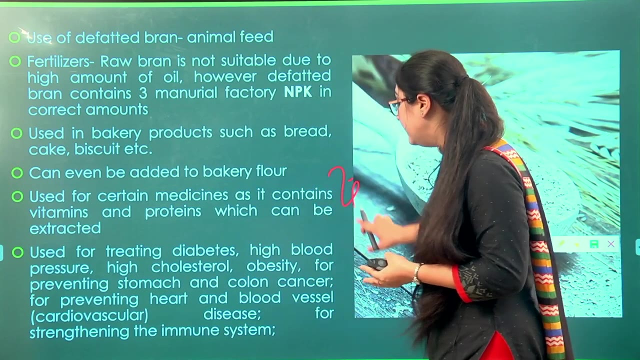 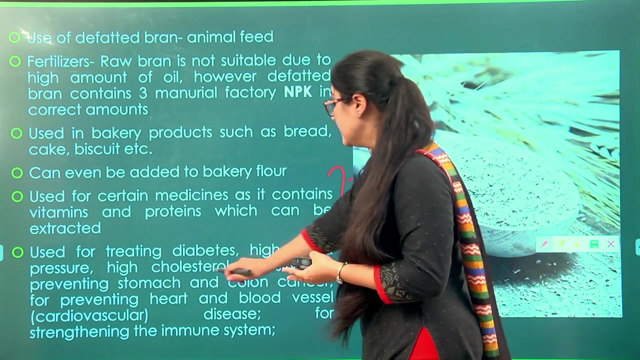 Amount Of Protein, Fat, Horizon, All Vitamin E As Well, And That Also It Has Been Used In The Food. As A Food It Can Be. 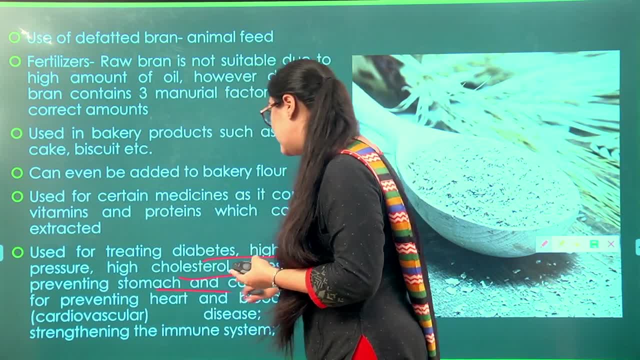 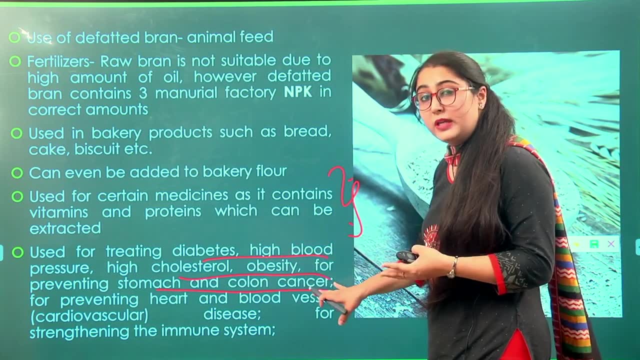 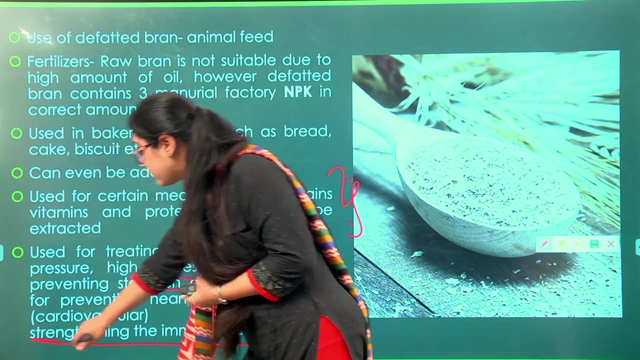 Utilized For The Management Of Number Of Diseases As Well, Such As Diabetes, High Blood Pressure, High Cholesterol, Obesity, Preventing Stomach Lung. For the 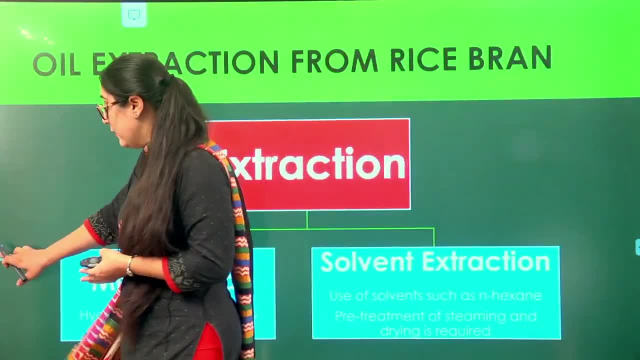 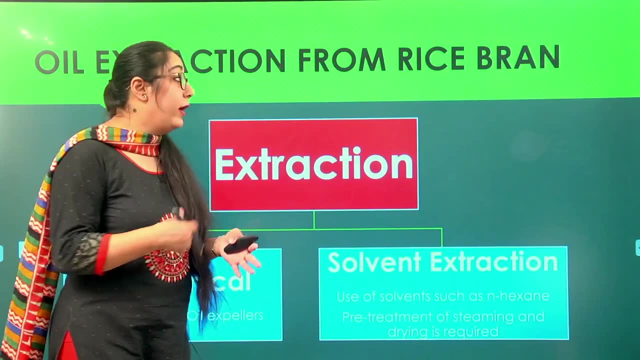 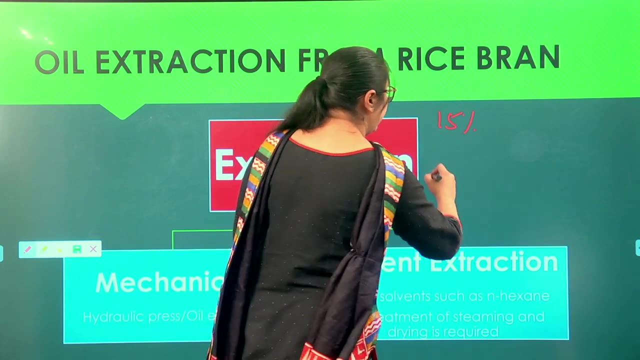 Same. So Now Looking at the oil extraction process from the rice bran. So Oil Extraction Is One Of The Main Users The Rice Bran Is Put Into And Because 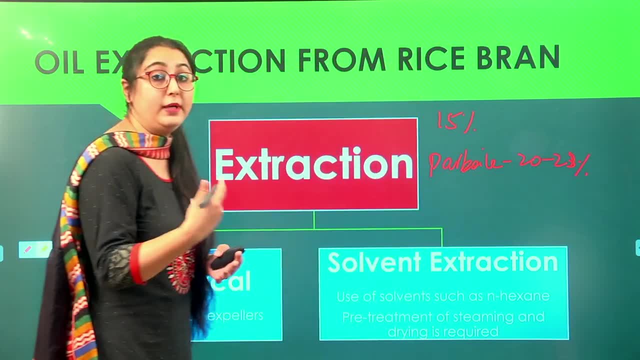 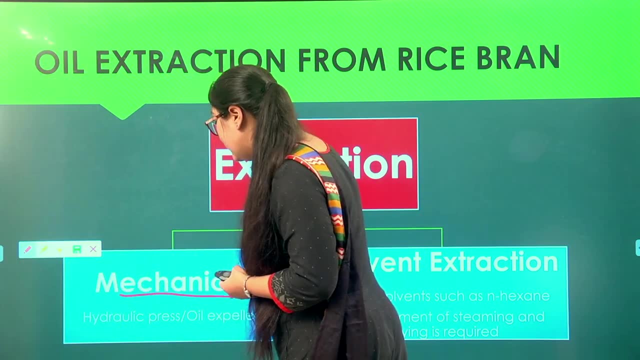 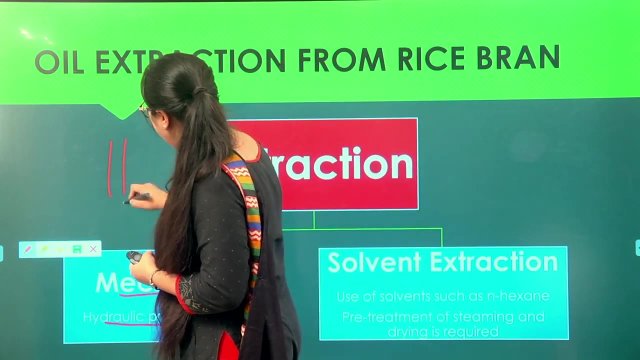 While They Are Extracting Oil From It as well, a good source of vitamin E or Eisenol. so, under the mechanical methods, we have equipment such as a hydraulic press or oil expellers which will extract oil. so, for example, we have vertical plates will be arranged and the 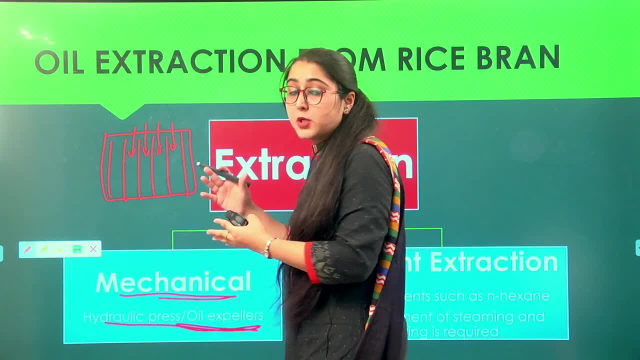 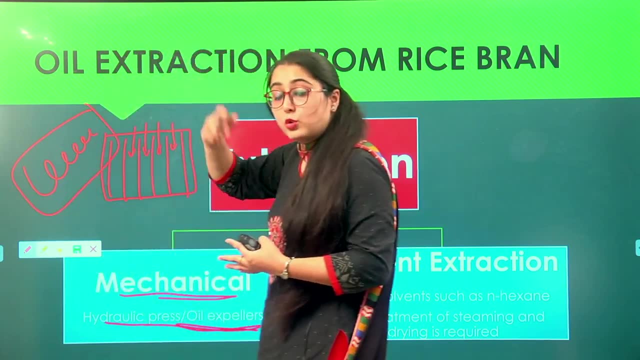 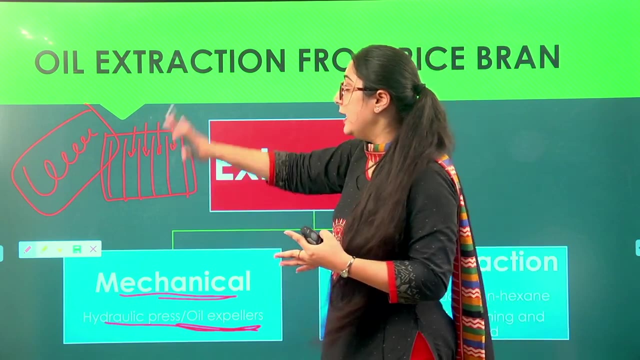 raw material for oil extraction will be kept here and it will be squeezed in order to remove the oil, or utilization of certain equipment, such as a screw press kind of equipment which have screw kind of a shape, and the raw material to extract oil is squeezed and the oil is extracted. so these kind of methods apply. 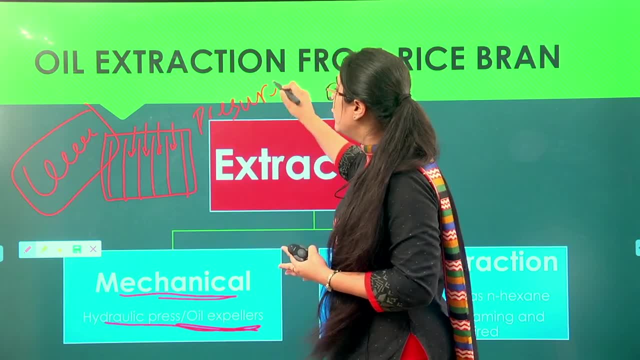 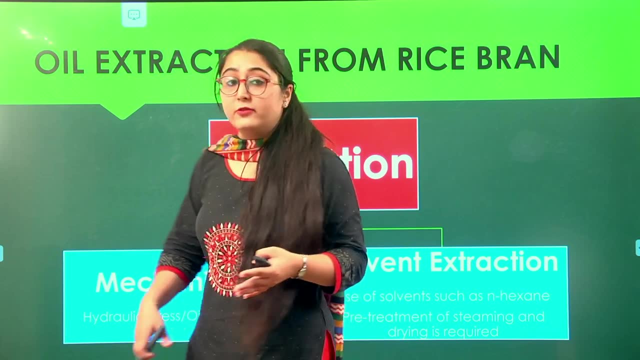 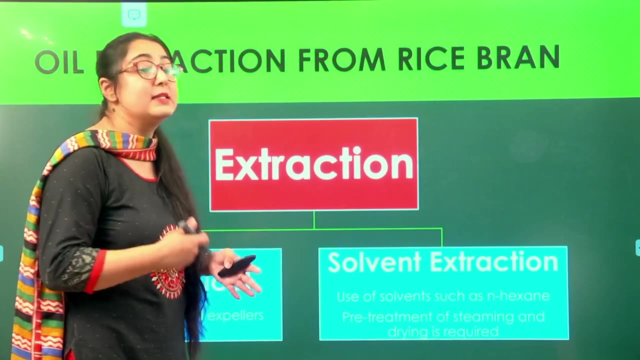 a lot of pressure for the extraction of oil and they are not that good. the amount of oil which is being obtained is not that high as well. so we have, generally, the modern method that we are using is the solvent extraction method and, as the name suggests, we are going to utilize certain solvents for extracting. 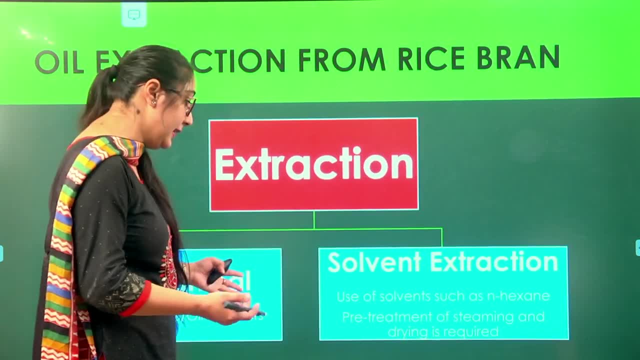 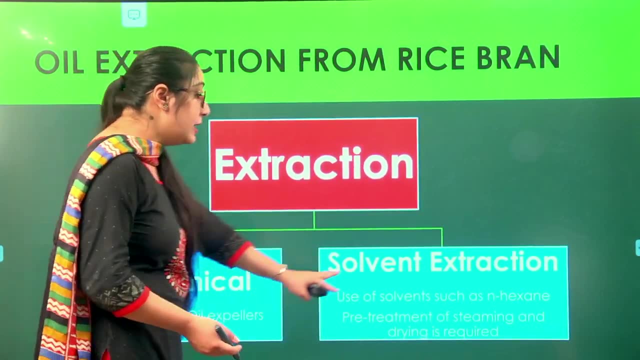 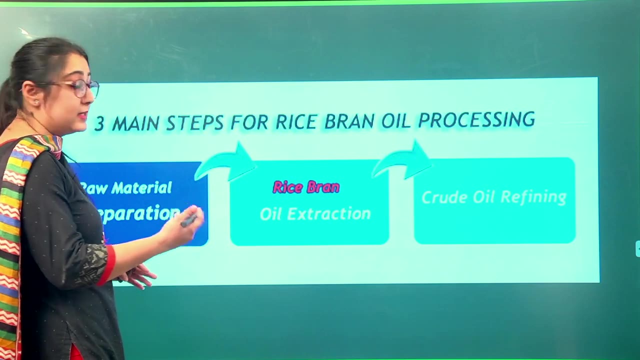 oil out of it. so example of such solvent is n-hexane. and For the production of the rice bran oil, the pre-treatment of the rice bran is very, very important, which consists of steaming and drying the rice bran. So now, looking at the rice extraction oil process, mainly it consists of three steps. 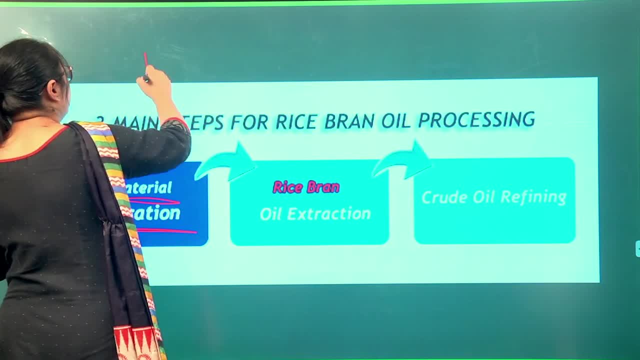 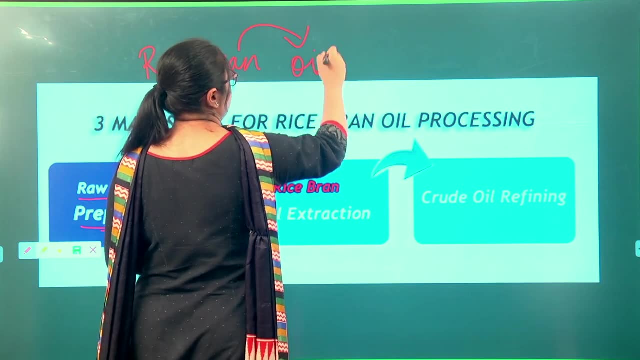 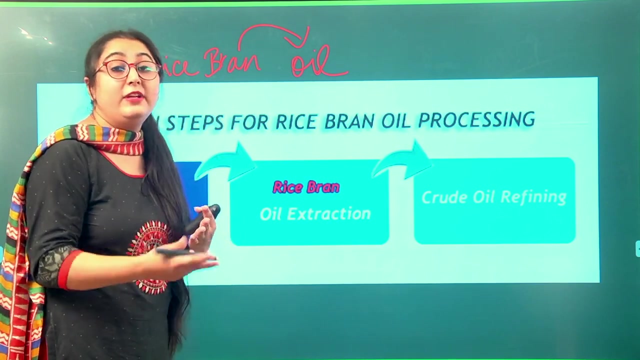 So the raw material is prepared. So we have the rice bran will be taken and then oil will be extracted out of it using solvent extraction method. Once we extract oil out of it- this oil, because it contains a darker color- it will contain certain free fatty acids. 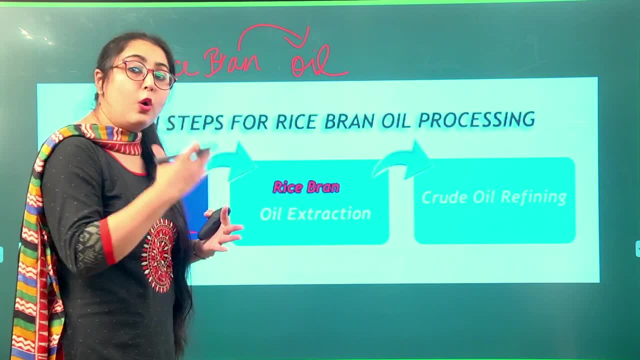 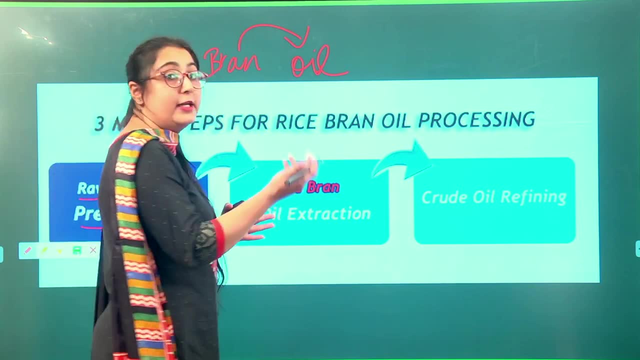 which will impart an undesirable flavor, odor, taste. So all of that have to be removed from the oil before it can be utilized as a oil for cooking or for edible purposes. So the oil in the crude form cannot be utilized and it has to be refined. 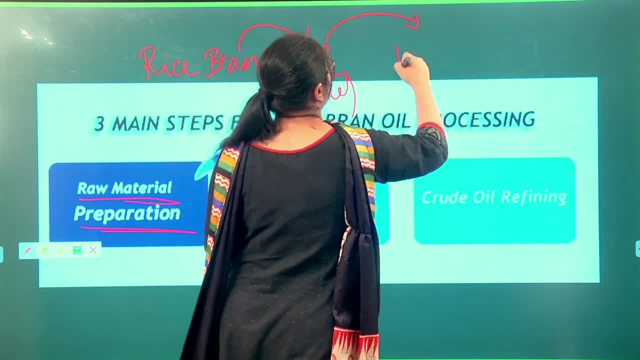 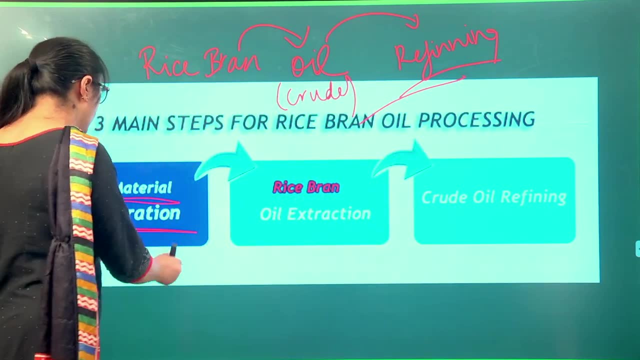 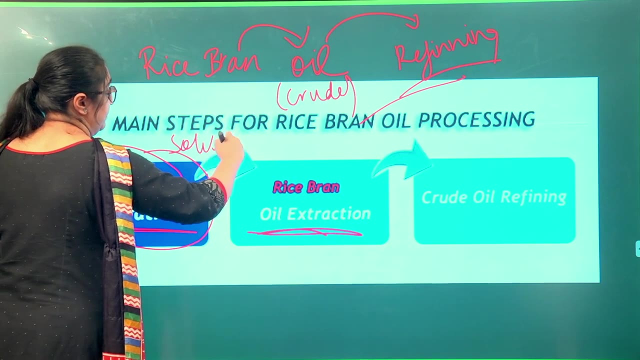 So, after the obtaining of the crude oil, what will happen is refining of oil will be done. So these are the basic three steps. First, we are taking the raw material, that is, the rice bran. We are extracting oil out of it, mainly using the solvent extraction method. 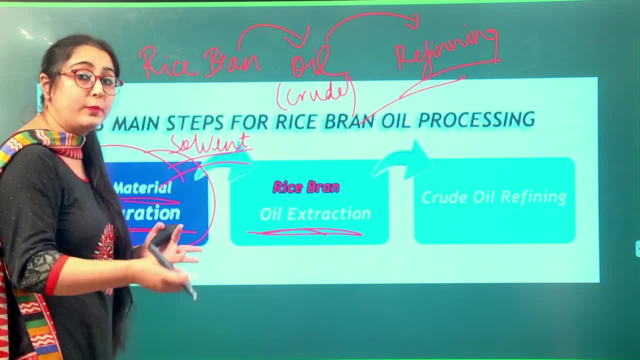 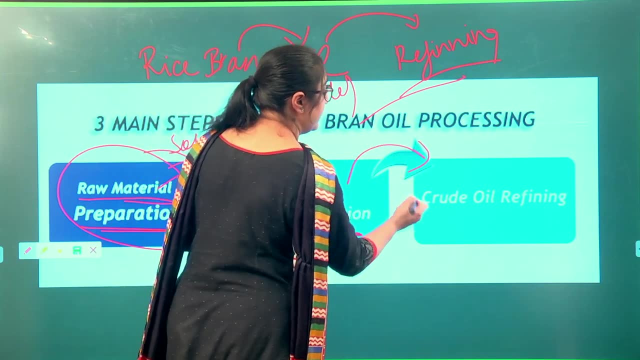 Certain other mechanical methods can also be used, but the oil obtained will be very, very less and not as good as quality as obtained from the solvent extraction method. And then, after extraction, we will go for the refining of the crude oil which is obtained in this step. 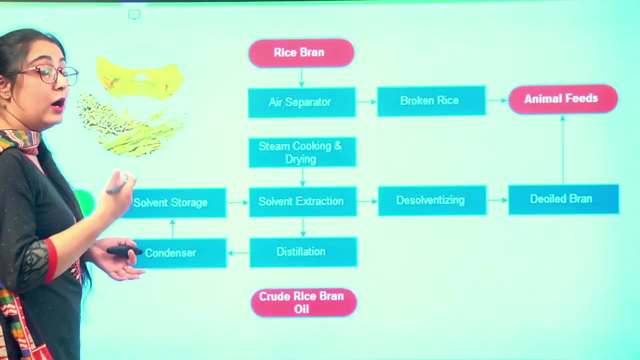 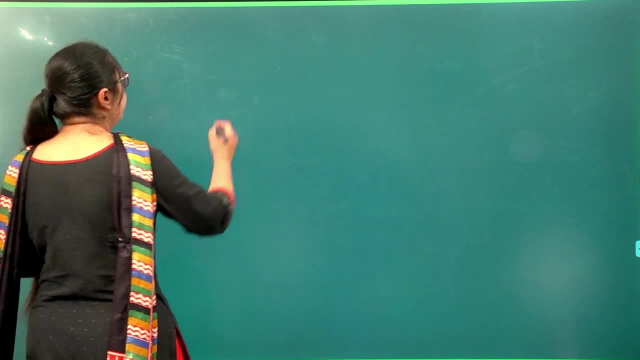 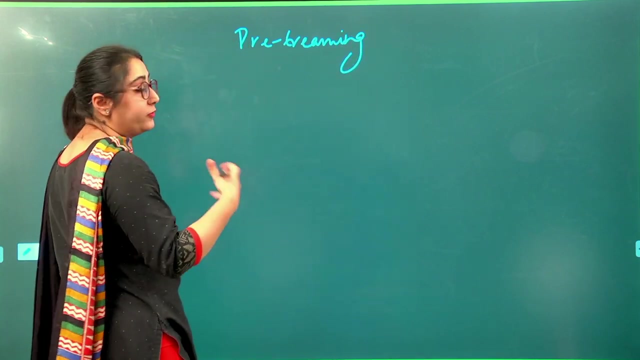 So, first, looking, understanding how this, how this crude oil extraction and refining takes place. So the first step, as we have already discussed, is the pre-treatment which is given to the bran, That is, the steaming and the drying so that oil can be extracted easily out of the bran. 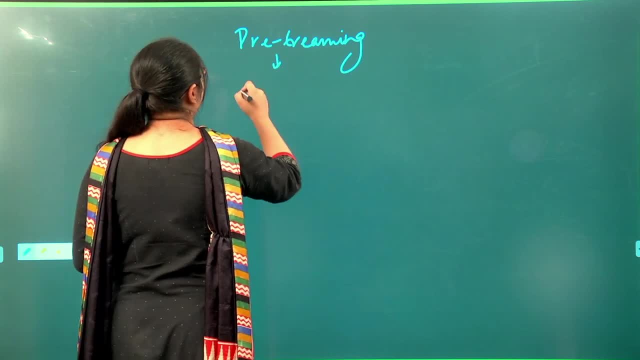 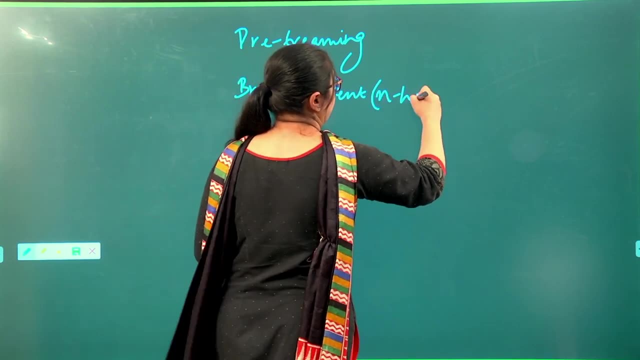 That is why we are giving the pre-treatment And then we are going to mix this bran along with the suitable solvent. So example of the solvent involves a solvent such as N-hexane, So the solvent will have, First of all, the solvent will be able to mix. 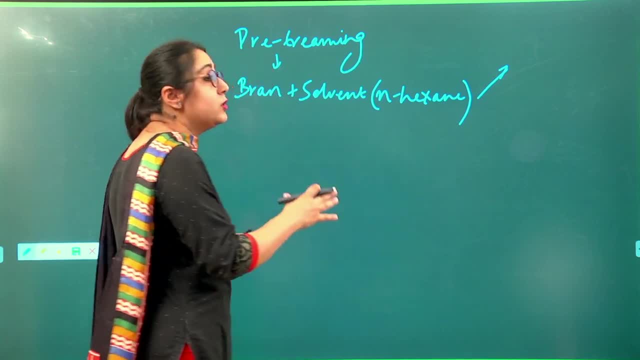 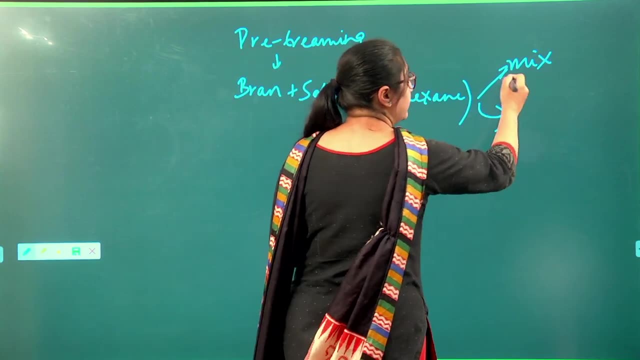 The oil will be able to mix in the solvent. This particular solvent has the property that oil is soluble in it. So it is going to, Oil is going to be soluble in it, It is going to mix in it and, second, it is going to have a low boiling point. 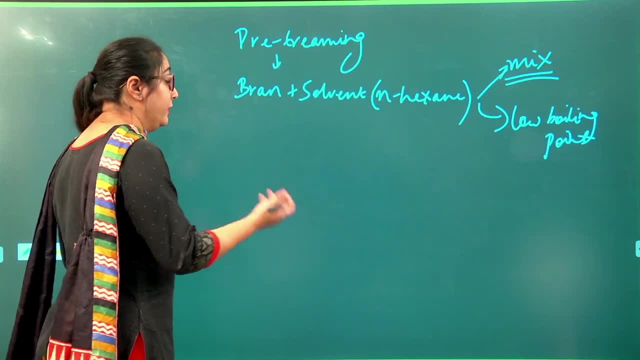 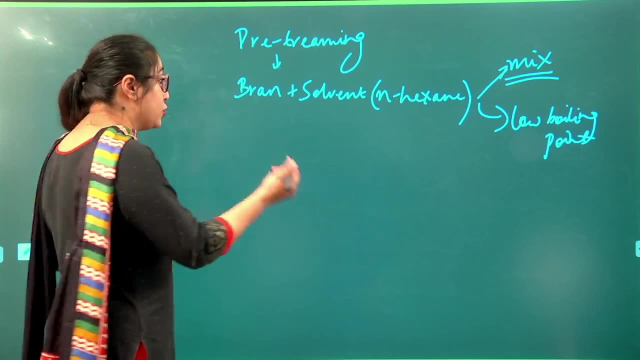 So, because it is going to have a low boiling point, there is going to be an advantage that once we are supplying heat, the solvent can be removed very easily and the oil can be retained. So now what we have over here. it can be divided into two parts after this. 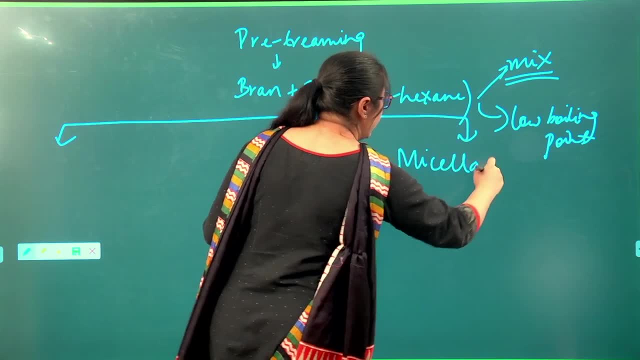 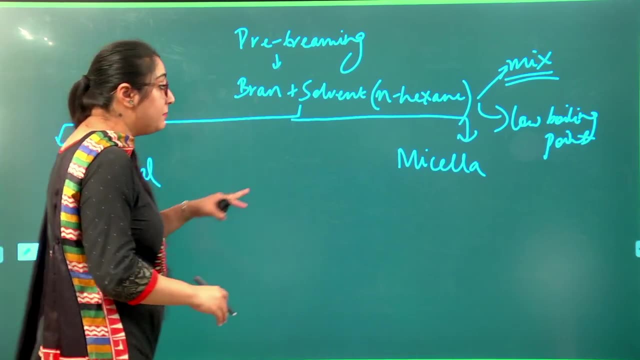 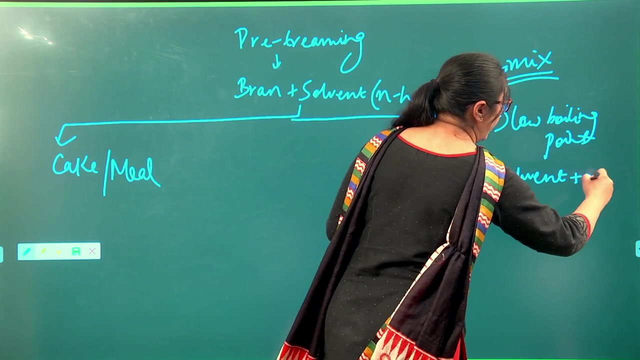 On one side we are taking the miscella and on other side we have the solid cake or the meal. So when we say miscella we actually mean a mixture of solvent. So it is a mixture of the solvent plus oil. So from this miscella, if we are able to remove the solvent, what we will be left with is the oil. 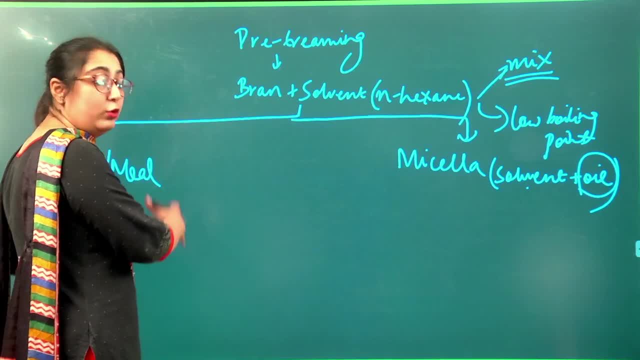 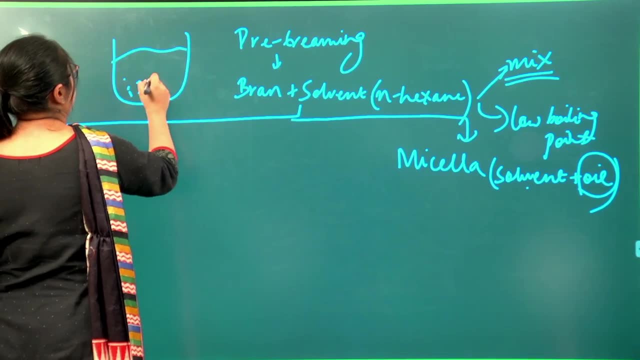 The oil that we want to extract and, on the other side, we have removed all the solid bran which was present. So what we did is we basically we had the bran and we mix the bran with this solvent and now we have extracted all of the solid material at one place. 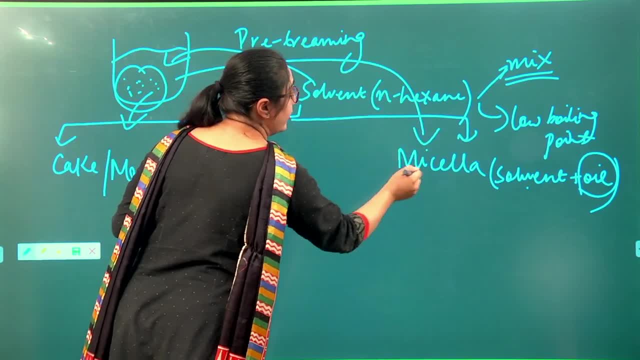 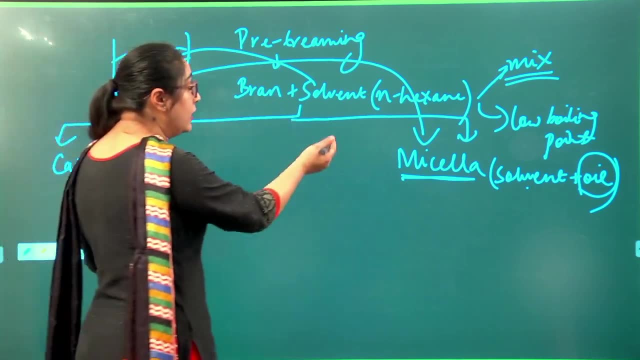 and we have taken all this liquid solvent at the other place in the form of a miscella, because the solvent will solubilize all the oil which is present in the bran inside it, and now the solvent is mixed with the oil. So we have collected the oil and the solvent and we have the solid bran particles. 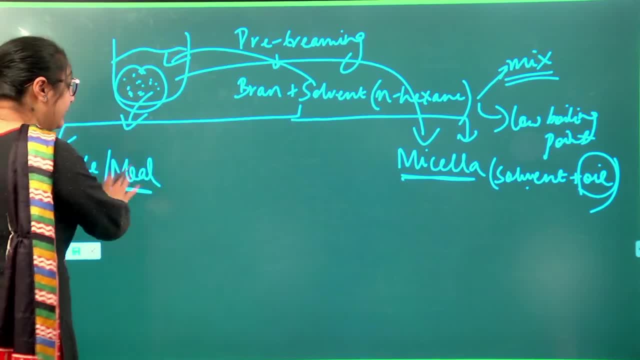 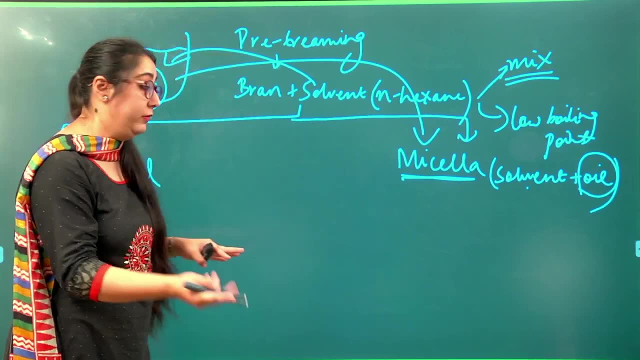 That is the bran from which oil has been removed. The defatted bran particles are in the form of a cake or a meal on the other side. So from this miscella the target is to remove the solvent. So because the solvent has a low boiling point. 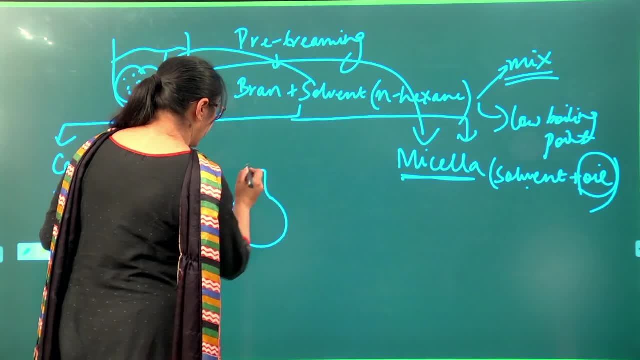 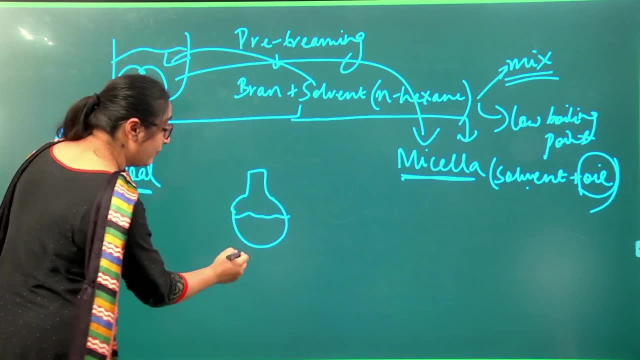 see if we take it in a particular equipment. what can happen is so we have a mixture of solvent and oil over here Now, because the solvent has a low boiling point. if we supply heat to it, what will happen is the solvent will start to evaporate. 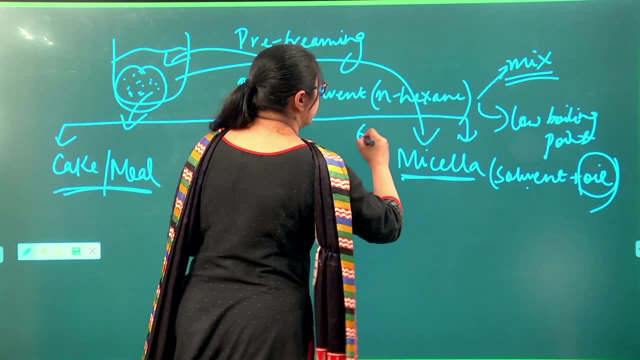 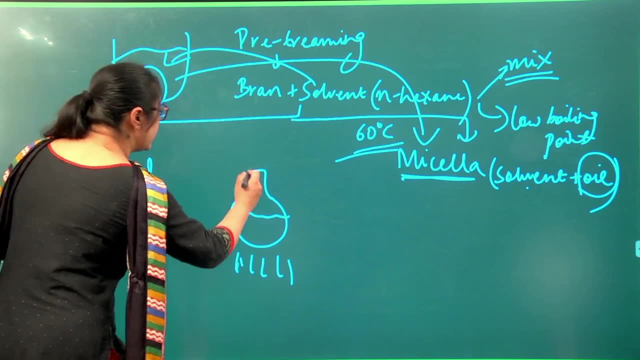 The boiling point of the solvent is very, very low, somewhat around 60 degree Celsius. So if we provide a little heat, what will happen is the solvent will start to evaporate. So the solvent will start to evaporate and the fumes and it will go out. 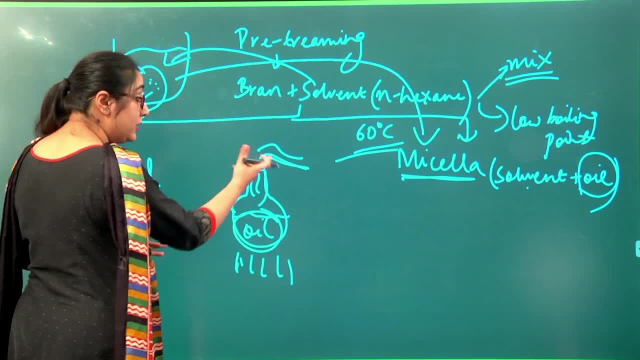 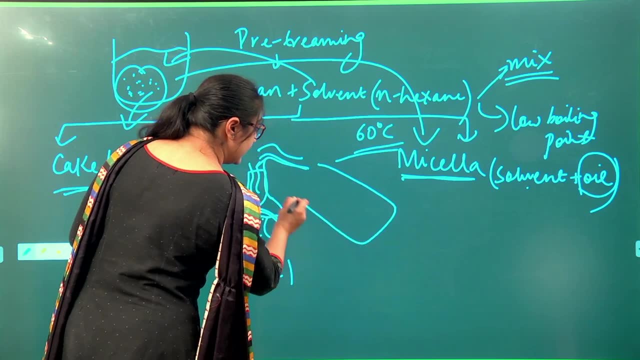 and what will be left over here will be only be the oil. This solvent is again not going to go waste. It can be collected very easily. So what we will do is we will attach one condenser, which will from this condenser. 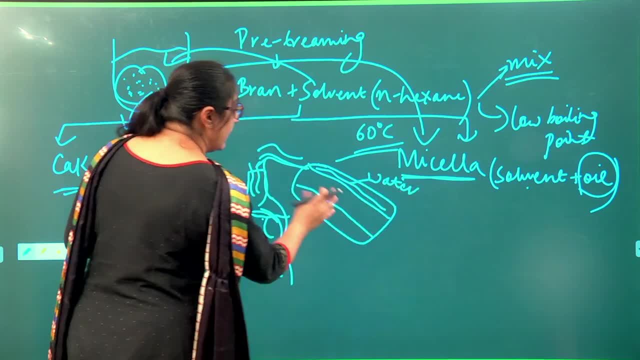 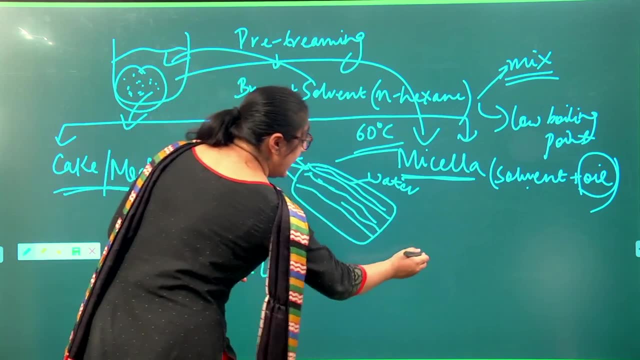 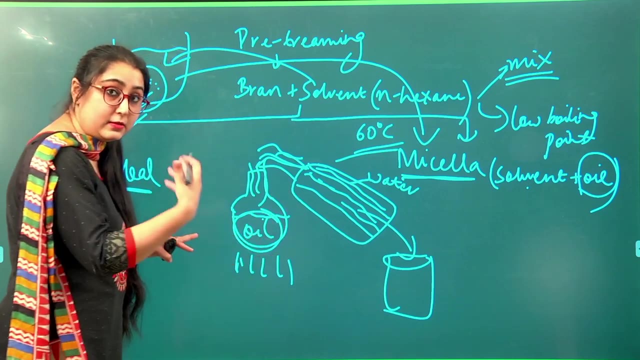 water is passed over here in order to cool it and because it is somewhat cooler, these vapors will condense over here and again convert back into liquid form and in a separate beaker they can be collected. So the solvent is also collected back through a condensate, through a condensing system. 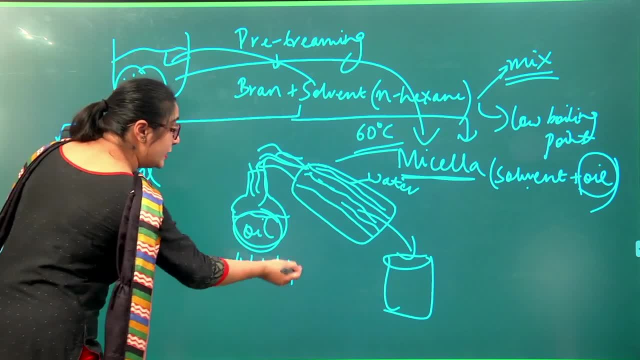 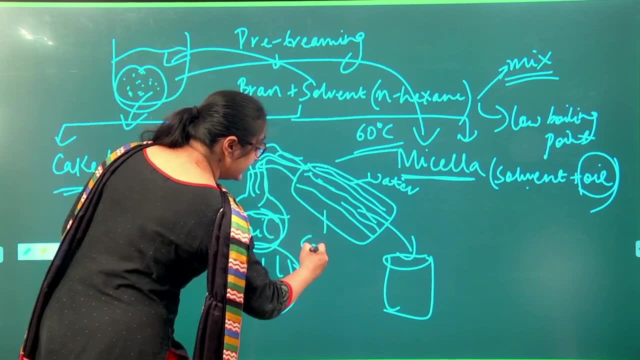 So what we are doing is we have oil mixed to the solvent Once we supplied heat. what will happen is the solvent will evaporate because of having a low boiling point, and then we attach the condenser which is going to condense it back into liquid form. 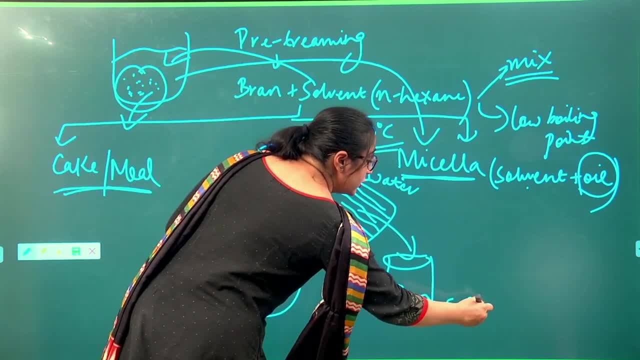 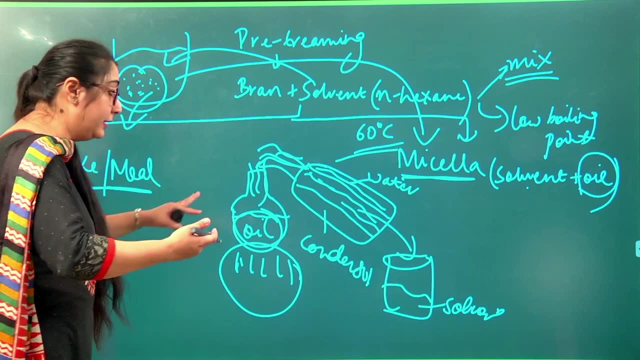 and we are going to collect the solvent back separately, So the solvent can be utilized again and again, and again for the extraction of oil, because it is not going to be contaminated. The oil has been removed out of it and the solvent is again back into its pure form. 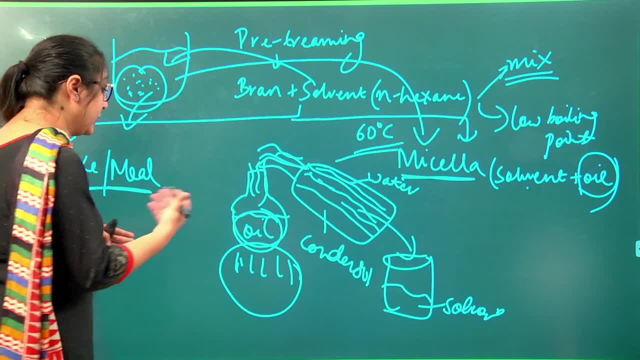 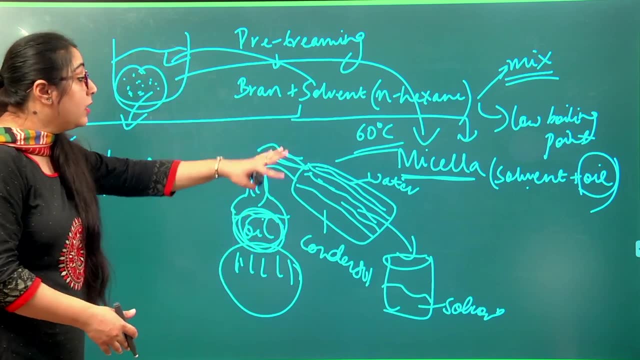 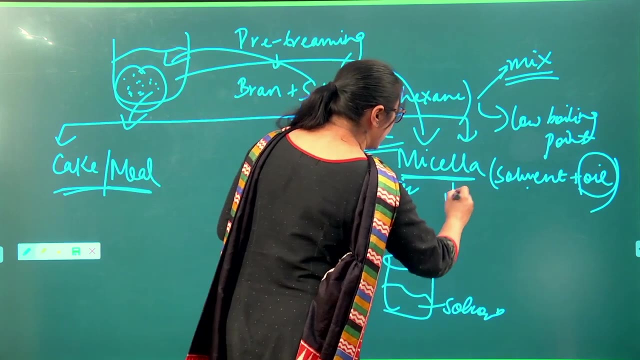 and again. it can be utilized for the extraction of oil, So it can be brought to use repeatedly And what will be left over here is the pure oil. In this way, the miscella can be separated into the oil and solvent. So what will happen is this miscella will undergo 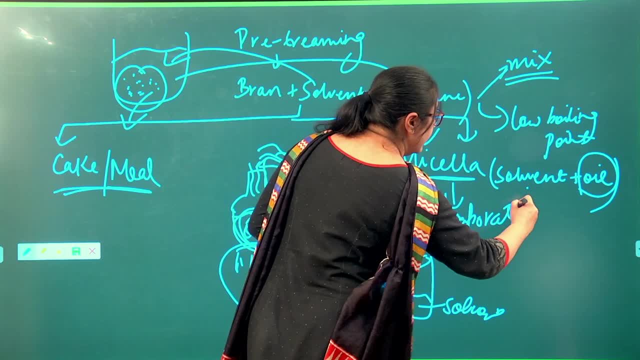 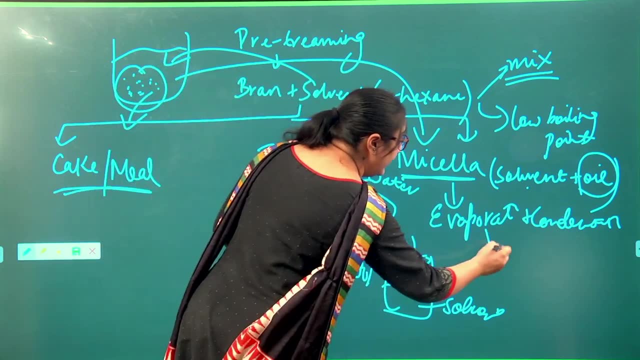 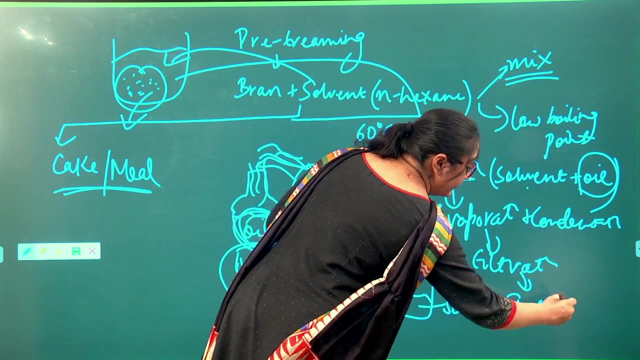 we will subject it to evaporation, followed by condensation, so that the solvent can be removed, and then, whatever oil we have left, we can simply go for filtration of the oil to ensure that it is clean, and what we collect is the crude oil. On the other hand, after evaporation and condensation, 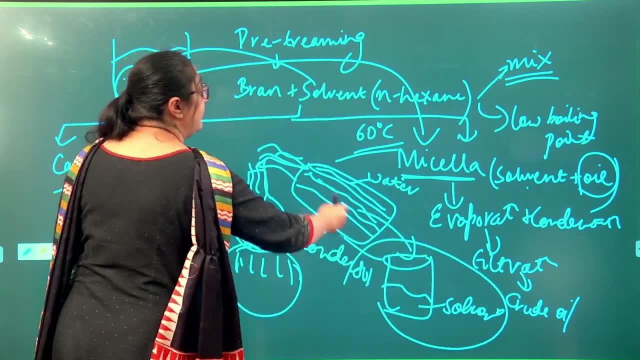 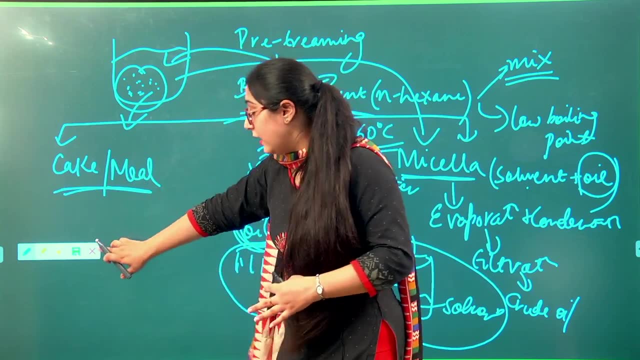 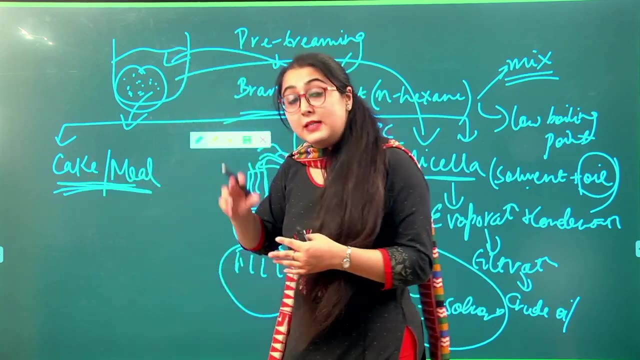 the solvent which is being recovered can be sent back again and utilized over here in this step again, in the bran and the solvent, On the other side we have the cake and the meal and this cake or the meal again we had discussed when we were discussing the uses of bran. 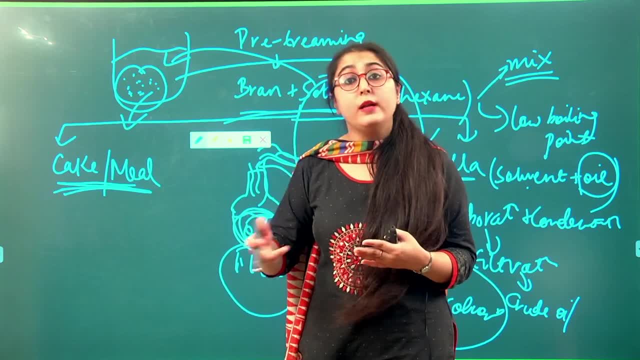 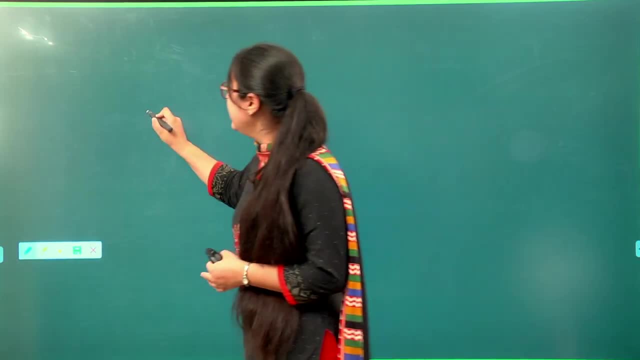 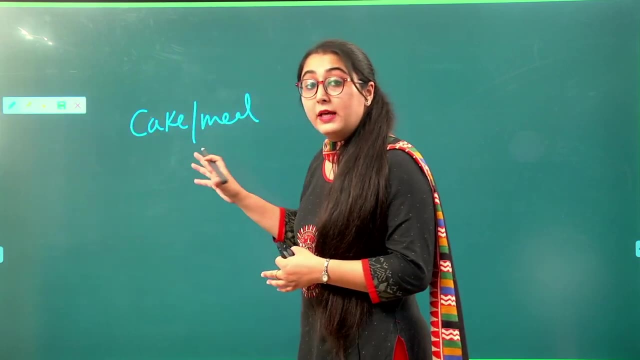 that even defatted bran has a use as a fertilizer or animal feed. So again, this bran cannot be left waste. It has a number of uses. So from the cake or the meal which we have obtained, again we want to remove the bran and we want to utilize the defatted bran. 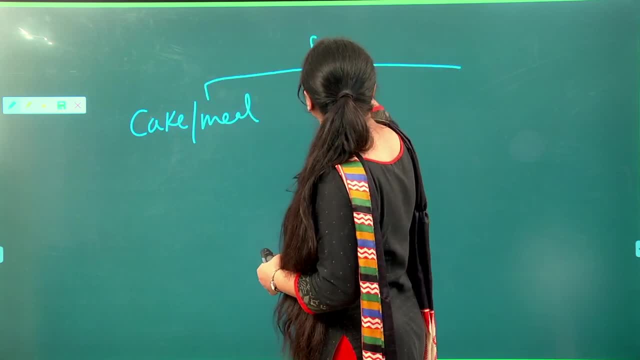 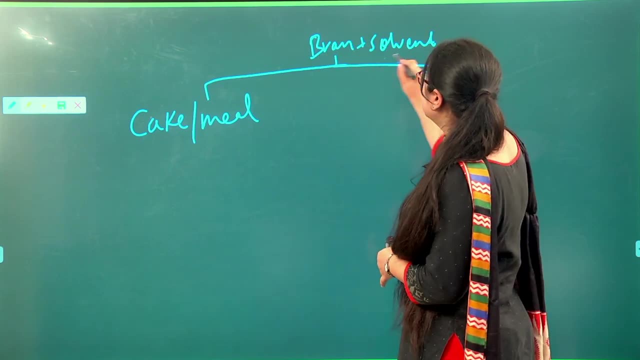 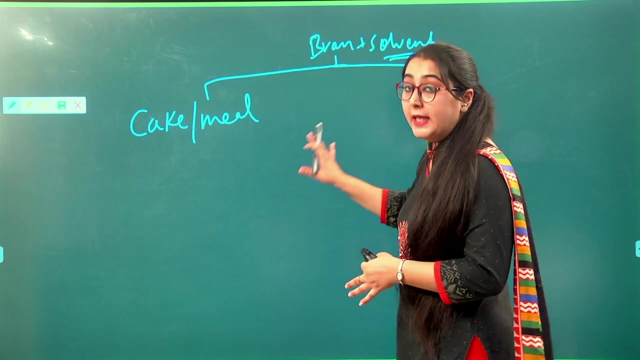 So this cake or the meal. so because we had added a solvent to it, this cake or the meal will also be contaminated with some amount of that solvent, So that solvent has to be removed from the cake or the meal as well. So what we will do is we will subject this cake or meal to steam. 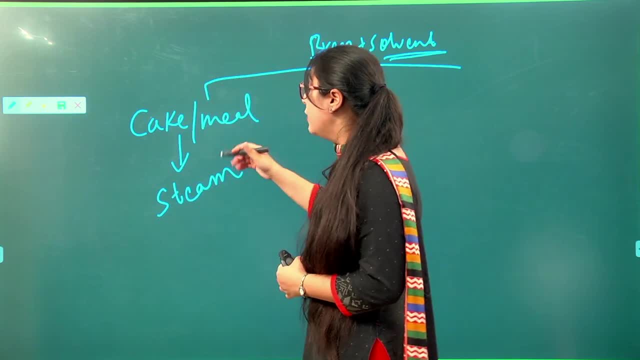 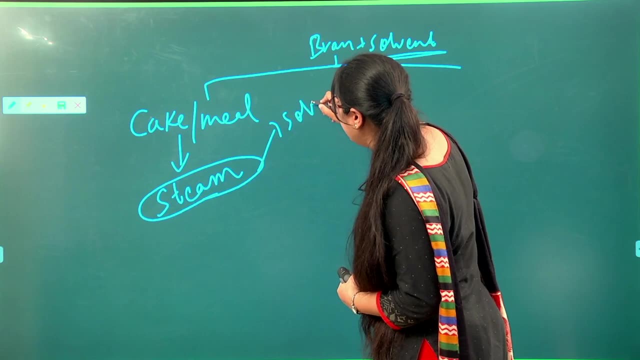 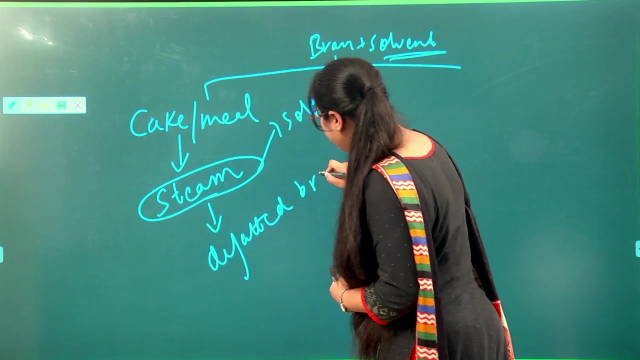 So once we are subjecting it to high steam, what will happen is, because of the high temperature, again the solvent will be evaporated. So the solvent will be removed and what we will be left with is the complete, pure defatted bran, which can be used in a number of uses, such as: 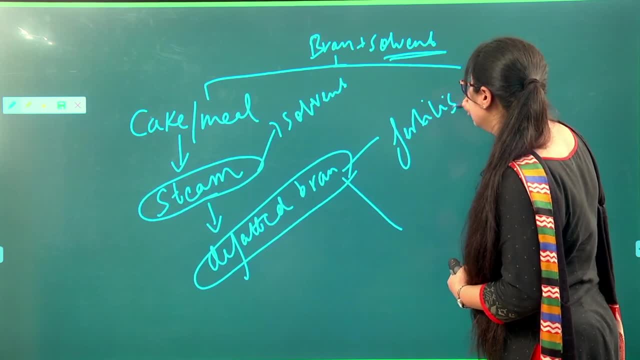 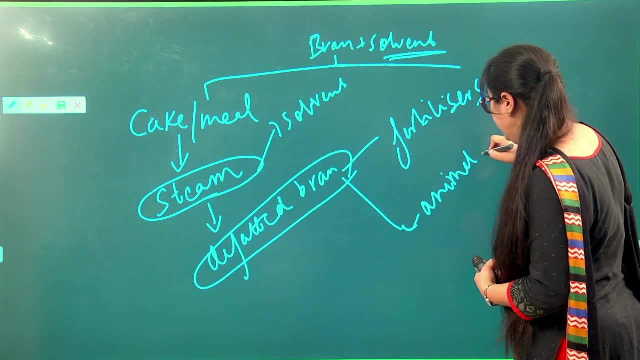 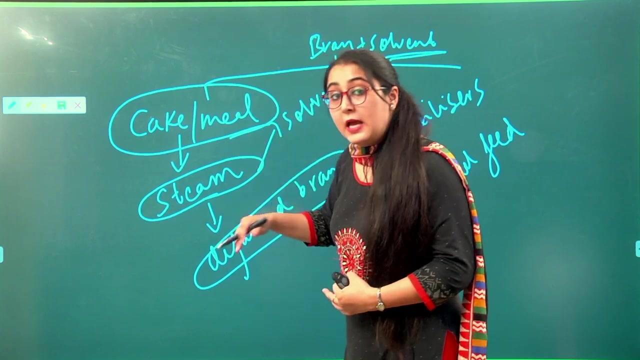 we can utilize it as fertilizers, or we can utilize it for producing as an animal feed because of high fiber content. So in this way, even the cake or the meal finds uses, because the defatted bran will be obtained for it. And for that purpose we have to remove any places of solvent which are 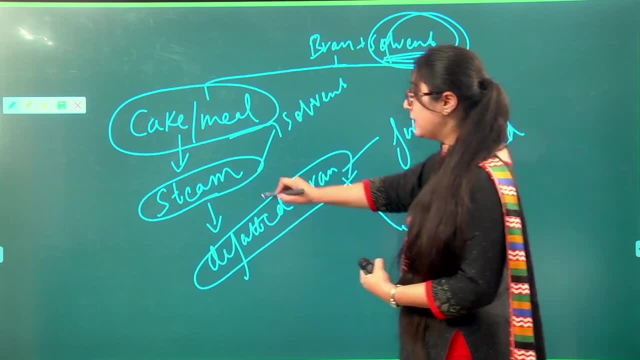 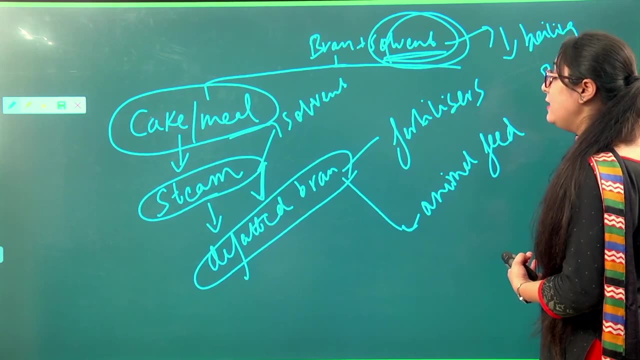 which might be present in it. To do that, we will subject it to steam And again, since the solvent contains a very low boiling point, what will happen is it will evaporate And what will be left is the solvent will be removed. 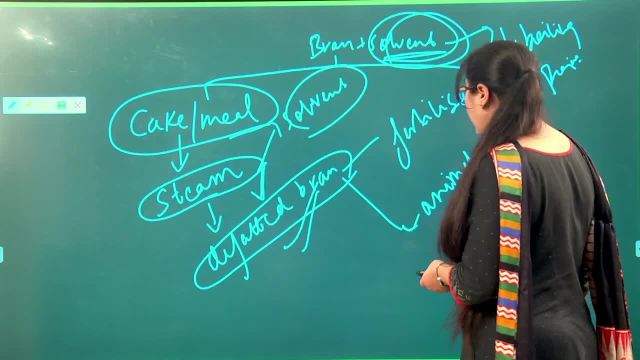 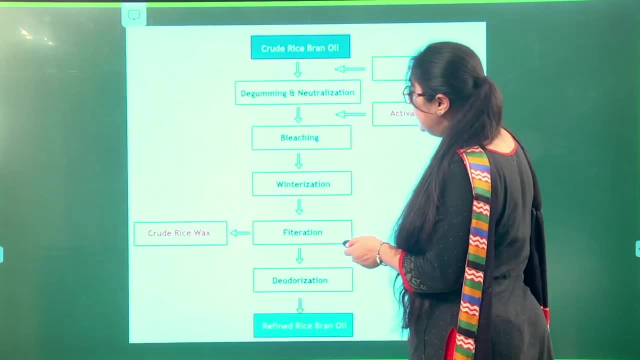 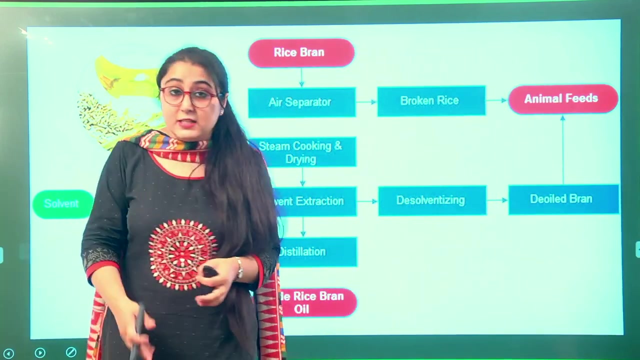 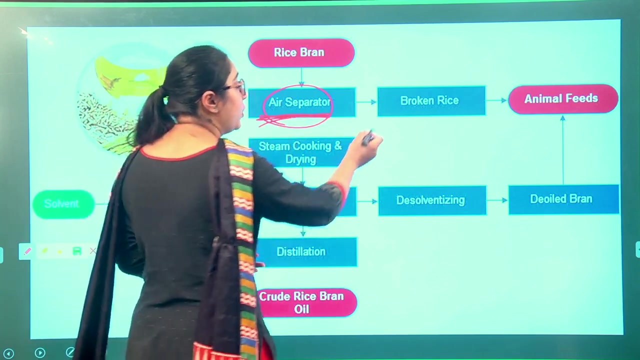 and what will be left is the purified, defatted or the de-oiled bran. So now, if we look at basically the crude oil extraction process, the rice bran is being present and first we are utilizing the air separator. So the use of air separator is simply to separate any broken rice bran. 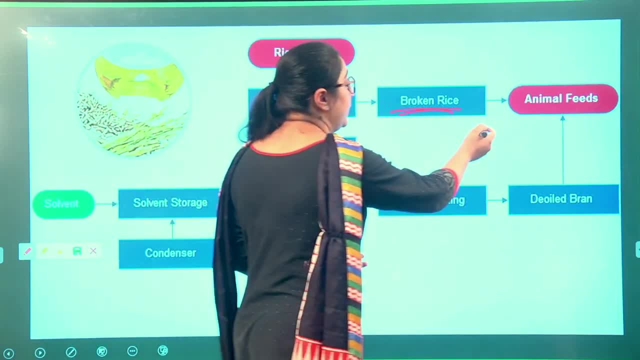 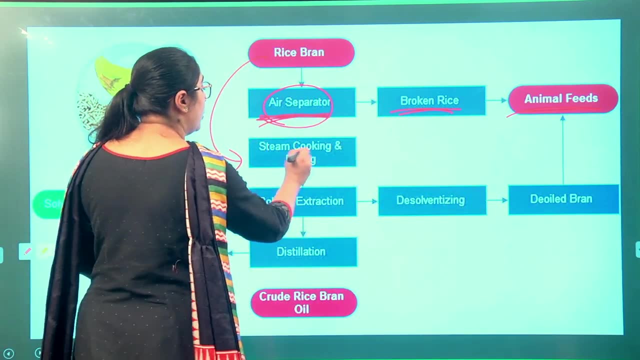 which might be mixed with the bran. So these broken rice will be utilized separately as an animal feed and what we have is the pure bran over here. So first step is the cooking and the drying: steaming and the drying. That is the pre-treatment which we have discussed. that pre-treatment has to be given. 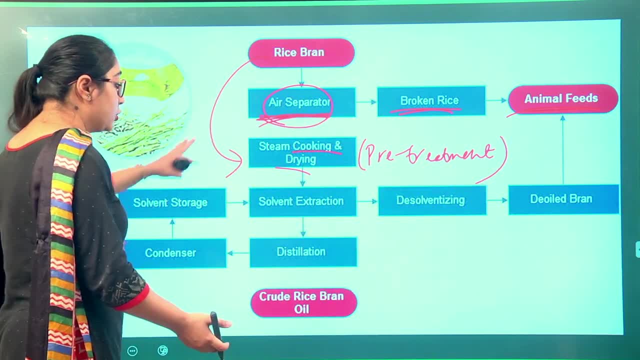 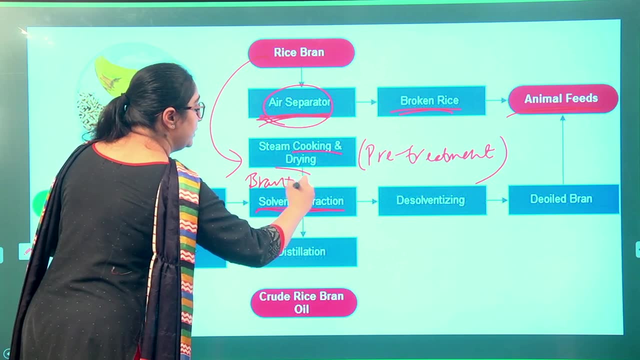 so that oil can be extracted efficiently out of it. So after the pre-treatment, we are subjecting it to solvent extraction, meaning we are mixing the bran along with the solvent in this step. So what will happen is distillation, condensation. all of this is performed. 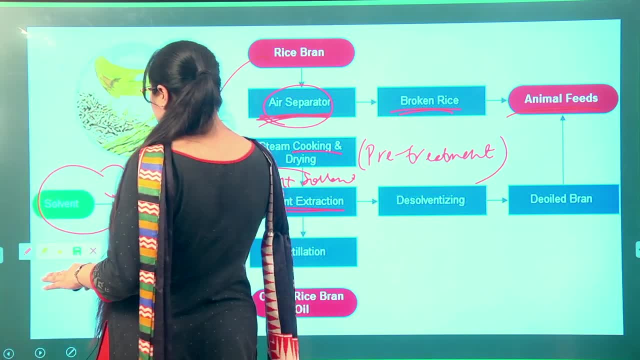 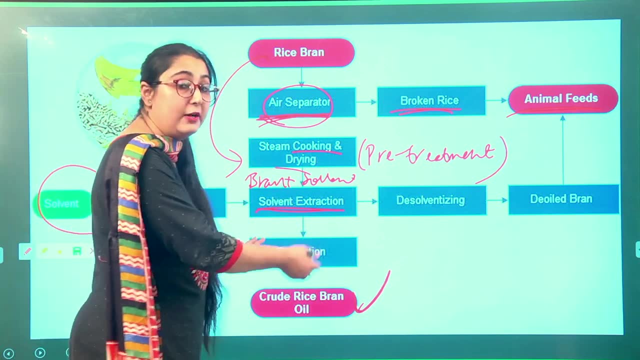 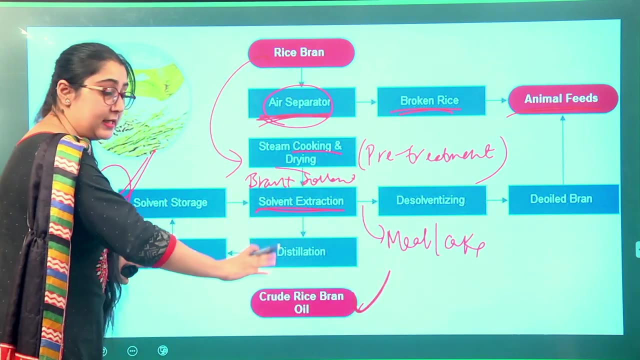 and, as a result, on the one side we can collect the solvent, on the other side we can collect the crude rice bran oil and whatever is left, the meal or the cake. here we are dealing with the meal or the cake and here, basically, we are dealing with the miscella. 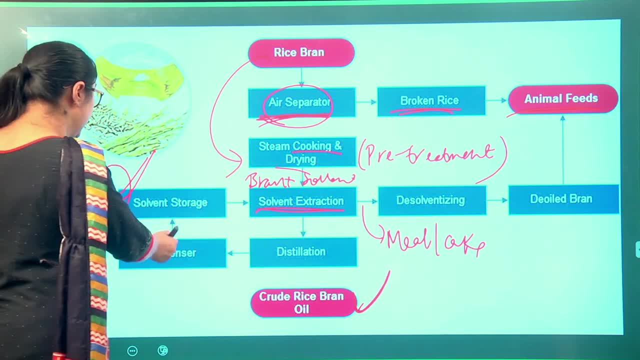 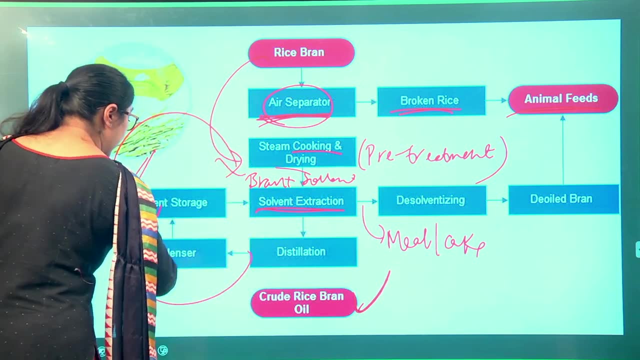 that we are subjecting it to evaporation, condensation, distillation, all of this and then obtaining the pure solvent, So that the solvent can be utilized again and again and again for this process, because the same solvent can be utilized n number of times. 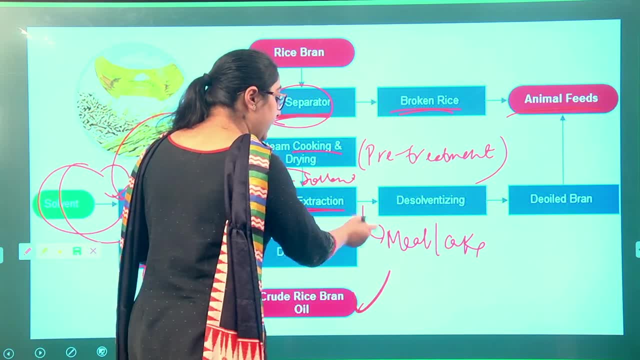 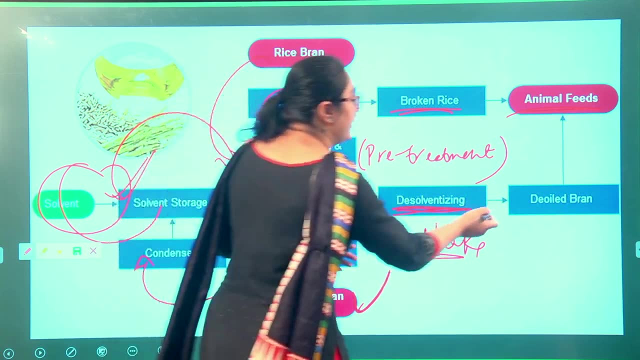 since no contamination is being occurring, and this particular meal or cake, again on the second side, that we have the solid portion. after desolventizing it, removing solvent from it, removing oil from it, it can again be used as an animal feed, along with the broken rice. 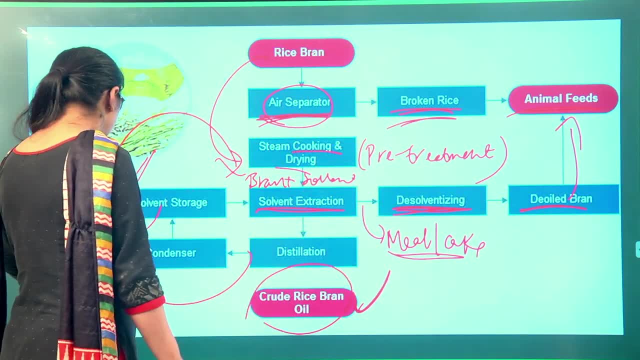 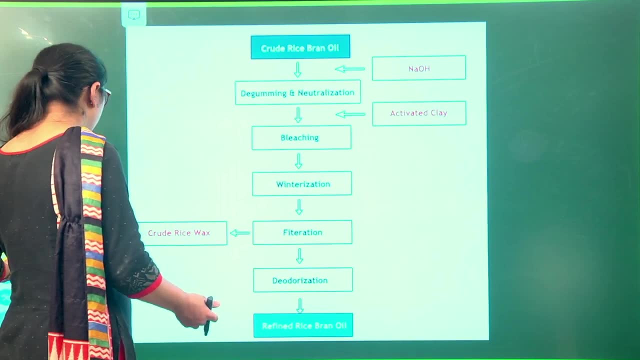 and we are obtaining the crude rice bran oil. So now, after obtaining the crude rice bran oil also, that crude rice bran oil cannot be put to use because it will have a lot of off flavor, off odor. so all of that has to be removed. 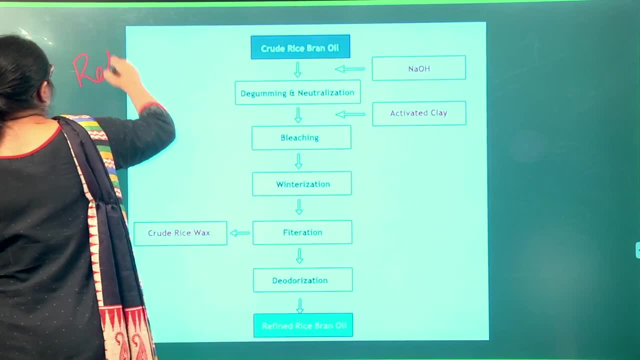 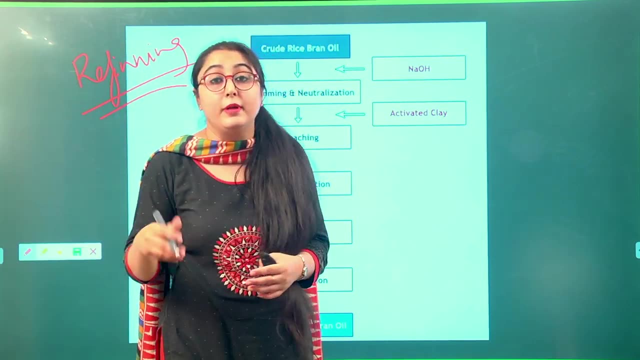 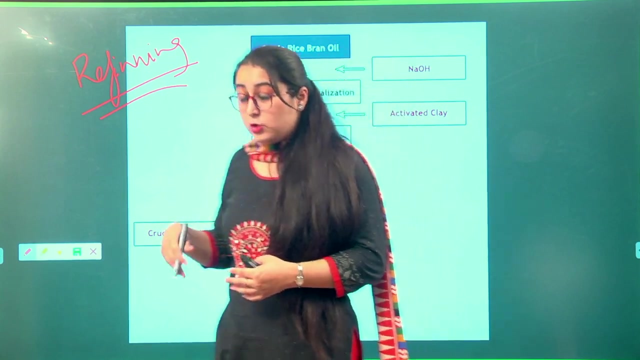 For that process, refining of the oil is done. So one disadvantage that we studied, or one problem that we studied associated with bran, was that refining in case of the rice bran oil is much more difficult as compared to other vegetable oils. So how this refining is basically done, 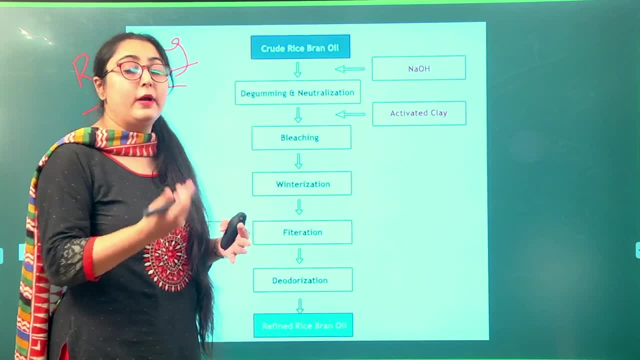 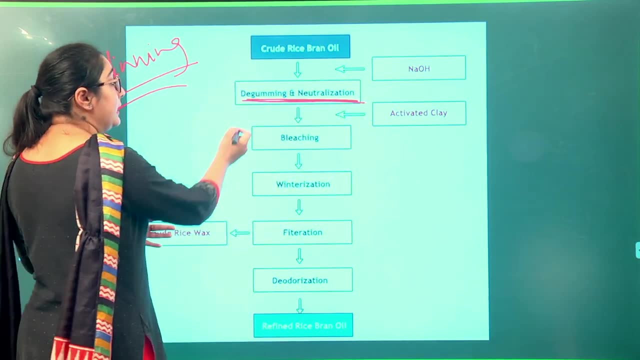 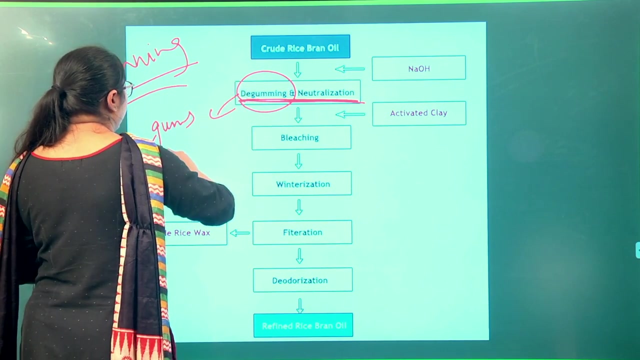 In the refining process we have to remove all of those which were providing an undesirable taste or odor. So first step we have is the degumming and the neutralization. So, as the name suggests, degumming meaning removal of the gums. So in this step, basically we are going to remove any gums or any mucilages kind of a material. 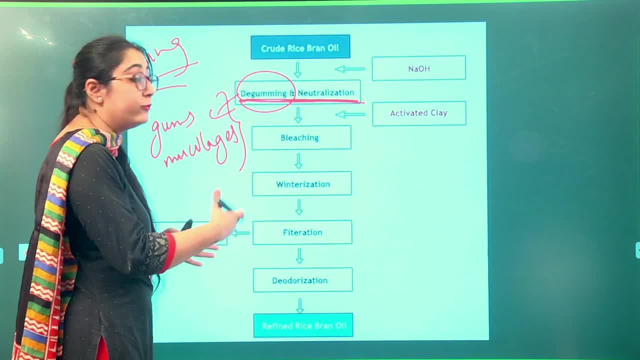 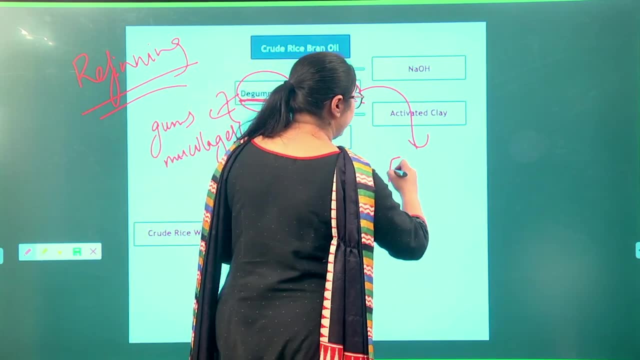 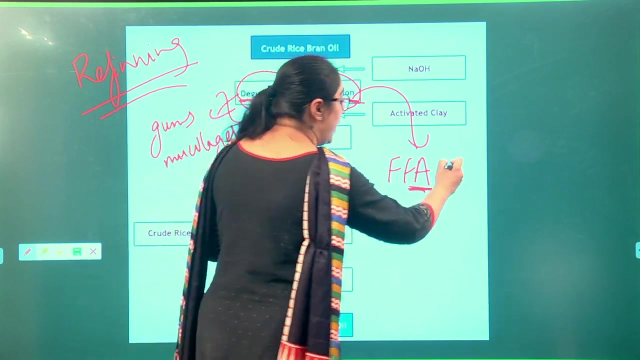 which might be present in the fats and the oil. They have to be removed. and in the neutralization process, again, as the name is telling, we have to neutralize. So we have to neutralize the free fatty acids which are present. So for utilizing the free fatty acids, since they are a type of acid, a base can be added to neutralize it. 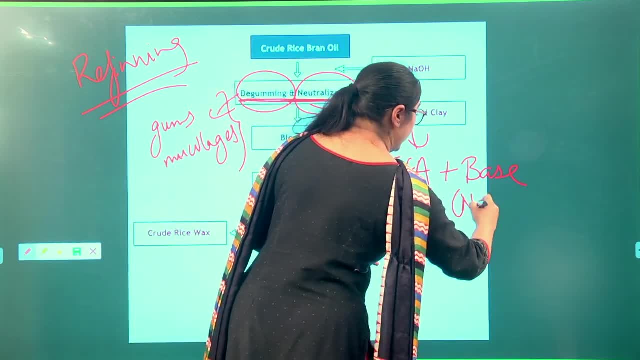 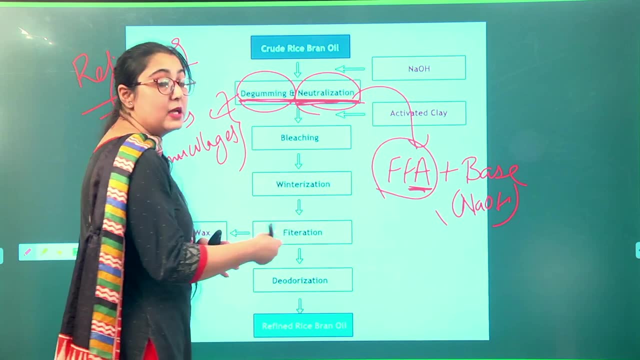 and the base that we are adding is NaOH. So for that reason, NaOH is being added in that step to neutralize the free fatty acids, because the oil, which is high in free fatty acids, cannot be utilized efficiently for the cooking or edible purposes. 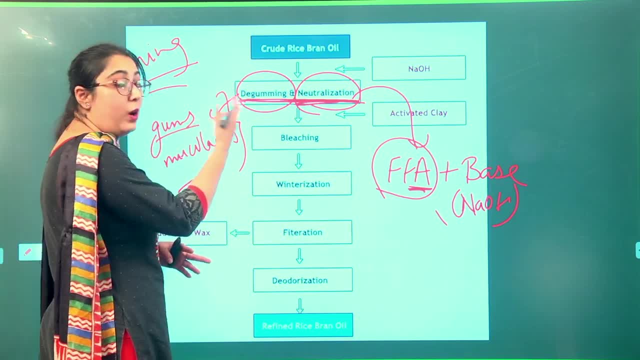 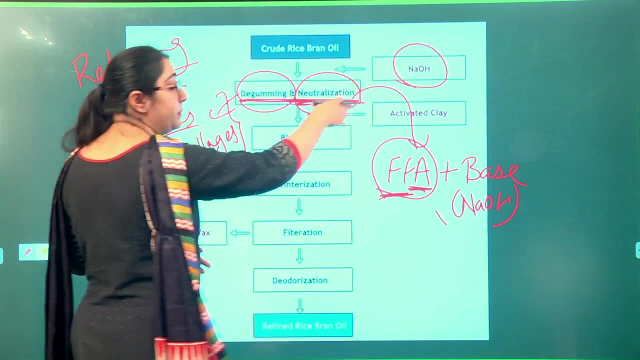 So, in the first step, we are removing the gums. So we are removing the gums or the mucilages, or, and we are doing the neutralization, that is, removing the free fatty acids, neutralizing the free fatty acids with the base, which is NaOH. 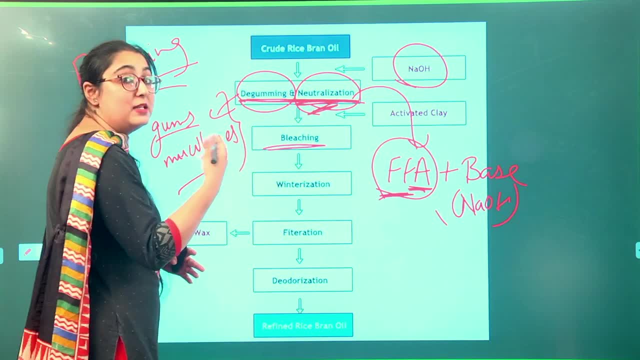 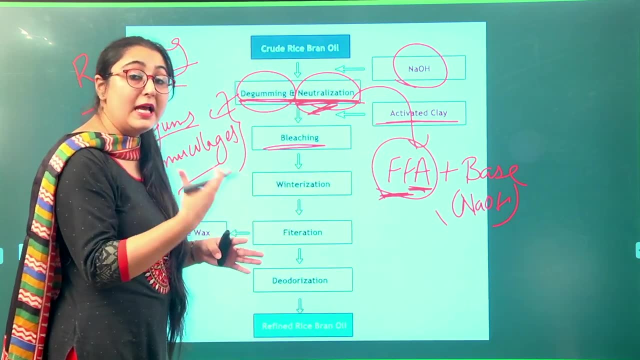 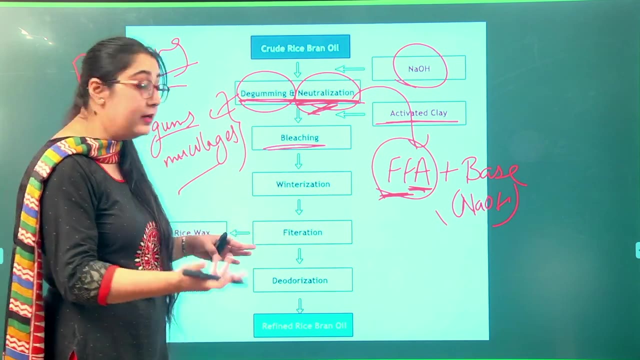 And after this we will perform bleaching, So, as the name suggests, trying to improve the color. So what we will do is we will add activated clay over here. As we know, clay has a very good absorbing properties. So all of those coloring pigments which are present in the oil which is giving the undesirable color, 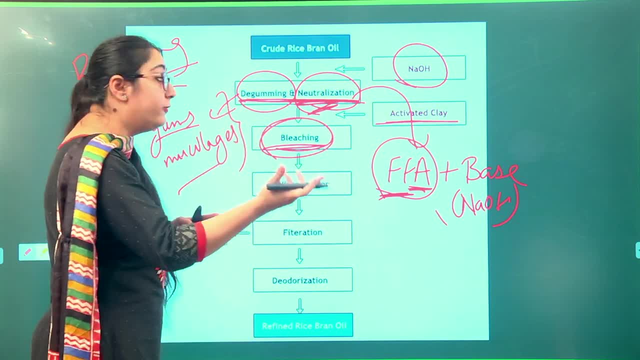 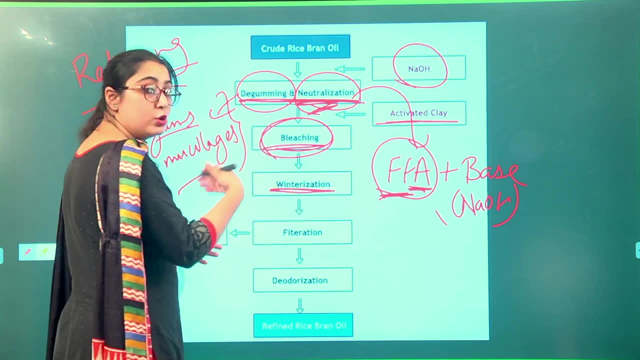 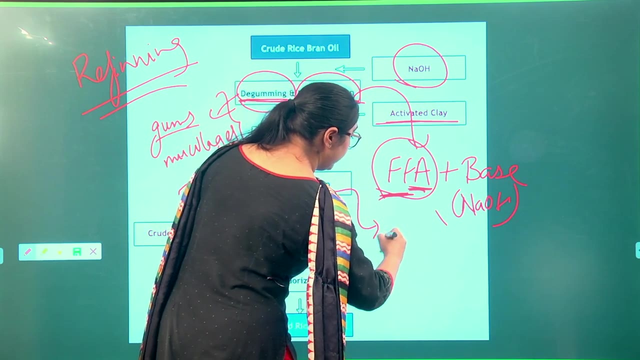 can be removed in this step. So adding of clay will remove all the coloring pigments and make the oil lighter in color. And then next step is the winterization. So, as the name suggests, winterization, utilization of cold temperatures. So what we will do is we will subject our rice to cold temperatures around freezing, around 0 degree Celsius. 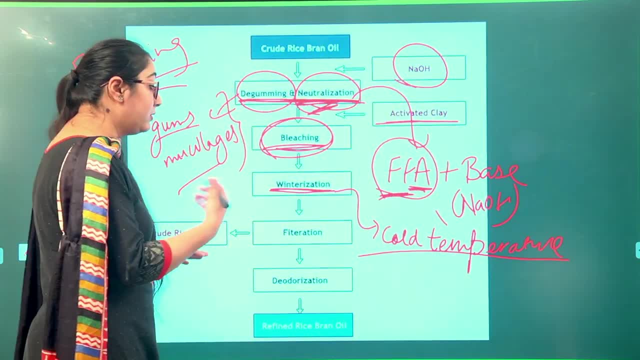 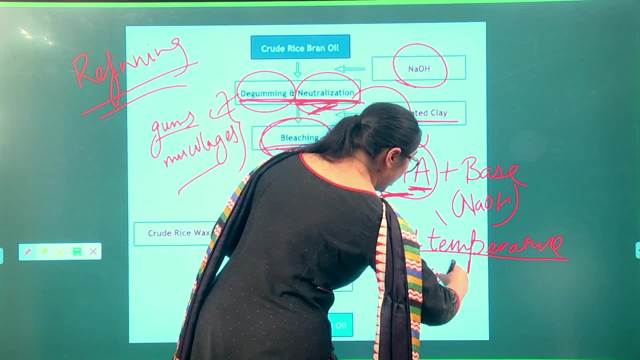 And what will happen at this cold temperature is all the triglycerides will be solidified. So this step is basically done To remove the triglycerides, or we can call them as triacylglycerols as well. So triglycerides are being removed. 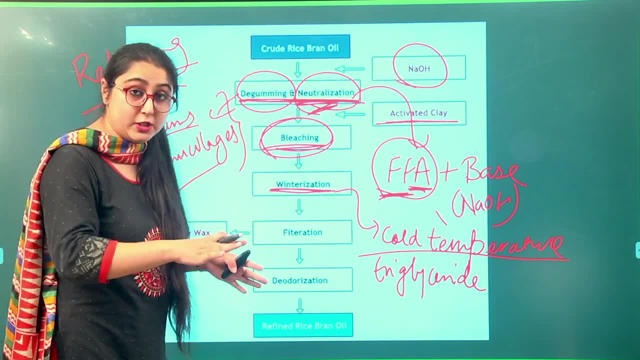 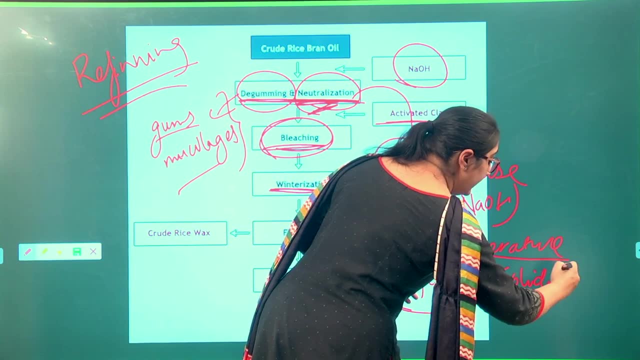 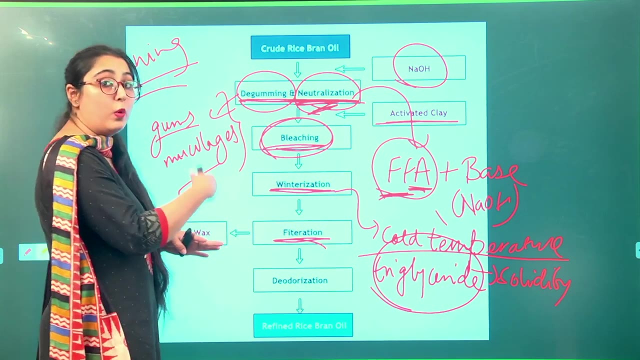 How they will be removed is it is being subjected to cold temperature. Once it is subjected to cold temperature, these triglycerides will solidify, And when they are solidified they can be easily removed from the oil by filtration. So winterization is followed by filtration, so that whatever triglycerides were solidified here can be removed. 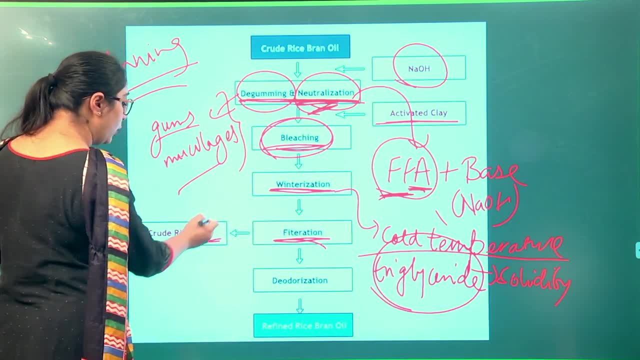 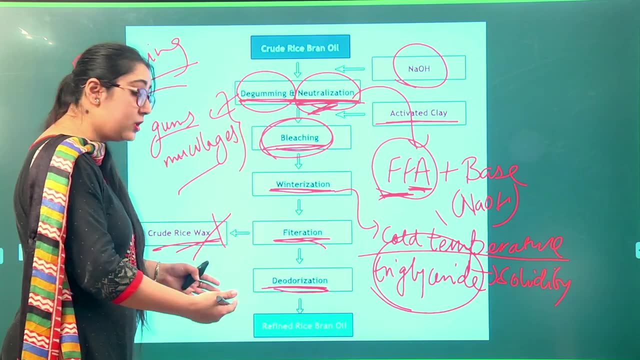 it can be filtered out, and then the crude wax oil, the triglycerides solidified, are removed, And then we have to subject it to deodorization. In deodorization we are subjecting the oil to high temperatures, We are injecting steam in it. 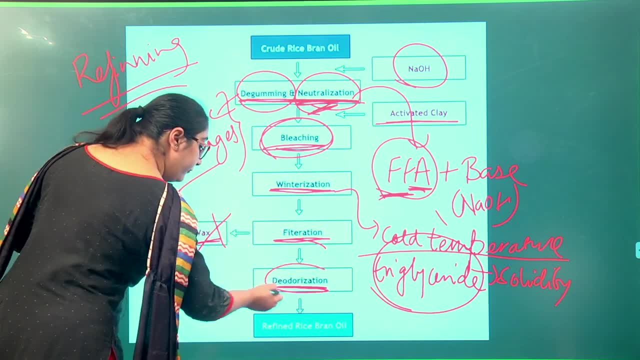 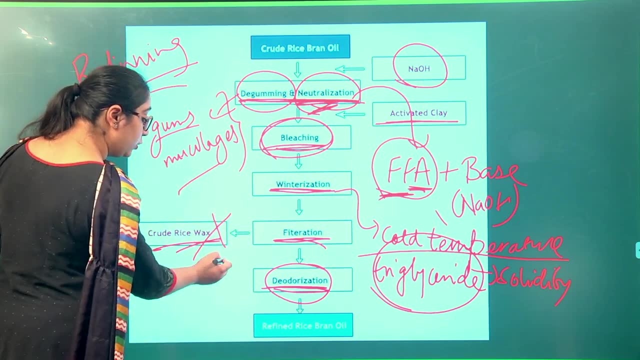 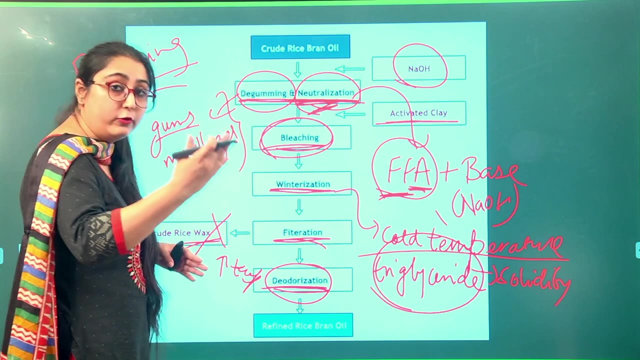 And what this will do is all the off odor is caused due to the ketones, aldehydes, all of this which are present, And once we are subjecting it to high temperature and steam, what will happen is they will get volatilized and they will be removed out of the fat or oil. 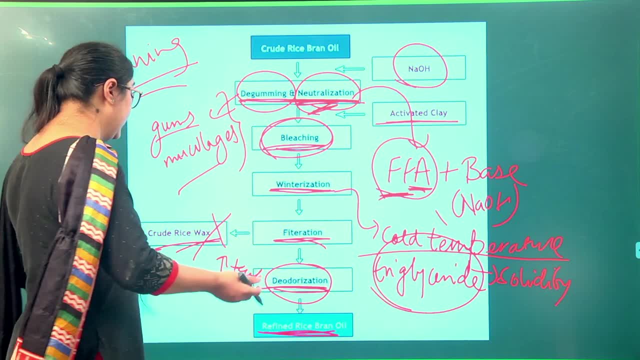 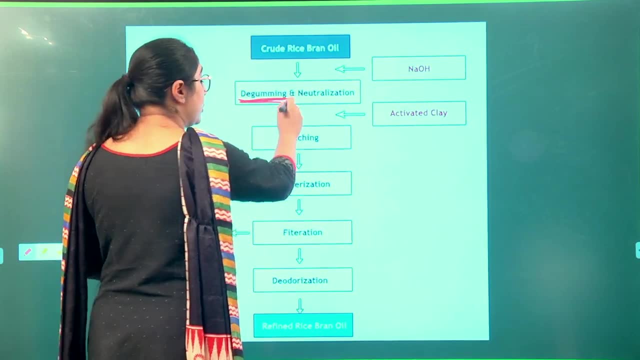 And, as a result, what we will obtain will be completely refined bran oil. So what we are basically doing during the refining process: The first step, removal of the gums or certain mucilages which can be present, So degumming and neutralization is done. 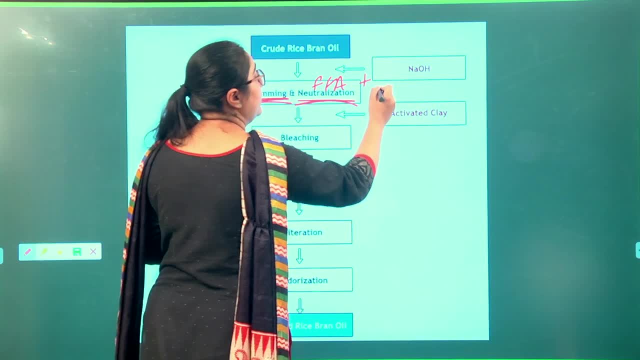 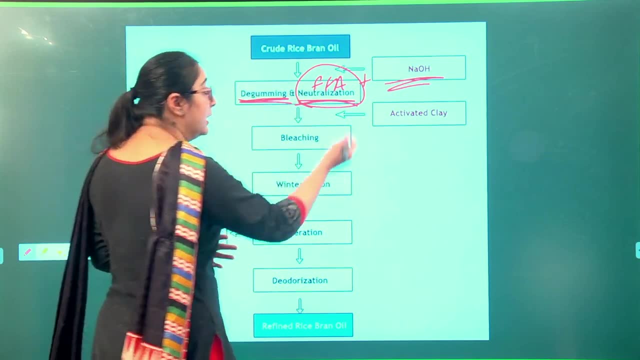 To neutralize it, that is, the removal of the free fatty acids. we are adding the NaOH to neutralize the acid. After the neutralization, the free fatty acid has been brought down. Now we have to remove the coloring substances. For that reason we are adding clay.